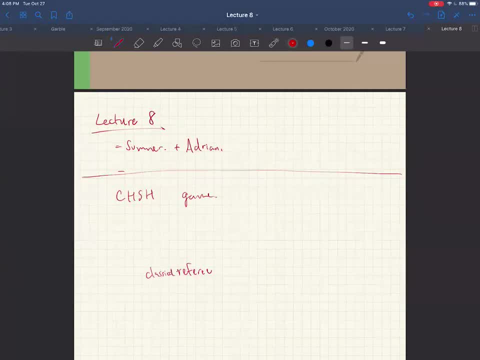 and two quantum players, Alice and Bob. right, And we assume that Alice and Bob can't communicate with each other, but instead they interact with the referee And this game, you know it has quantum games, Meaning that, using quantum entanglement, Alice and Bob can win this game with a higher probability. 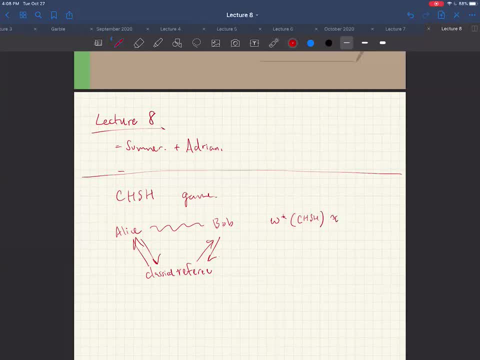 than what's allowed classically. So the quantum value of this game, which is denoted by this omega star of CHSH, is this cosine: squared pi over H value, Well, it's exactly equal to it, And this is, you know, 0.854.. 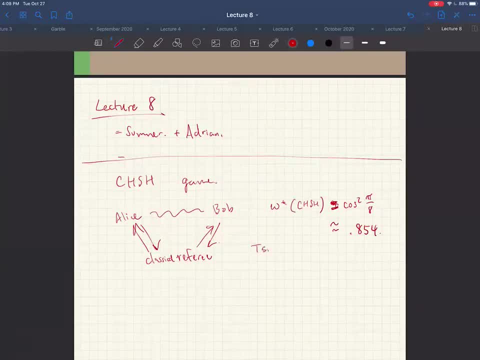 So we saw that the game is a non-local game, And we saw that the game is a non-local game. So we saw that the game is a non-local game And we saw that, based on this thing called Serilson's bound, this is the optimal quantum value, Like no quantum strategy can do better than this. 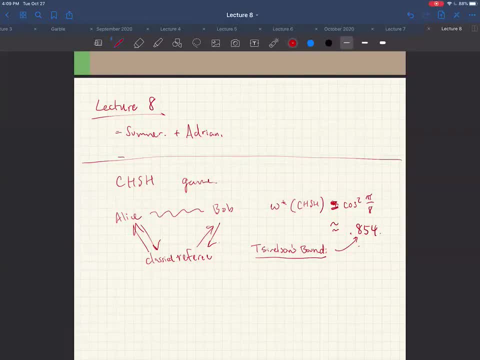 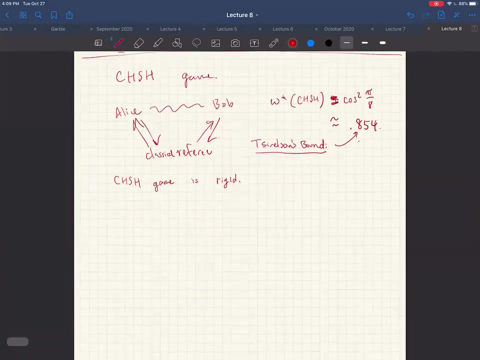 Okay, So that's what Serilson's bound proves. And we also saw that not only is this the optimal winning probability, but this game has this rigidity phenomenon. So the CHSH game is, it is rigid. So let's just remember what that means And I'll rewrite the theorem statement. 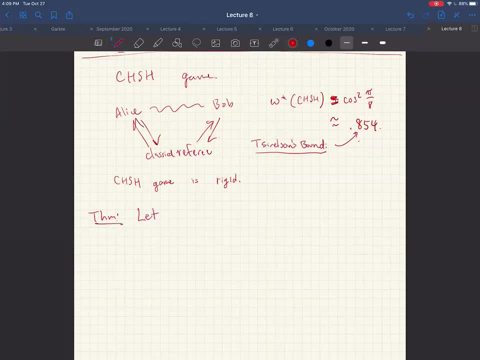 So it says that if you walk up with any quantum strategy for the CHSH game. so what's a strategy? Well, it's some quantum state that's shared between Alice and Bob, And it's a collection of measurements that they both perform when they get their particular. 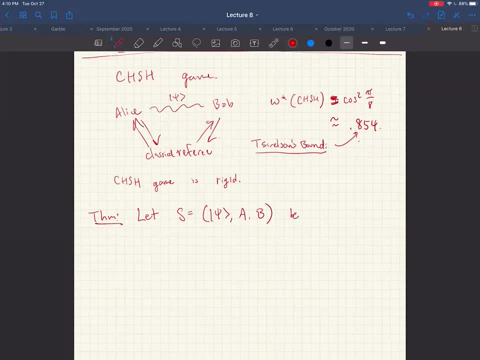 questions in the game. So let's say that this is a D-dimensional strategy in the game And all you know about this strategy- I mean this dimension D- could be arbitrary. It could be like two or a hundred or a million or anything. You just know that it achieves the. 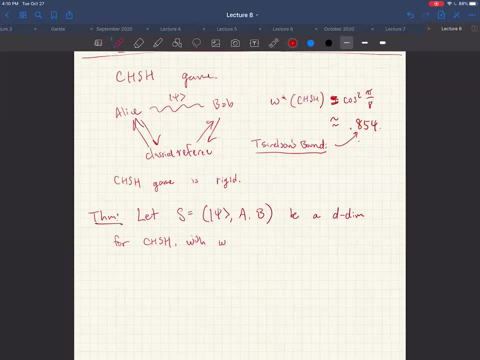 quantum value. So that actually places very strict constraints on what this strategy can look like. So the conclusion is that there exists these local changes of bases. Formally speaking, they're these isometries. So there's gonna be an isometry for Alice that maps her part of the state which we call A to. 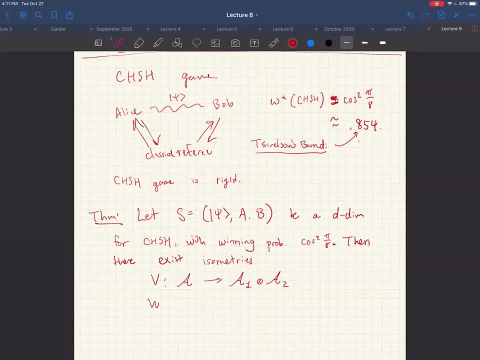 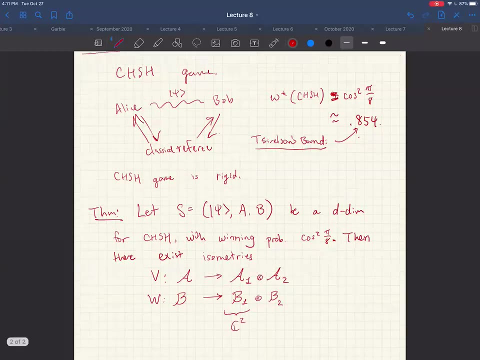 some new spaces that I'll call A1 and A2.. And there's an isometry for Bob that maps to B1 tensor B2,. both of these are two-dimensional spaces, A1 and B1, and under this basis change. 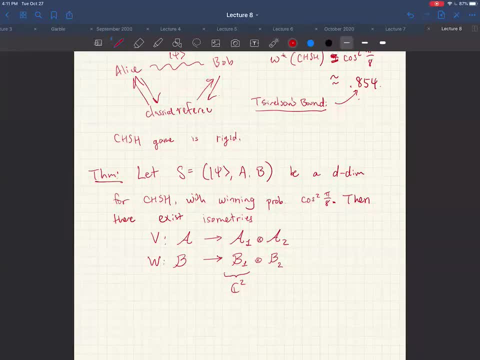 you see that this strategy S looks exactly like the textbook strategy that we know and love. So if we let theta denote applying these local change of bases to the state that they share, then the state factors into the EPR pair and some junk state. 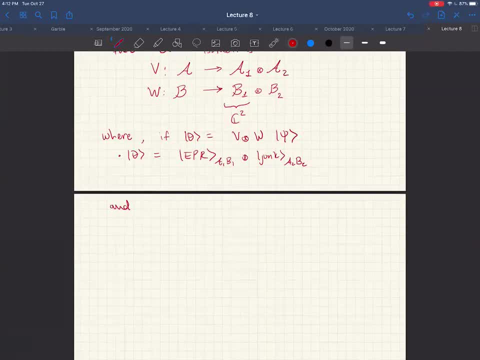 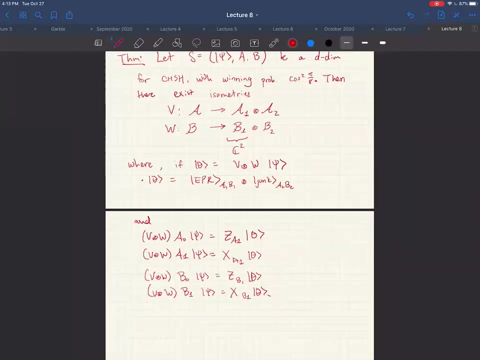 and their measurement observed in observables. look like the poly Z and X observables. So I'm just reviewing what we proved last time. Oh oops, this should be A1.. I'm sorry. Okay, and furthermore, like this, theorem can be made robust. 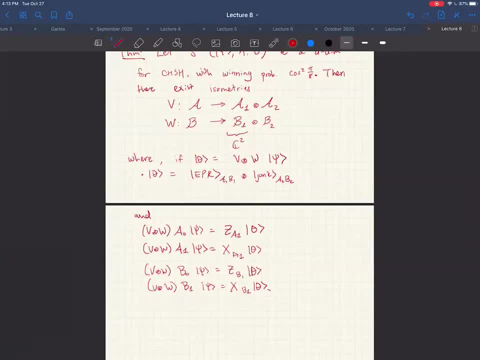 in the sense that this strategy didn't actually need to succeed with exactly the optimal success probability. If it, if they won with probability, say, you know, optimal minus epsilon, then all of these equalities will just be replaced with approximations. 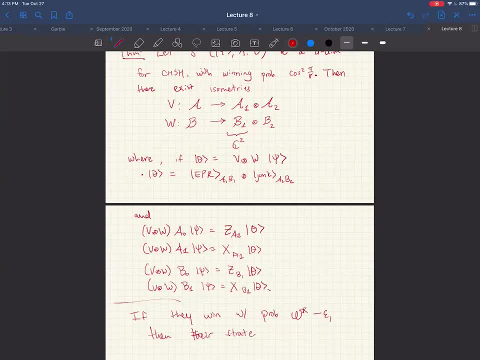 So I'm just comparing that to the textbook operation And so you can see that in terms of the asterisk, you can see the x-axis, the, Where the Z and the y-axis is the plus or minus, the z goes to z. 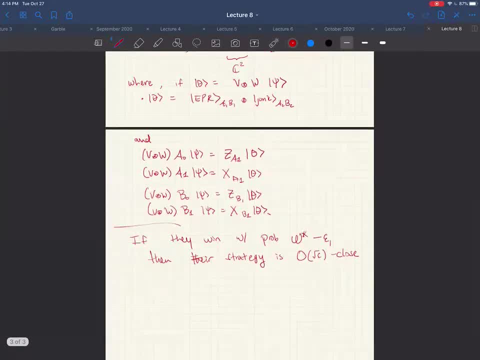 and the z goes to x And it will be the z to z. So you can see that it's all in the textbook strategy. The problem is it's different than the past, So you have to make sure you get this right. It is between the plus and minus operators. 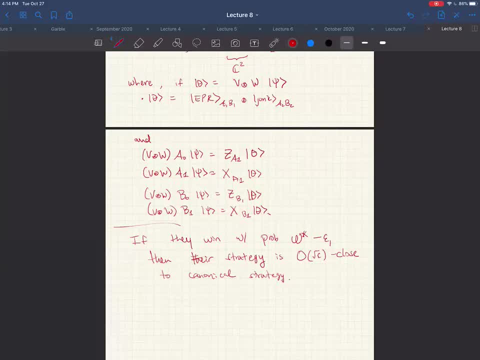 because you haven't been able to do any ever since we've done as you've been doing this all along. You need to make sure that this gives you the same Wo. you need to make sure that this gives you the same as the last. 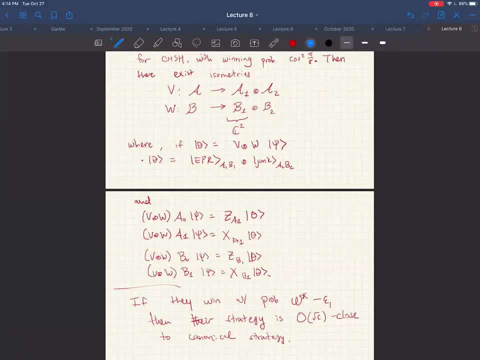 It's all in here, So you should be able. textbook strategy. So I'll just make a note here. So you know, the textbook strategy says that you know Bob should be. you know z plus x and z minus x. 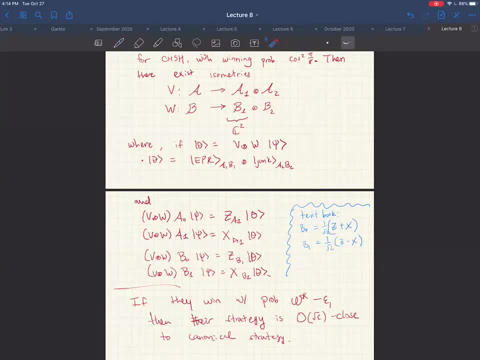 But these are actually. you can conjugate these with some another change of bases to get exactly z and x again. So in some sense, like these two matrices are the same, it's just you. so that change of basis is folded into your choice of w. 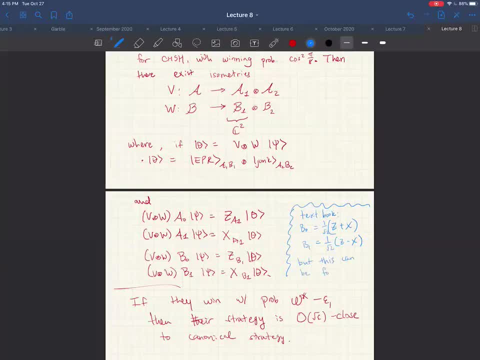 Okay, So yeah, That's a good question. So there's like two ways of thinking about what the textbook strategy is. One is the one that you saw, where they share the EPR pair, but Alice and Bob's operators look a little different. The other way is to think of it here, where Alice and Bob both apply z and x. 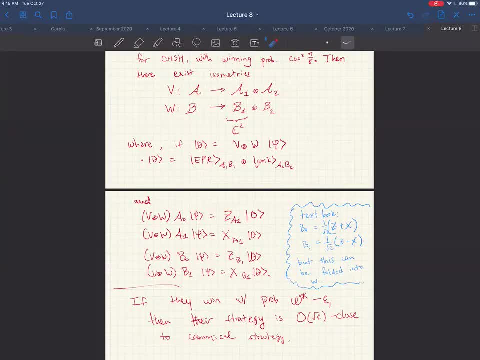 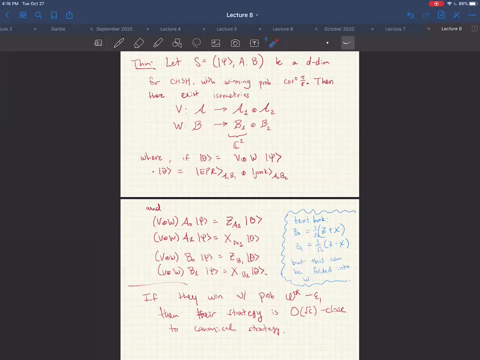 but the state that they share is kind of like a slightly twisted version of the EPR pair. It's the EPR pair where Bob's side has an additional unitary. Any questions about, like, what's the meaning of this, this statement? 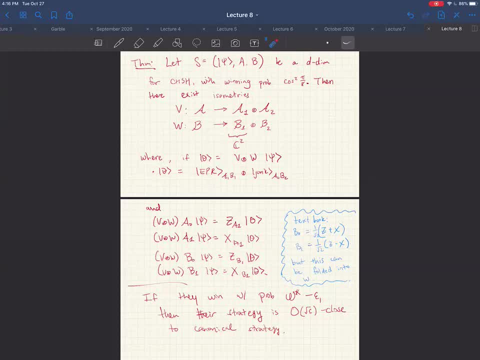 So one thing that's important to note: like: so this is kind of a mouthful right. Like this theorem statement has like a lot of parts like there's these isometries and things like that, But these like any rigidity statement. 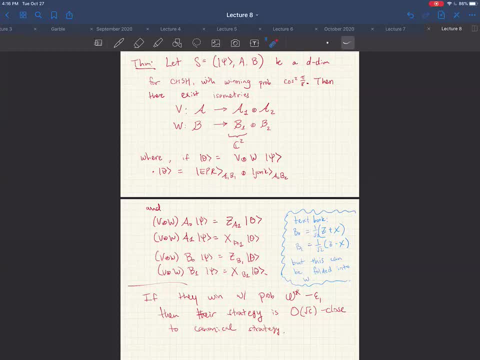 I mean okay. so what is the rigidity statement morally saying? It's saying that there's essentially just a unique quantum strategy to win optimally in this game, And it but this uniqueness has to be like there's always some wiggle room, because like 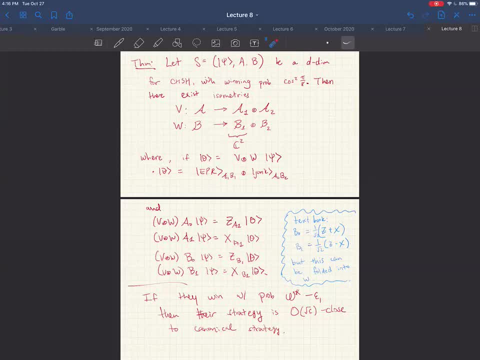 imagine that Alice and Bob took the unique, took the textbook strategy and they just applied some arbitrary change of basis locally on their own side. And I mean this clearly won't change the success probability of their strategy. I mean they're just 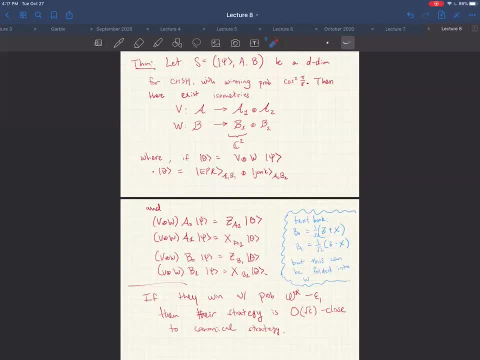 you know just kind of like changing coordinates, but you know it doesn't fundamentally affect anything. So any rigidity statement has to take that into account. But this theorem is saying that's the only thing you need to take into account. But aside from that you really just 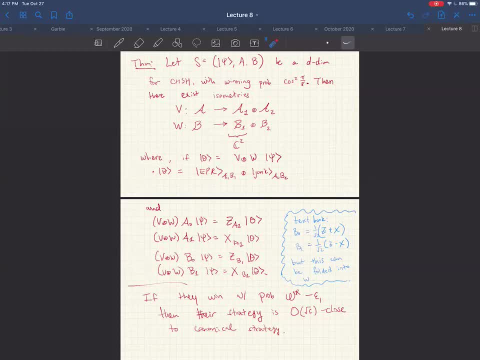 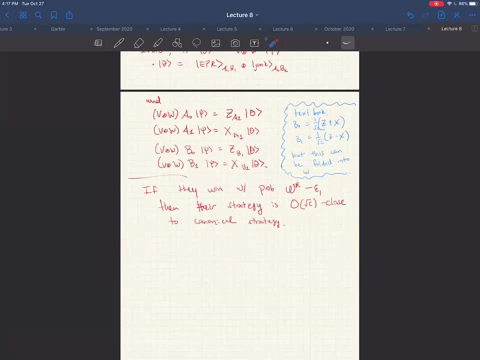 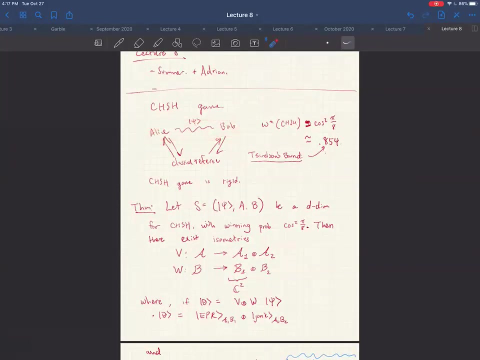 just have this. So this rigidity statement is really powerful because this is a way for this purely classical verifier to start getting like a very precise handle on what quantum operations these two players are doing, Right? So you know, you imagine that you're this classical referee and these two unknown quantum devices are out there and you're interacting with them and you have no idea what's going on inside of them. 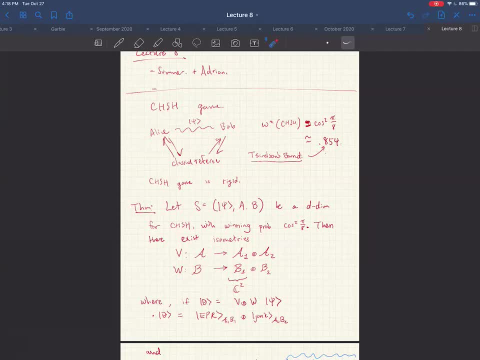 Like they can be arbitrarily complicated. but by playing the CHSH game And if you see that they're winning with this optimal probability or close to it, then you actually have, like you know, structurally inside those devices, Essentially what's going on, Like they have no other choice. 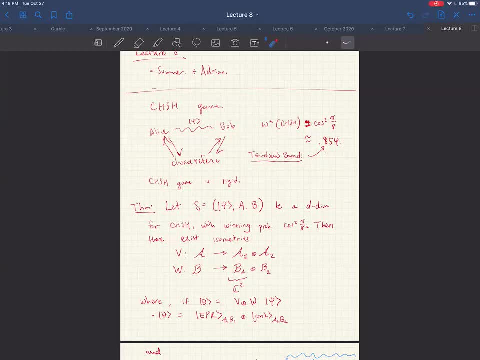 And so we're going to use this idea, this rigidity phenomenon, not just to force Alice and Bob to share a specific quantum state and perform specific quantum measurements, but we can actually force them to perform our favorite quantum computations, And in that way we can actually 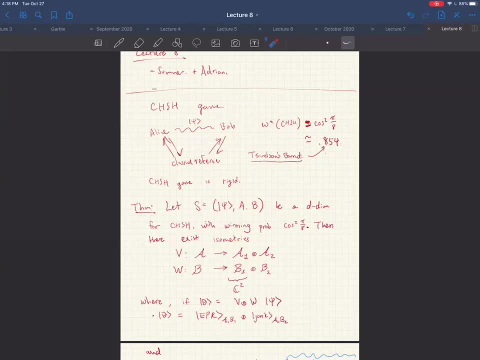 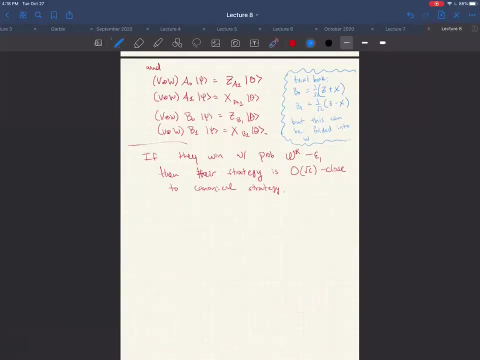 Classically verify quantum computations. But before we get there, actually, I have to just describe a couple other non-local games other than the CHSH game that will have properties that will be slightly easier for us to use. So let's discuss those. 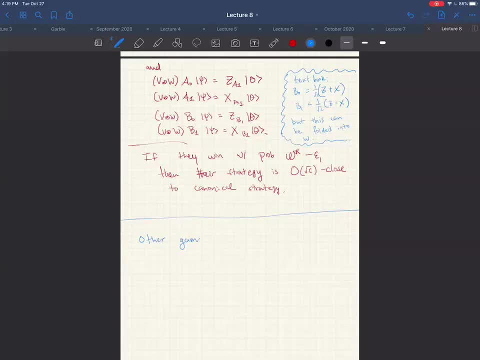 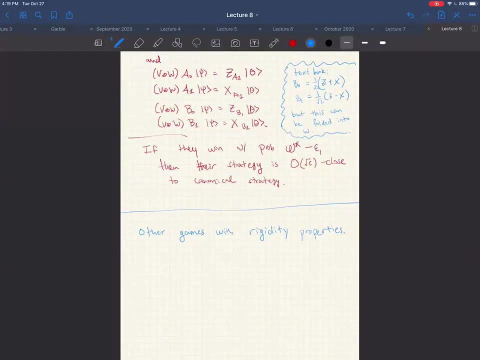 Okay. so one downside of the CHSH game is that the optimal quantum success probability it's it's not 100%. you know it's this like 0.85, 0.4 value. So you know that's kind of a good idea. 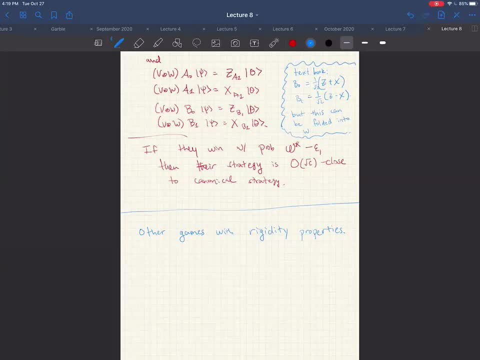 But it's kind of annoying. It's not as nice, You know. so, for example, like: imagine that you're this classical referee and you know you're interacting with these two devices. How do you know that they're winning with a probability that's exactly cosine squared pi over eight. 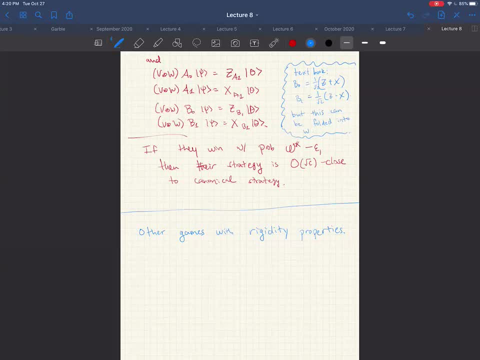 I mean, it's not possible, right? You know, the only thing you can do is just play this game repeatedly with the devices and just try to get some empirical estimate of how often they're winning. So you're just going to get some approximation of their winning probability. 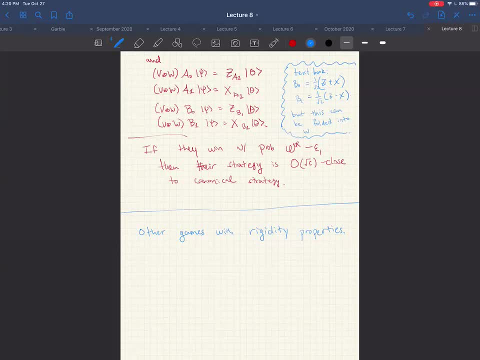 So, you know, so that's, that's one thing. So it'll be nicer to have a rigid game that actually has a quantum success probability of 100% right, where they can win 100% of the time. So so this, you know, this motivates the something called the magic square game. 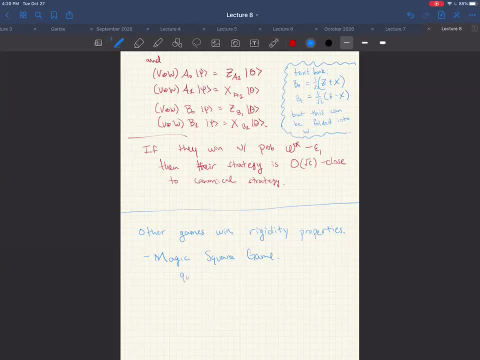 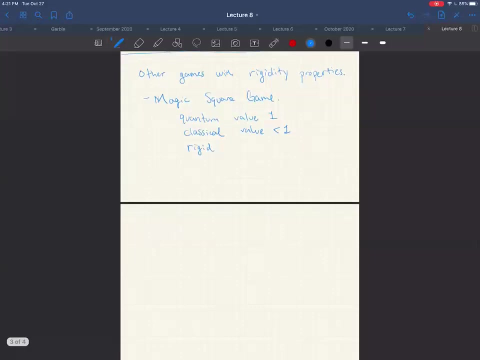 So this is going to be a game that Has quantum value one And the classical value is going to be strictly less than one, And it's going to be A rigid game, like there's again essentially only a unique optimal quantum strategy. So so this game is a slightly more involved in the CHSH game. So how does that work? 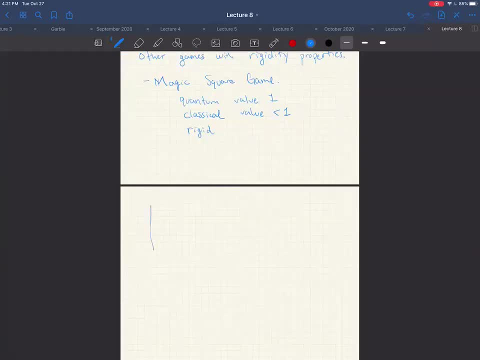 It's based on the following setup. So let's imagine that we have a three by three grid And The goal is you want to populate each of these squares with zeros or ones That satisfy two constraints. So one is that all rows have to have even parity. 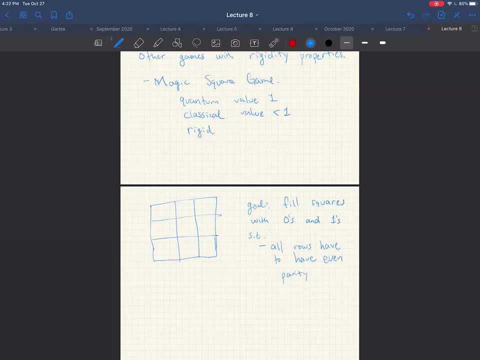 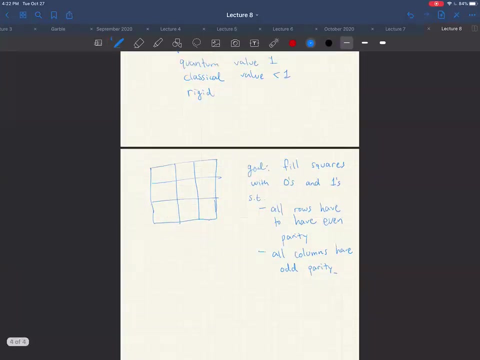 like meaning: if you sum up the ones and zeros, you get an even number, Whereas in all the columns, if you sum up the zeros and ones, you get odd parity. So is this possible? Nope, And why not Cause count the parity of the sum of all the boxes. 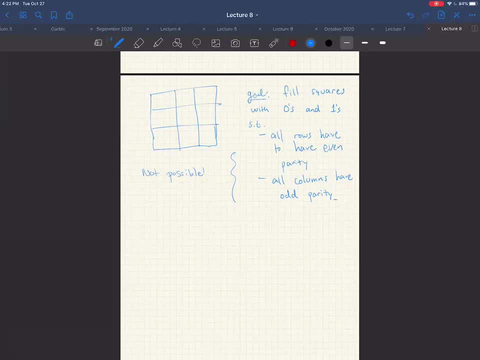 If you count it via the rows, you have that each box has, or each row has even parity. So in total, the entire nine boxes have even parity, Whereas if you count it with the columns, each column is odd parity. So the nine boxes have odd parity. 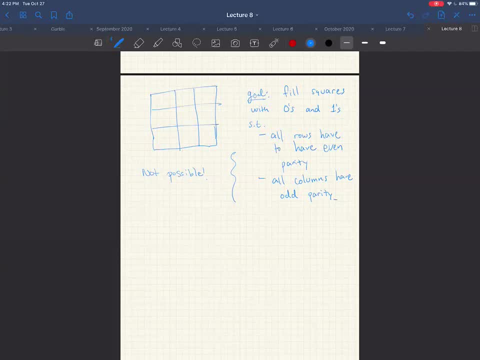 Exactly So. there's no way to fill out these squares that satisfy all these constraints. You're always going to get at least one of the squares like, or you're always going to violate at least one of the constraints, So okay, so that's. you know. that's pretty straightforward. 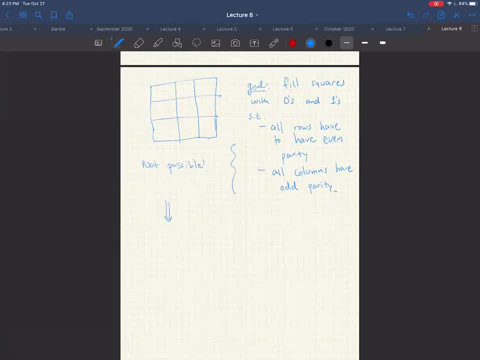 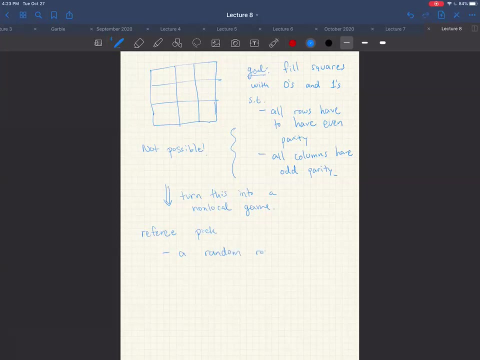 So let's turn this into a non-local game, And the way this game works is that the referee is going to pick a random row or column. So there's six choices, right? There's three rows or three columns. Just pick a random row, column, call it X. 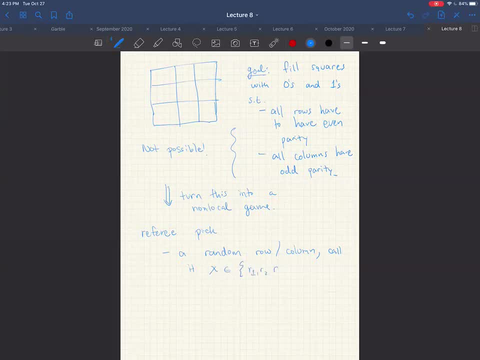 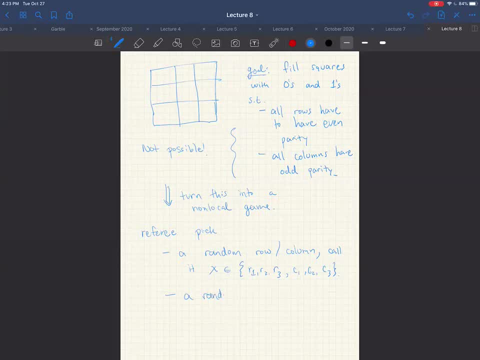 And then it also picks a random cell within that row or column, right? So there's, there's nine cells, right? We can label them 1, 2, 3,, 4,, 5,, 6,, 7,, 8,, 9.. 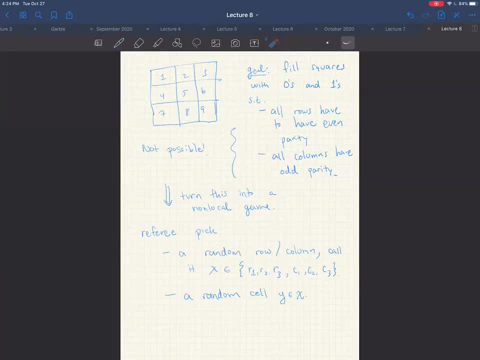 So you know, for the example, the referee could randomly choose to pick column C3. So this middle column, and then it will pick a random cell, maybe cell number eight. So the referee will pick these things and then the referee sends X to Alice and then Y to Bob. 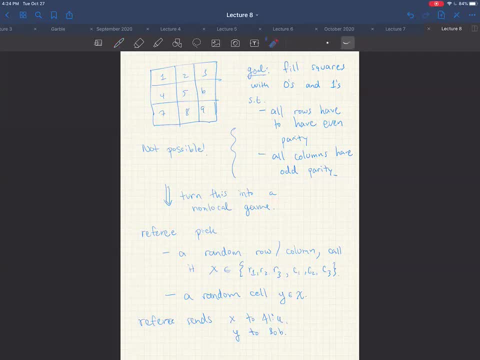 So the important thing is, when Alice gets her- let's say she gets a column- she has no idea what which of the three cells Bob received. and on the other hand, when Bob sees his cell, he doesn't know whether it was the row or a column. 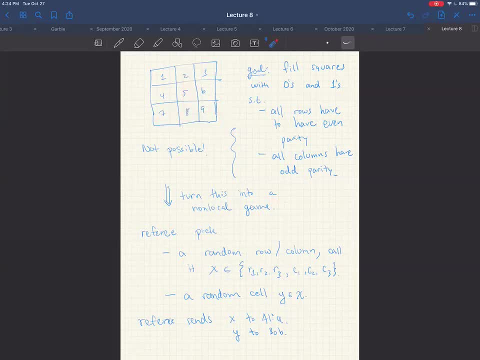 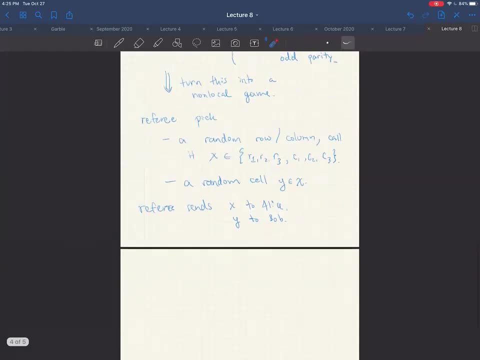 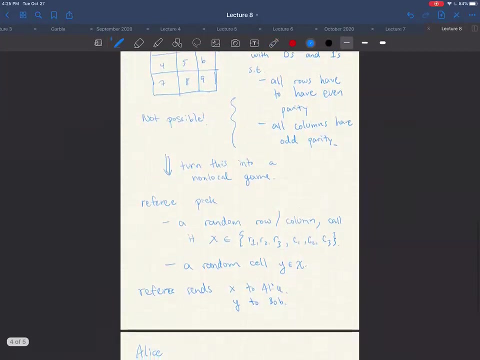 that intersected that cell, which one that Alice got. Okay, So so it. you know they have incomplete information about the questions. So what are they supposed to respond with? Alice is supposed to just give an assignment of the three cells in her row or column. 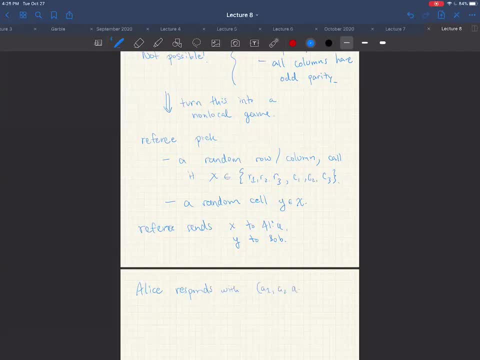 And then Bob responds with just a single bit That's supposed to be an assignment to the cell that he received. And then Bob and then Alice gives the same assignment as the two-cell that he received. Okay, So Alice is supposed to write. 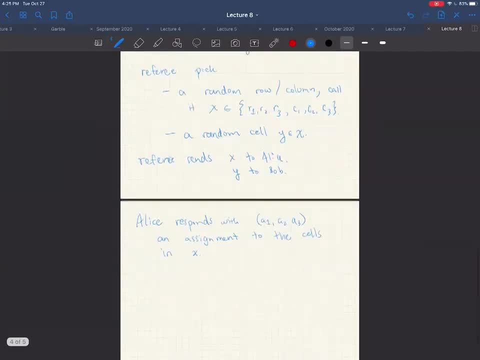 a set of three things and send it to Bob. So you're going to get four parts, Okay, So the other thing that all of these steps are going to be was kind of a set of numbers, And so the easiest way of getting an assignment of those numbers is to answer. 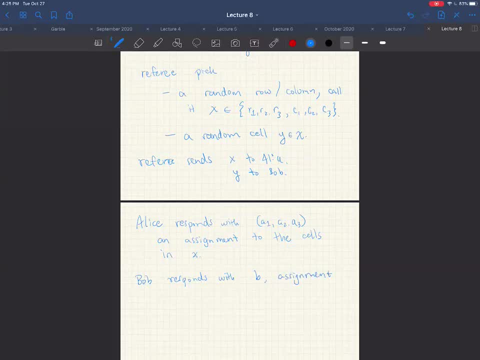 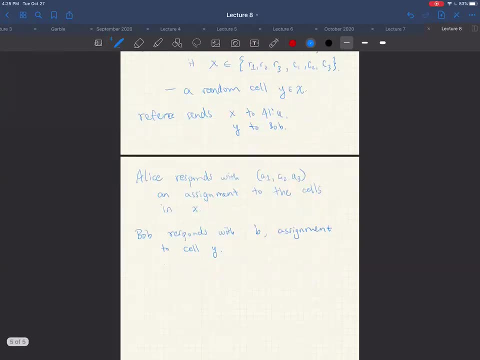 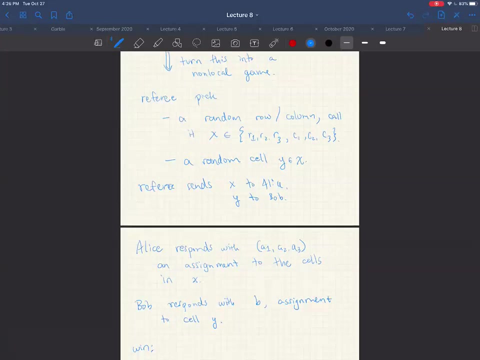 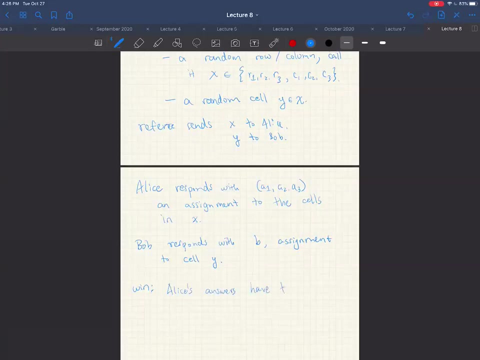 Okay, So this is like the questions and answers they get. How do they win? Well, they win. if well, Alice has to respond with an assignment to like a row or column, So her answers have to satisfy the parity constraint Right Corresponding to whether she got a row or column, And Bob's answer for the cell. 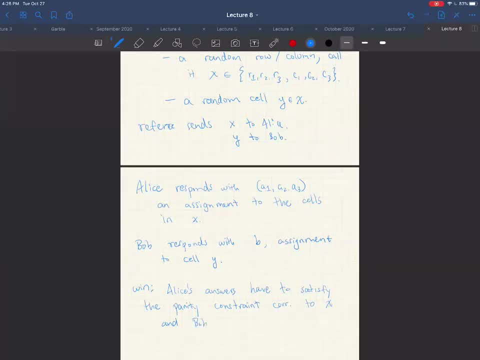 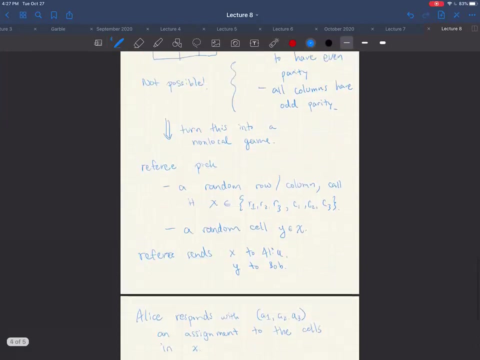 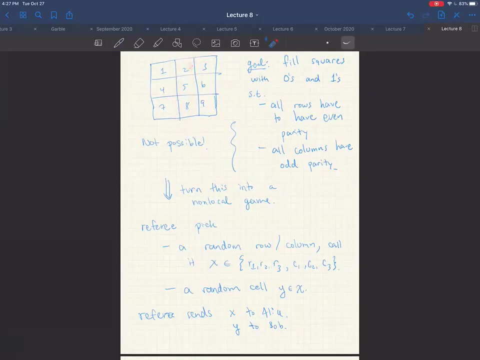 has to match what Alice received, Right, Corresponding to whether she got a row or column, And Bob's answer for the cell has to match what Alice received. So this is the winning condition. Does that make sense to everyone? All right, so Alice is. let's say again: take this middle column, Alice is going to give. 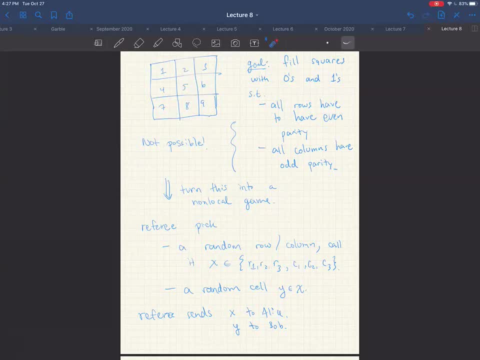 bits for box 2,, 5, and 8.. Bob is going to only answer for box 8, and they just have to match on that bit, And furthermore, Alice's. the parity of her answers has to be, in this case, odd. 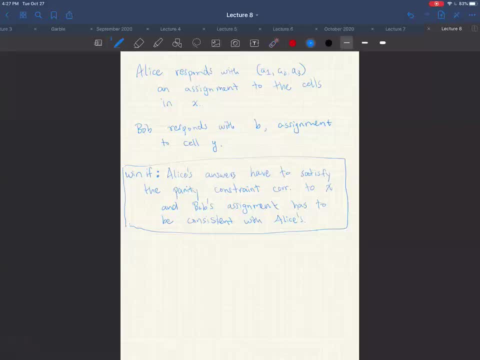 I have a very basic question: What is the parity on a row or the parity on the column? If you have the bits specified on a particular row, when you say it has a parity of x, what exactly do you mean by that? Oh, 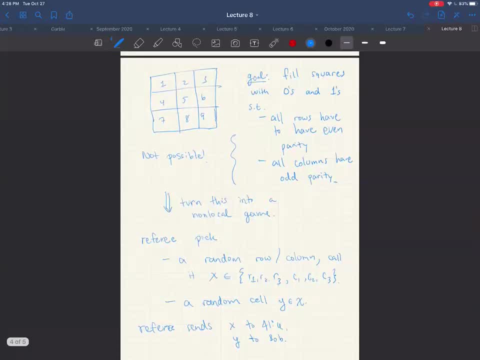 so I mean x refers to whether which row or column she got. So let's again. if x was say the first row, then she gives it three bits right: a1,, a2,, a3, and then the parity of those. 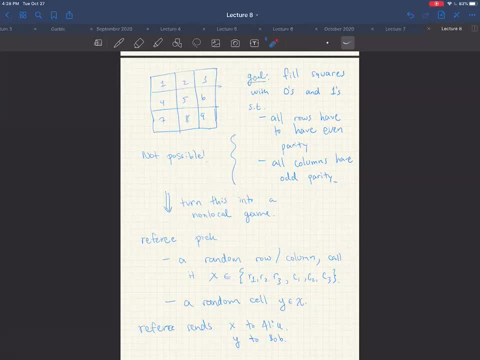 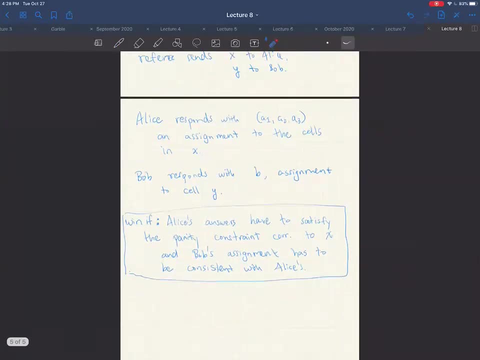 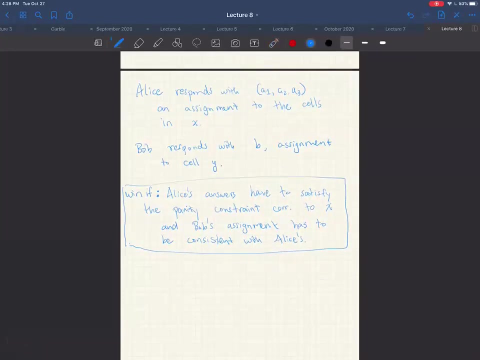 bits. if you sum up those bits, it has to be an even number, Whereas if you sum along a column, it has to be an odd number. That's what I want to know, Thank you, Thanks. Okay, So so you know this is the Magic Square game As a non-local game. 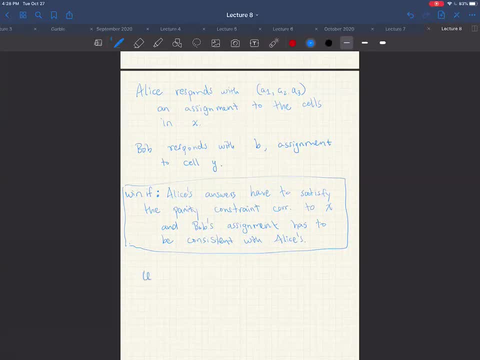 I'm just going to abbreviate it as ms. And the classical value of this game. it's going to be strictly less than one, as I mentioned. In fact, it's only going to be 17 over 18.. I mean, basically, the way to see that it cannot be one is that if it were one, 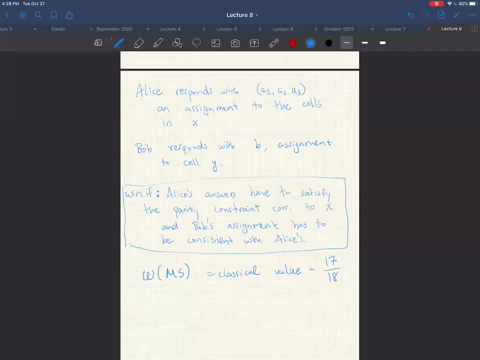 it would actually imply that they could consistently fill out all of the squares such that it satisfies all of the constraints, But we know that's not possible, So it has to be less than one, And in fact they can win 17 out of 18 times, So that's not too hard to show. 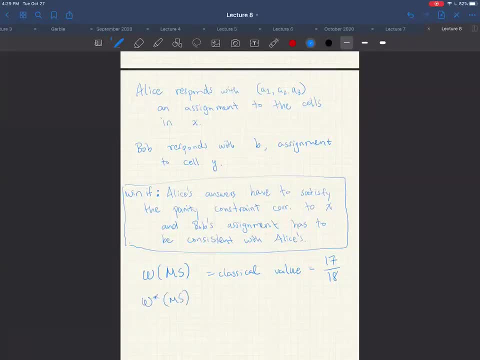 But the quantum value is actually one. There's a, there's a quantum strategy where they can always win, which is kind of strange because you know, like an, you know an undiscerning external value, right Yeah? 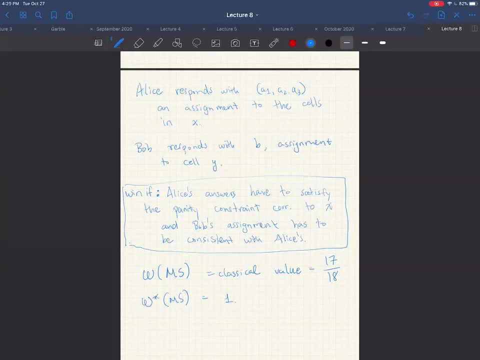 So an undiscerning external observer watching them play this game would be like: well, how are they doing this? It would seem like they had a way to fill all of these squares in this consistent way, which is impossible, But they're just making use of quantum entanglement. 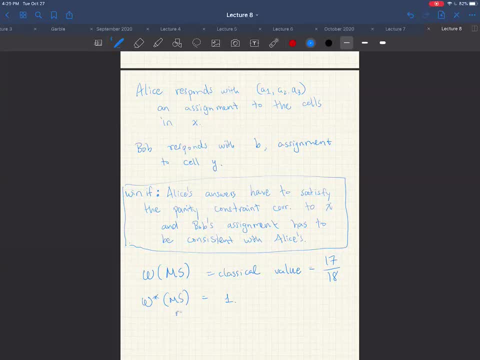 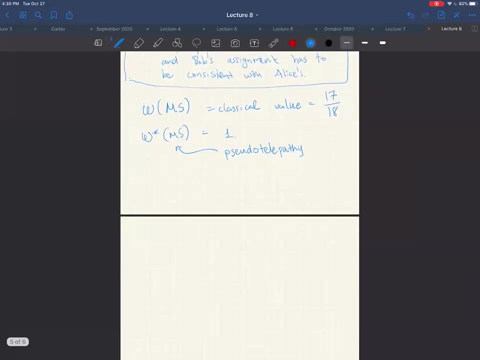 to do this. So for this reason, since it has quantum value one, this is off. the Magic Square game is often called a pseudo telepathy game. So So that's an interesting feature of the Magic Square game. So what does? 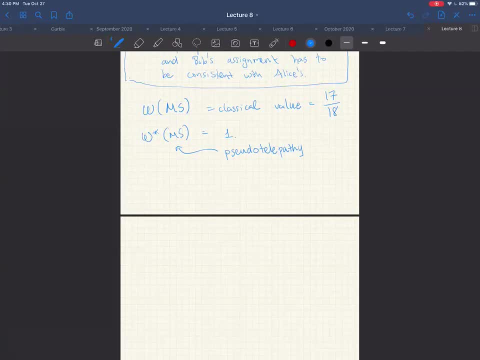 the quantum strategy look like It involves two EPR pairs. Okay, so there's a total of four qubits And and two goes to Alice and two goes to Bob, And the measurements they make are also going to be poly measurements. 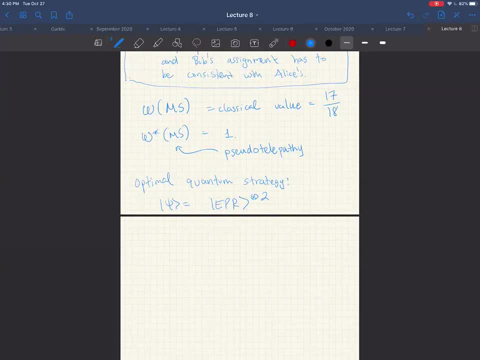 And they're gonna follow this following table of observables and we're gonna draw them on this three by three grid, So I'll just write them out, Okay, so each of these letters like I, X, Y and Z denote the standard like poly observables, right? 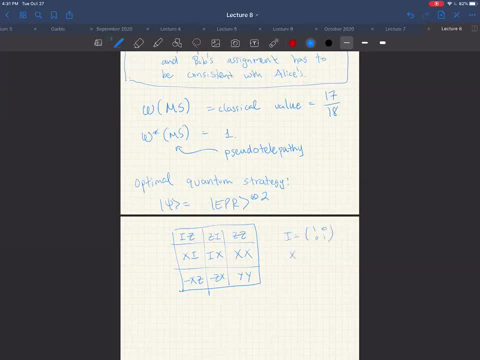 So I is identity. matrix X is this bit flip. matrix Y is this thing, And really there's an implicit tensor product in between these two, but we just don't write them. So all of these are observables. they're two qubit observables. 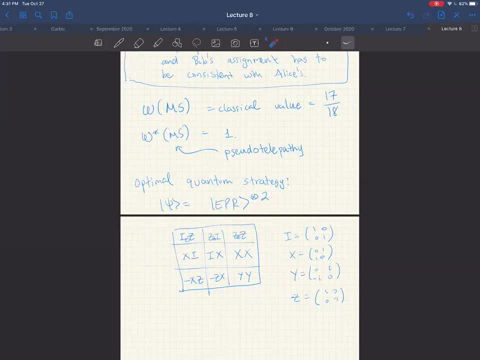 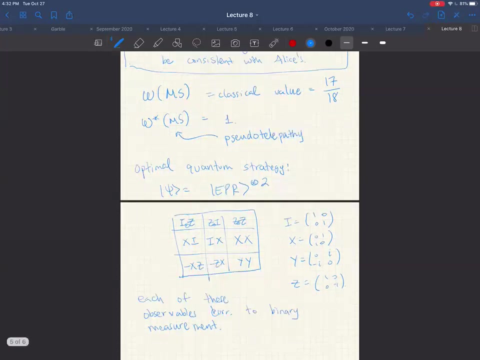 So, like if you're given two qubits, you can measure the both of them using one of these observables, And each of these observables gives a one bit answer out. So the strategy that they'll use to win with probability one is going to be as follows: 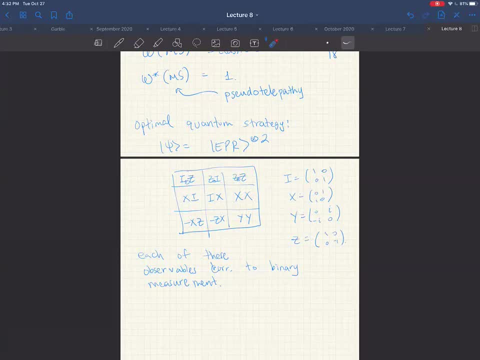 So when Alice gets her random row or column- let's say she gets the middle column- she has two qubits, So she's gonna measure her two qubits using these three observables in sequence. Okay, So she's gonna measure using ZI. 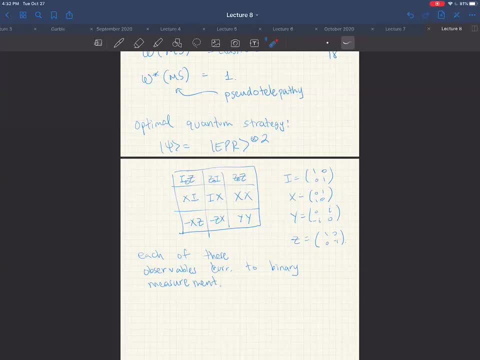 So she's gonna get a bit. she calls that A1.. Then she's going to measure the same two qubits using this observable IX. She's gonna get another bit, A2.. And then, finally, she's gonna measure with minus ZX and to get her final bit, A3.. 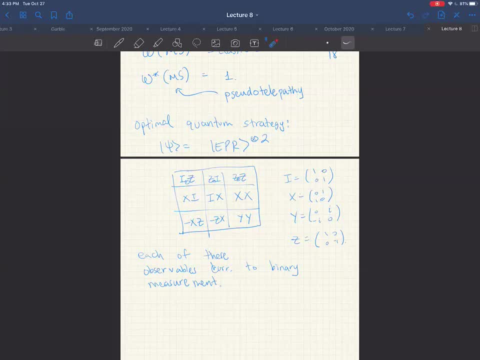 I understood from the description of the game before that Alice doesn't know whether she got a row or column, or which row or which column. Is that not the case? Oh, she knows whether she got which row and which column, she was told. What she doesn't know is the particular cell. 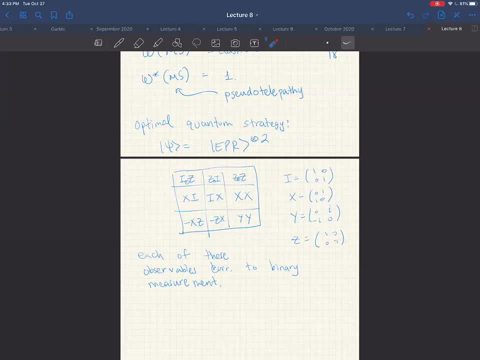 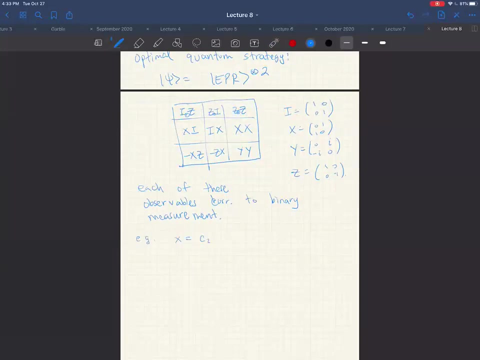 that Bob received. Okay, thanks. So let's say, like her question, X is. so let me write this out. Let's say, for example: let's say that X is equal to C2 and Y is equal to cell number eight. 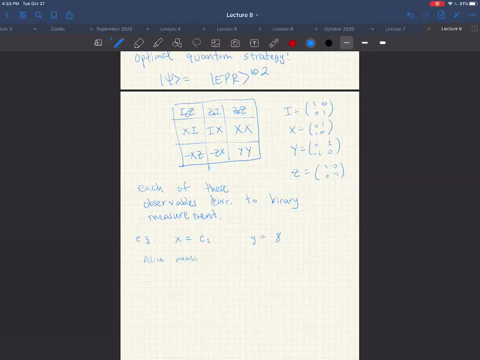 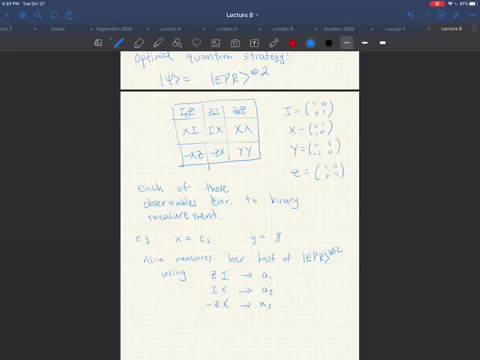 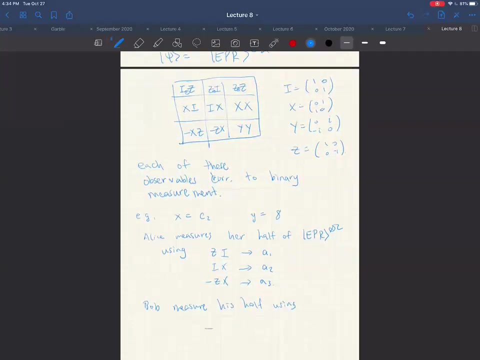 And each of these yield bits A1, A2, A3.. And each of these yield bits A1, A2, A3.. Bob will just measure his half using minus ZX and he'll get a bit B. So So one thing that is important to know. it's: like: what does it mean to measure? like, how is it possible to measure these three observables in sequence? I mean, you can always do that, But in fact the order in which she measures does not matter. 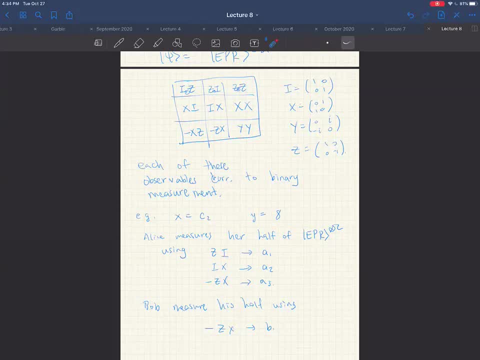 This is not generally the case in quantum mechanics, but these observables have a very special relationship, which is that in any given row or column, these observables commute with each other, And the fact that they commute implies that Alice can actually simultaneously measure all of them. or, put another way, she can measure them in any particular order, it doesn't matter. 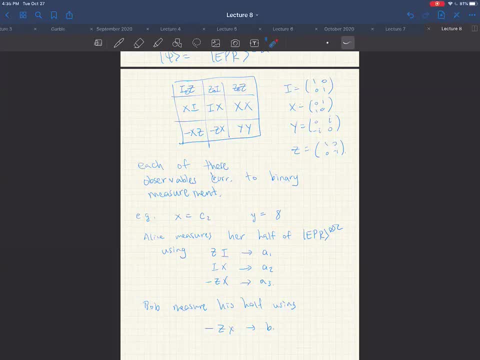 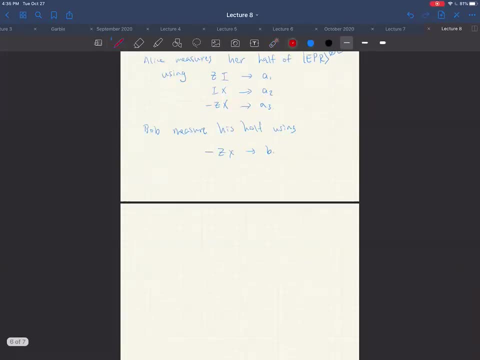 She's always going to get sort of the same distribution of outcomes. So important point, Okay, Okay. so I think that's a pretty good one. Any other questions? any other questions, please? Okay, Thank you, Thank you all right, um, so we're not going to work through the details here, but, um, this strategy actually. 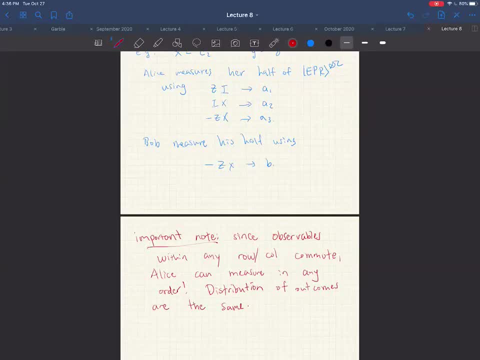 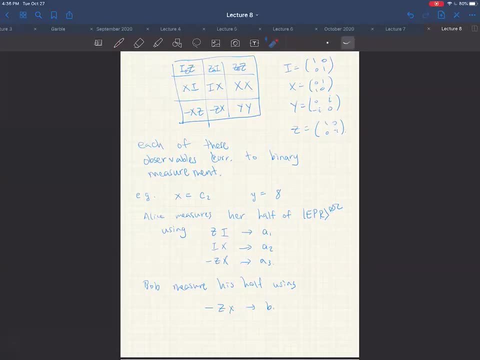 allows them to win with um, probability one, uh, and to get some intuition for why that's the case. well, you know what are the, the, the rules for winning? uh, well, first of all, alice's answer has to be consistent with bob's. um, but notice that they're always going to measure for the cell in which they. 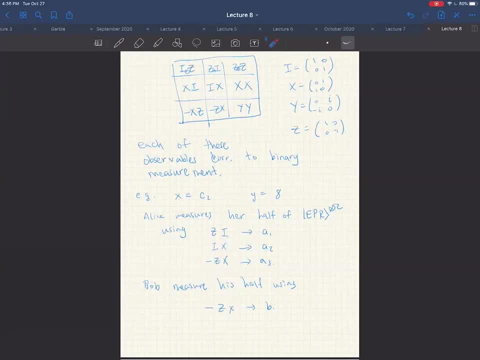 overlap, they're always going to measure the same operator, right. so, like in this case, alice and bob measure minus zx on their two qubits and since they share an epr pair, um, they're always going to return the same outcome for that particular square. so that's always going to you know that. 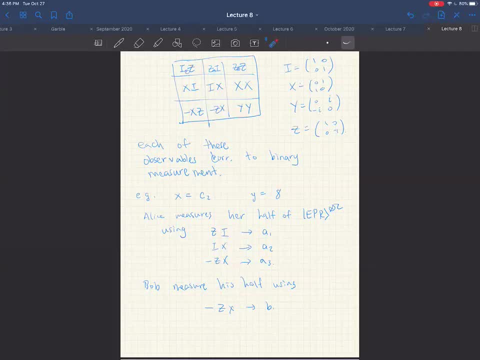 that part's always going to pass. now the other part of the winning condition is that, you know, alice's three bits have to satisfy the the parity constraint. and the reason that this is always satisfied is because another relationship that these observables satisfy is that if you look in any column, if you multiply the 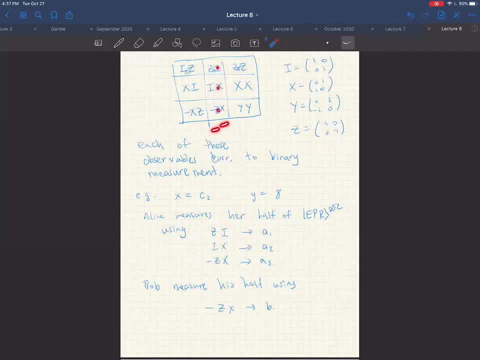 the observables together, you actually get minus identity. so let me write that here. well, they don't share an epr pair. if alice first of all measured zi ix and then only measured minus zx, right, because the first two measurements changed the shared state. but if you use the fact that, like, the order of measurements doesn't matter, we can assume that 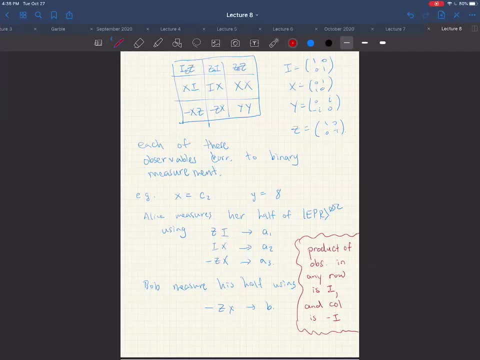 the minus zx is the same as the zi ix, and then only measured minus zx. right, because the first two measurements, zx one, happened first. yes, exactly, okay. um, you raise a really good point like: um you know, because you might think, well, if you're not careful about the order in which you're measuring, um. 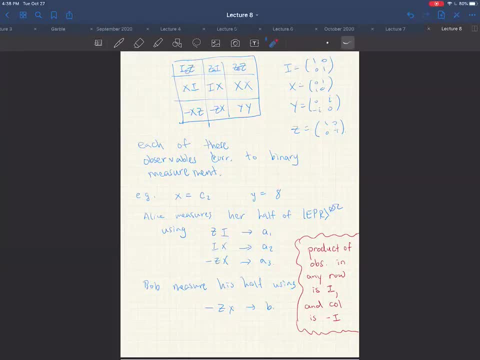 when you measure something, the state changes and you know it'll no longer be the epr pair. that's correct. um, but um. you know, the fact that you can change the order uh in any way means you can always uh without loss of generality. you can always change the order in any way and you can. 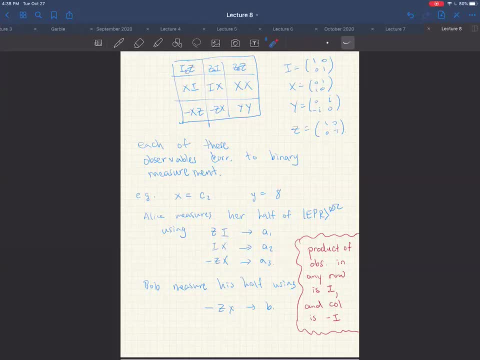 always assume that alice and bob are measuring the, the shared square at this at the same time, or they measure it first, um, and the outcomes will always be the same. another way to see it is that even if you say, well, but i want to stick with this order, you know. 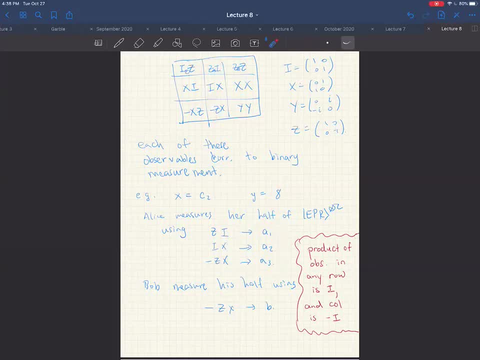 from top to bottom. and why does it mean that alice and bob have the same answer? um, well, it's because, let's, when, um, when you say that when you make, um, all your measures, uh, when alice measures this first observable, it's going to partially collapse the epr pairs into some other state. it'll still be. 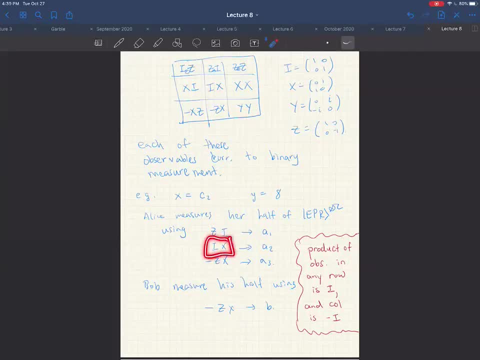 partially entangled, um so so that's why there's still some interesting correlations that occur when you measure eighths, if you go back four or five timesية. verl is that I measure with the observable, which is Z times I. I mean that the first qubit is being measured using Z. 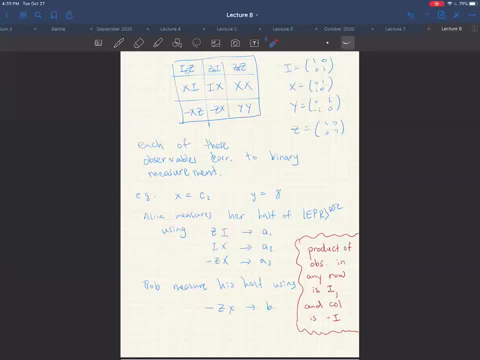 and the second qubit is being measured using I. Oh no, the first thing that you said, the observable that's being measured is Z, tensor I. Oh yeah, that's what I meant. So, like, the first qubit is measured using Z. 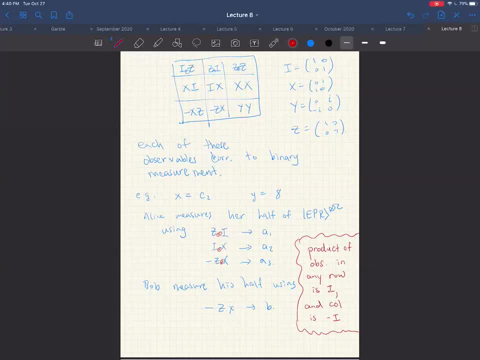 the second one is measured using I. Oh no, that would be a different-. Is the way that I'm phrasing it bad? So if you do it that way, then you're going to get two bits as output, right, Because you measure one qubit. 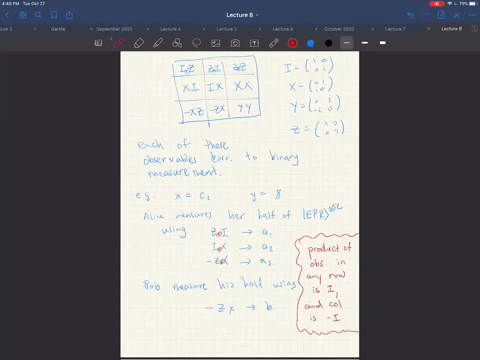 and then you measure the second qubit, then you'll have two outcomes. That would actually be- Okay, so okay, I see Like okay, so I phrased it the wrong way. but yes, Oh, okay, sure thanks. 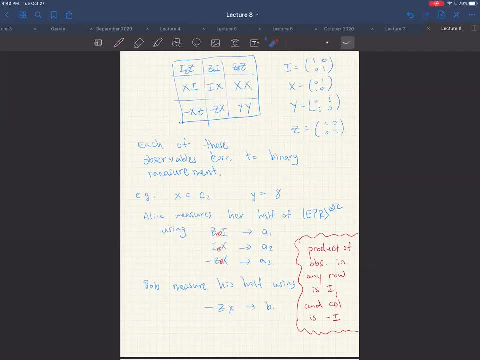 Okay, so maybe, yeah, that might've been confusing. So this looks like a two qubit measurement, right, But you should think of it, since what I'm not saying is measure the first qubit using Z and then ignore this, measure the second qubit using I. 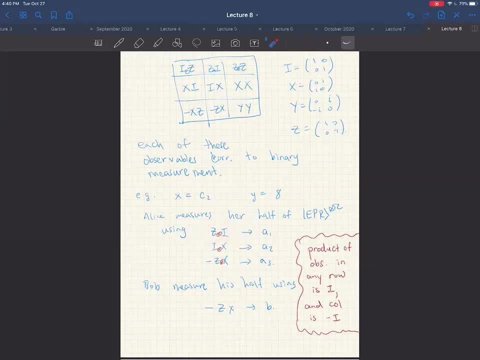 That's not what this means. This thing as an observable is like it's kind of like an entangling measurement, So this will actually entangle the Alice's two qubits together in some way And it returns a single bit as outcome. 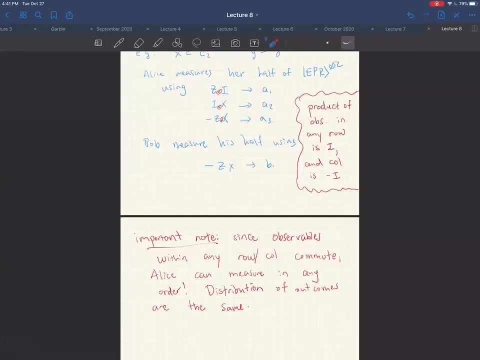 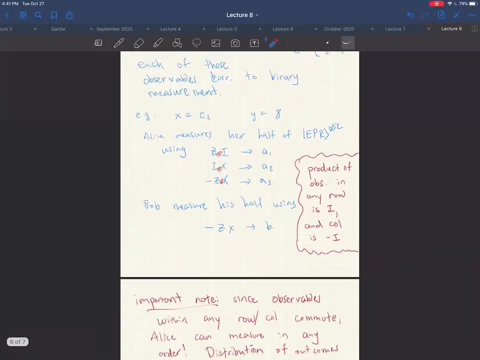 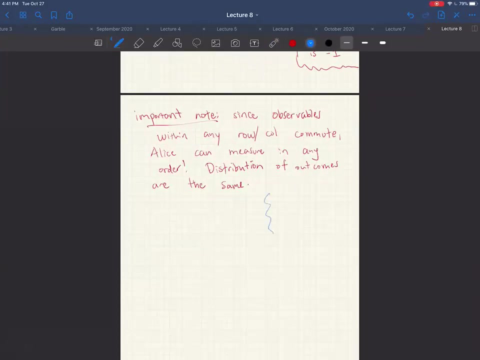 So that means Alice has two qubits and Bob has two qubits. So there are two EPR pairs in play. Yeah, that's the state that they share. So let me just draw a picture. Let me get it to the side. 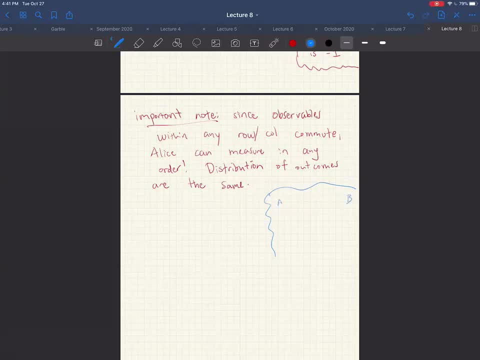 You should imagine that you know, here's Alice, here's Bob, and they share two EPR pairs, Right, this is the first one, This is the second one, And Alice will do a measurement on these two qubits. And Alice will do a measurement on these two qubits. Just to follow up on Yuval's question, I'm not quite sure I'm seeing the difference between measuring the two qubits separately. To me like how you would implement this experimentally: you would be measuring the two qubits separately and you would just multiply their results. 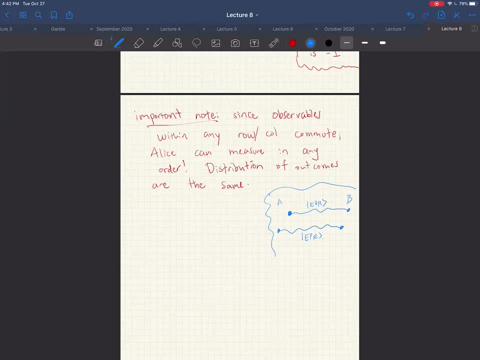 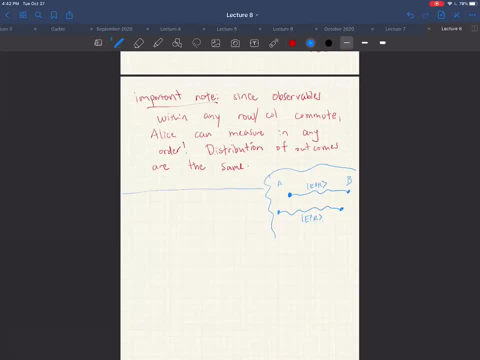 Let me choose. what's one way to do this. So let's look at the observable z times z. So let's take a quick look at the observable z. OK, So this is a binary observable. So this is equal to a projector: pi0 minus pi1.. 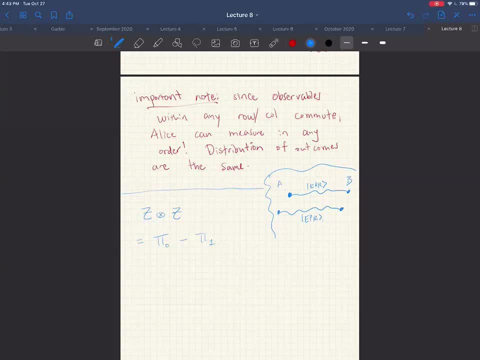 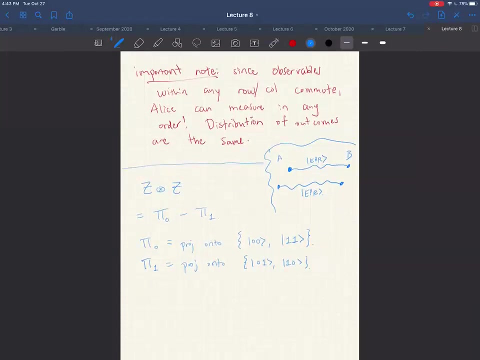 Right, And the binary measurement that you're performing on these two qubits is like this projective measurement: pi0, pi1.. But what is pi0? it's actually going to beat the projector on to Right, Right, 0, 0 or 1, 1, and pi 1 is going to be the projection onto 0, 1, 1, 0. so so let's say I took an EPR pair. 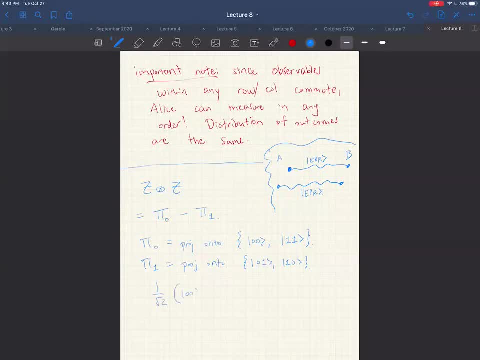 and I decided to measure both of these qubits using the ZZ observable, the. then the point is that this state is invariant under this projector. it doesn't change. so when you perform the ZZ measurement on the EPR pair, it actually doesn't change the state at all. 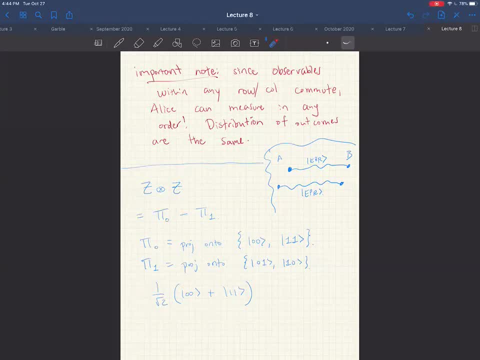 on the other hand, if you measured each qubit separately, then it would actually change the state of the EPR pair. it would actually collapse the state and you would get either 0, 0 or 1, 1. okay, so I hear what you're saying and I know we're not in like experimental physics, but I 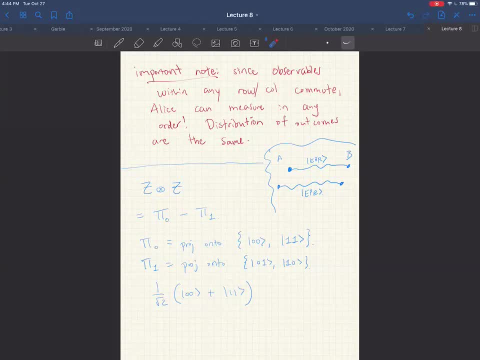 have no idea how you actually do such a measurement. oh okay, um good. so how do you actually implement this two qubit measurement? well, you first have to apply basically a, a quantum circuit, and then you, you measure, and then you measure a quantum circuit, and then you, you measure. 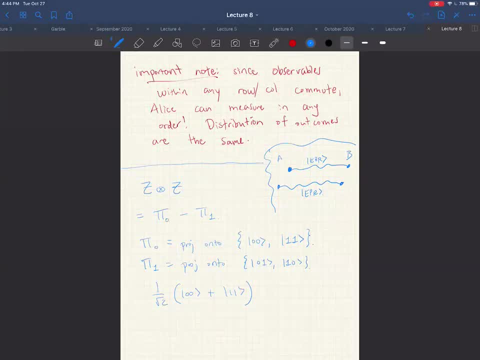 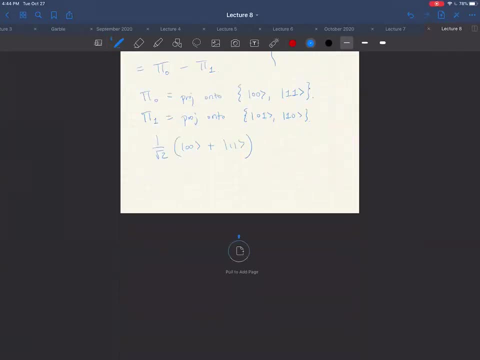 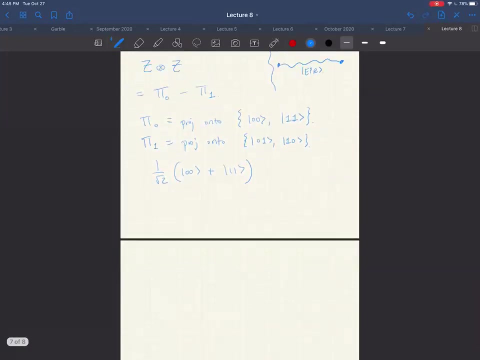 and then you, you like, you know you, you can just measure one qubit for the outcome. so, um, so, how like, okay, so this is a good question: how like, how would you actually implement this um the ZZ measurement as a quantum circuit? so I think the easiest way to do it is you. 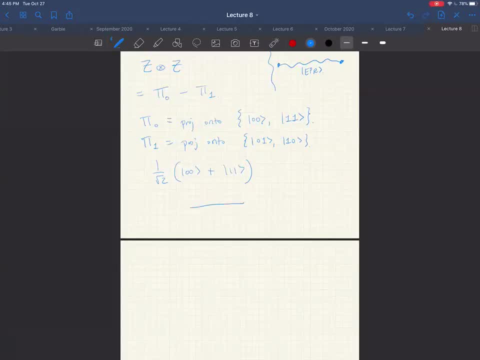 introduce an ancilla. um, let's see, let me do off the top of my head. let's do it this way. if you can't think of an example, I get the point conceptually. yeah, um, so, so I think it's this way. so let's say you had um. 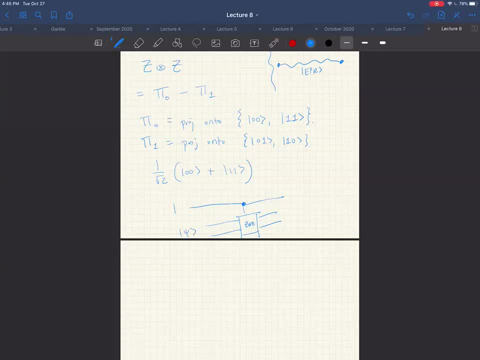 you wanted to measure like some state psi using, like some two qubit state psi using ZZ. uh, one way to do this coherently is, um, you would initialize a, an ancilla, in the, I think, the plus state and then, based on this plus state, you do a controlled operation, you do this control ZZ. 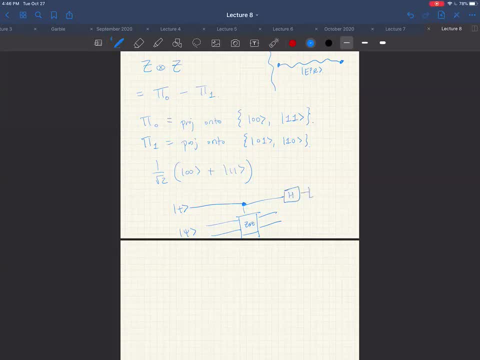 right, you do a Hadamard and then you measure, and so when you measure, you just get a zero or a one, and the claim is that, conditioned on this being a zero or one, you're going to get the appropriate post-measurement state out here. okay, so kind of a digression, but I think it's an important point, like: 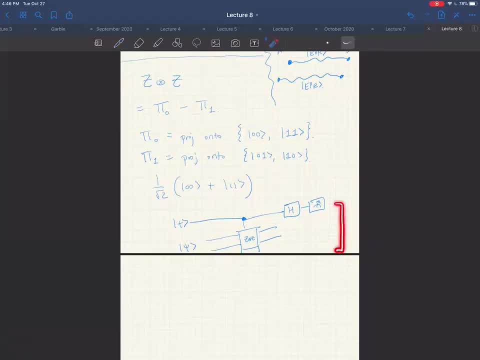 this is how you do, like a non-destructive measurement, because you you know, after you perform this measurement, you could still have some entanglement remaining between these two qubits, and then that's important. so essentially for the ZZ case, what's going on here? it's that, like um, 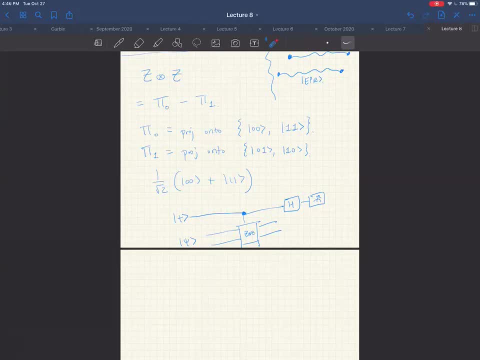 you actually measure in the standard base basis that that is zero, zero, one, one, zero, zero. but then you group two of the uh outcomes to be like, say, one, and you group the two other uh outcomes to be z, z, zero, zero. right, exactly so uh. in in this measurement you're only learning the parity between the two bits, but 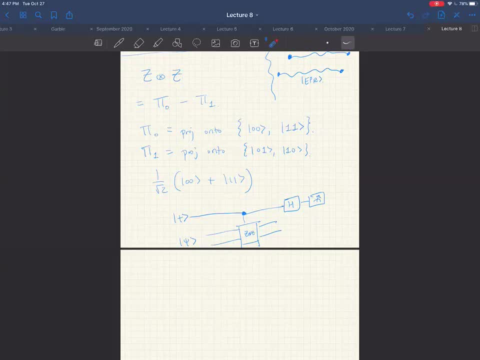 you're not going to be able to learn the the values of the each two bits. so so it's slightly less destructive than measuring each qubit separately, and something that happens here is that, even though they'll have the same bit value output, if you were to just do ZZ on x and with roughly 10.5 on x and with Special 1, if you were to just do z on compromising, the first point shall lose until zero. 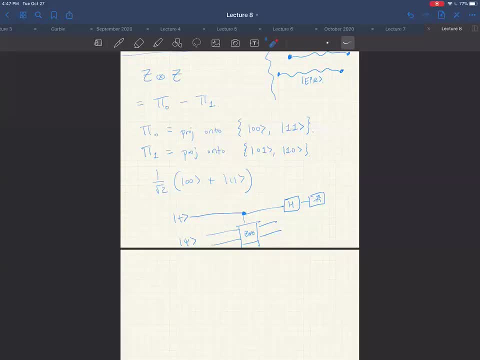 could turn to insufficiency: right one, do z on the other and multiply Like. we've still got two versions that'll come out one, two versions that come out with a negative one. What makes this non-destructive is that by attaching them to this ancilla qubit, you aren't getting out the information about that state. 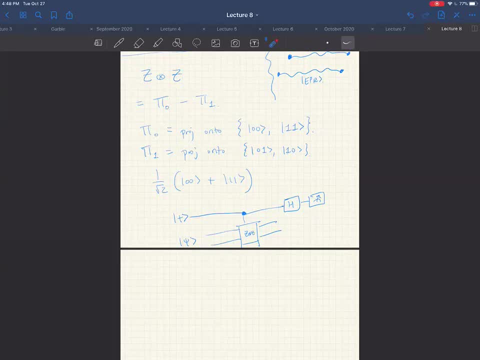 You're not assigning values to it. You're using another qubit to capture the parity rather than make assignments through measurement. Exactly, You're basically just minimally extracting just the information you need and not like. if you extract too much, then that actually damages the state too much. 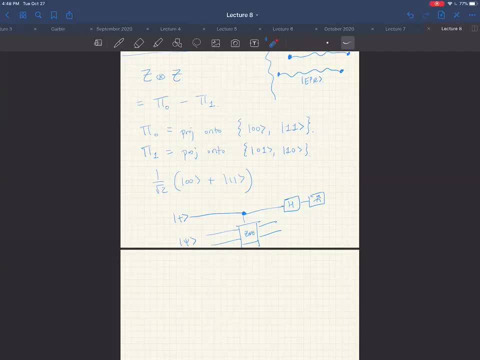 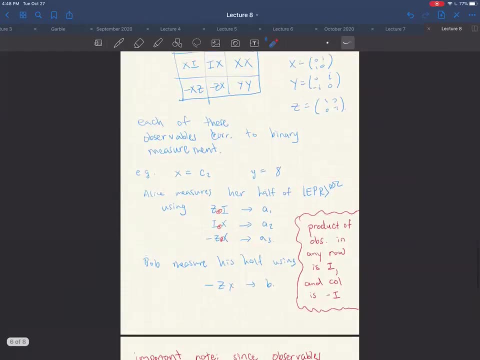 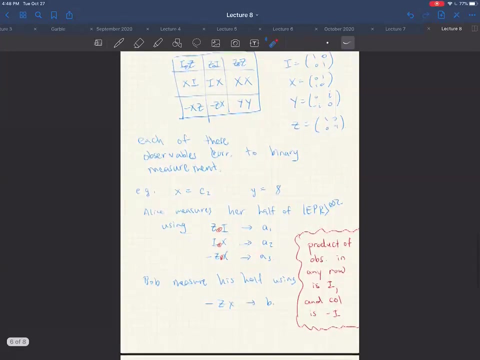 So that's another way of thinking about it. Okay, so blah, blah, blah. where were we? So that's an overview of the strategy, and I guess I was saying the reason that the parity constraints are always satisfied is because this sequence of operators has the interesting property that 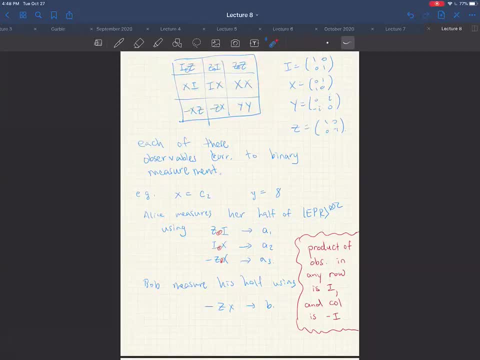 if you multiply along any row, you're going to get identity, whereas if you multiply along any column you're going to get minus identity. So it's kind of like it's impossible to assign zeros or ones to these squares to satisfy all the parity constraints. but if you allow yourself to stick in, 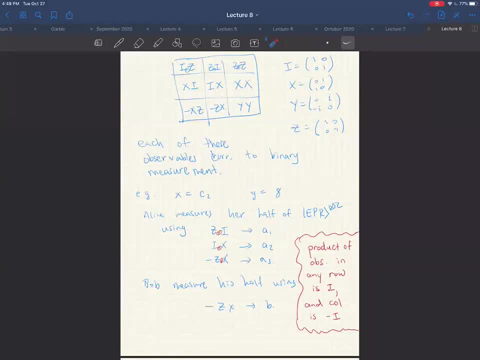 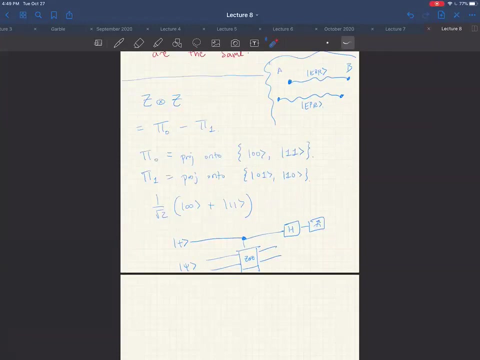 operators, then it then becomes possible. So this is what this is capturing, Henry. it occurs to me that there's one thing I'm still not clear on about what Bob and Alice's answers do when they're both sent to the referee. Does Bob have to give the same answer for that cell? 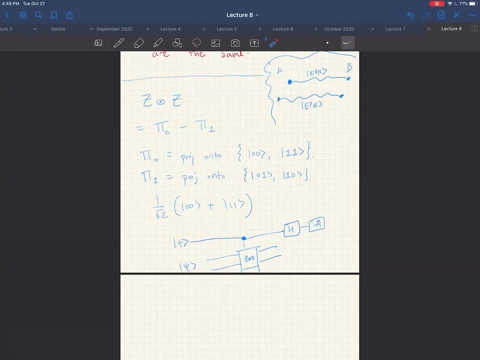 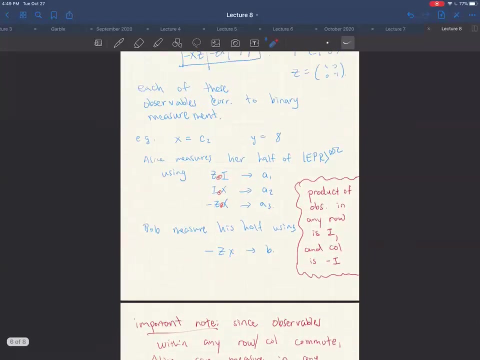 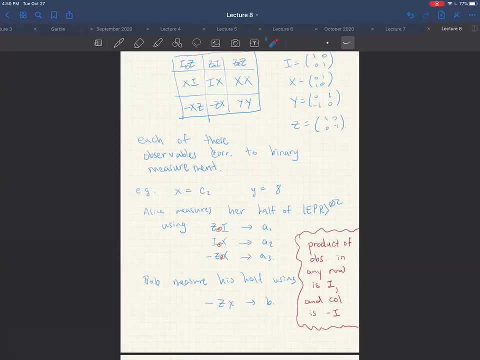 as Alice, Or does Bob's answer need to insert into Alice's strategy such that what sh Like, say, A1 and Bob happen to be the same cell? Does that make it so that B, A2, A3 has to satisfy Or independently? A1, A2, and A3 satisfy and A1 equals B. 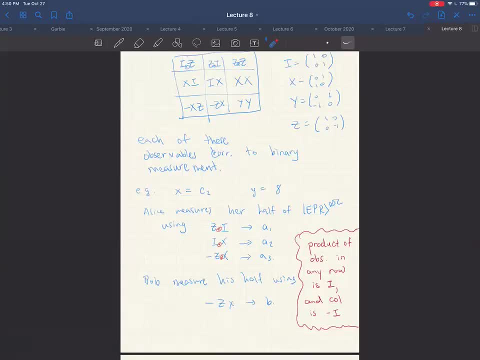 It's the second thing you said. All right, Well, I guess they're equivalent because, Well, I guess they're equivalent because, Well, I guess they're equivalent, because If A1 is supposed to be B, then Then, 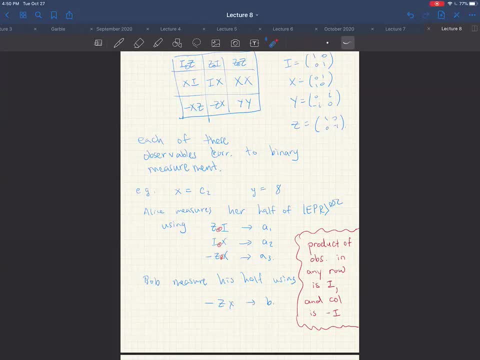 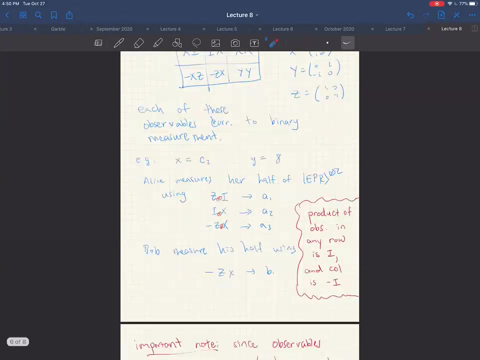 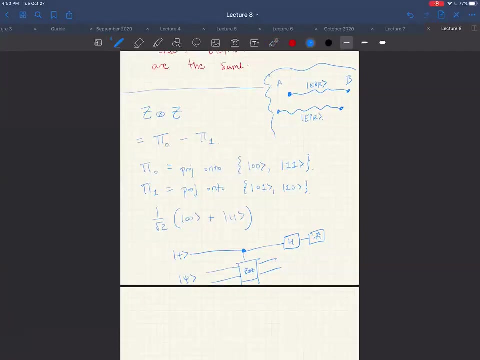 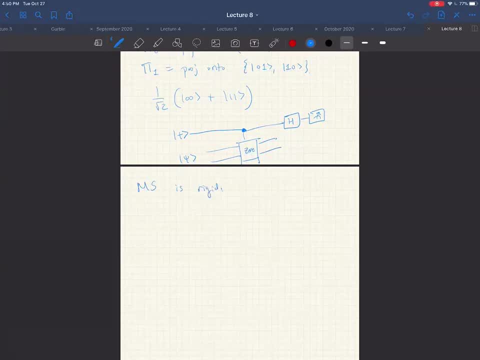 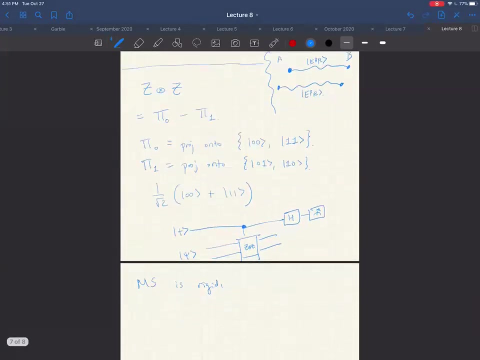 is rigid and you know I won't spell out all the details. It's basically the same thing as the, the, the CHSH rigidity: any strategy that wins with probability one or close to a hundred percent. There has to be local isometries under which their strategy looks like the thing I just wrote. 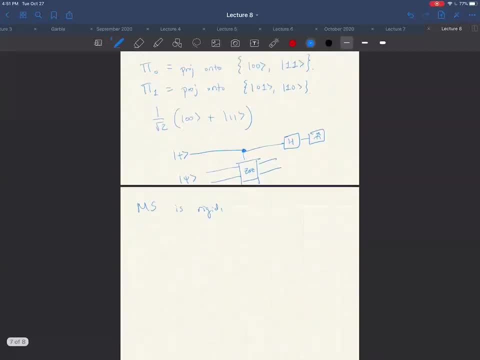 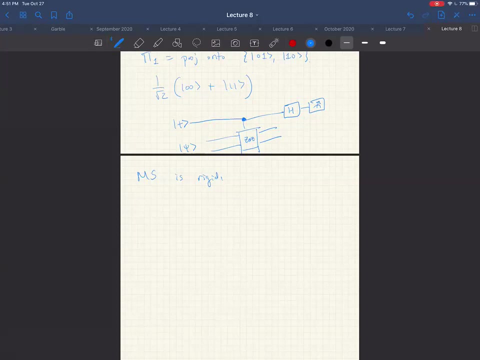 Right, There's no way around it. They have to be doing this two qubit strategy and applying this. you know this interesting sequence of observables And that's it. You know they could be using like a huge D dimensional strategy, but most of that will be. it's just some junk state. 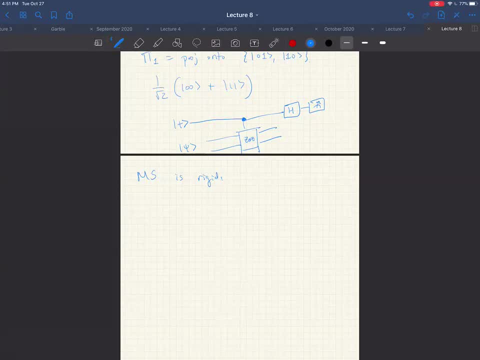 that that's not used at all. Okay, So, so, that's cool. So this is a non-local strategy, So this is a non-local strategy. So this is a non-local strategy, So this is a non-local game with a hundred percent winning probability. So what? what about the direction in terms of 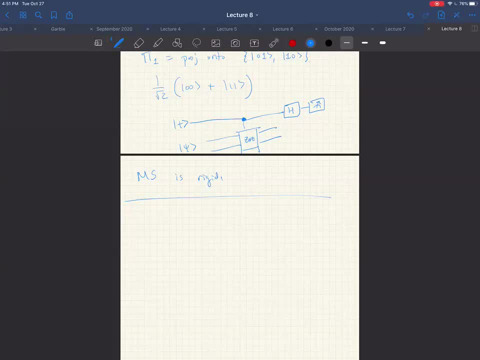 trying to certify more entanglement. So CHSH certifies one EPR pair. the magic square game certifies two EPR pairs. What if you wanted to certify more? Like you know N EPR pairs. So there's a simple game to certify two N EPR pairs. 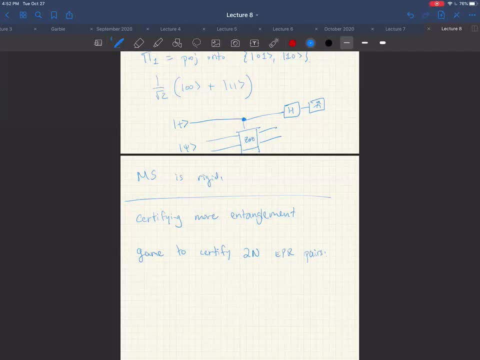 Does anyone have any suggestions for how one might do this, At least a natural approach that you would take? Can you repeat the question please? Yeah, Like if you were to design a game, like a non-local game that you know has quantum value. 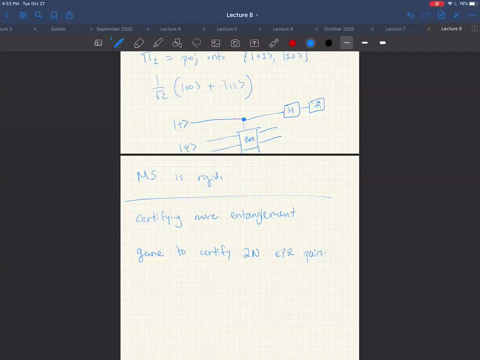 that's higher than its classical value, and any strategy that achieves the optimal winning probability has to be, you know, isomorphic to a strategy that involves a lot of quantum value, And so this is a non-local strategy. So it's a non-local strategy. 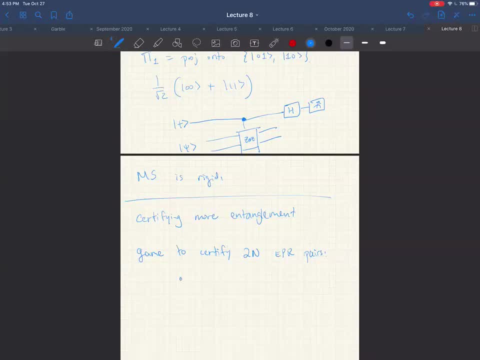 So it's a non-local strategy And it's a non-local strategy, And it's a non-local strategy, So it's a non-local strategy, So it's a non-local strategy, So it's a non-local strategy. I'm going to go out on a limb and say that you just need to construct something where Bob answers one bit and Alice answers. 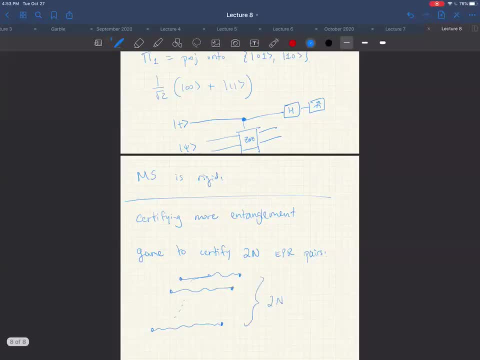 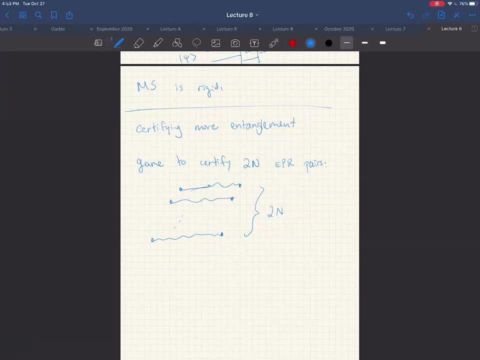 gives them N minus one bits in her answer. with N EPR pairs You like on. you know, on some level you can just generalize the magic squares to more dimensions. I like that suggestion. Like magic cubes, magic hypercubes, going deeper and deeper and deeper. 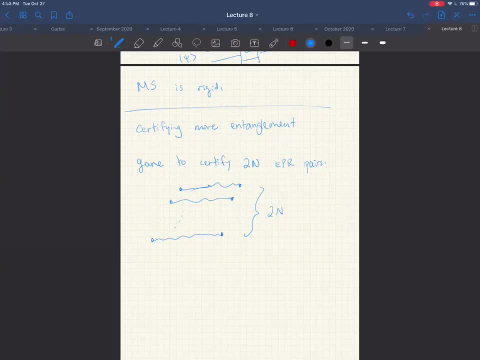 Uh-huh, Yeah, that's an interesting suggestion. They have to get longer and longer and longer as well. So making sort of like generalizing it, the magic square game to like sort of be bigger dimensional, is the right idea. 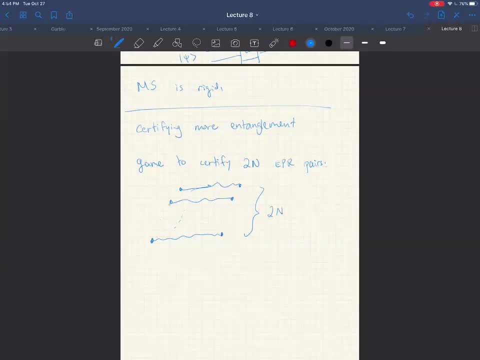 One way that this could work. I guess the thing that I had in mind is something called the what's called the parallel repeated magic square game, And basically the idea is you just instead of playing one instance of the magic square game, 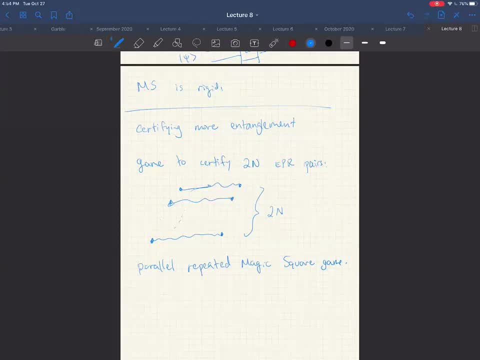 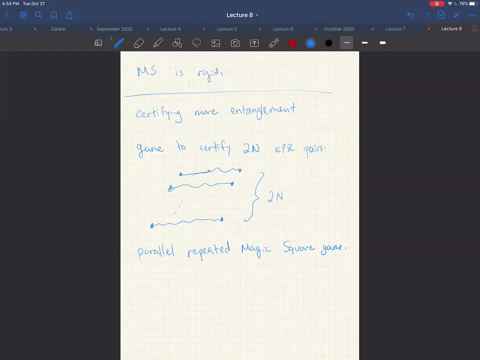 you just play N of it, N of them all at the same time, right? So like, have you ever seen those? you know those chess masters that are going around playing like a hundred simultaneous chess games with you know little kids. it's kind of like the same idea, right? 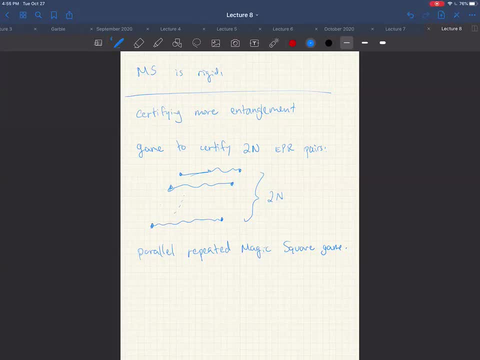 Instead of playing one chess game, you play like a hundred of them, and you actually certify the existence of not just two EPR pairs, but two times 100 or two times N. So we still have two players, but now they're supposed to be playing lots and lots. 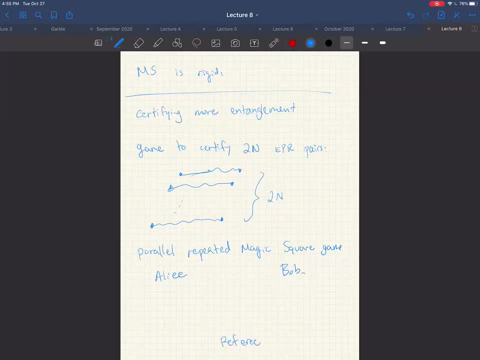 of copies of the magic square game at the same time. So the referee is going to, like, you know, imagine that there's like many, many copies of this three by three grid. You know there's there's instance one, two, up to N, and for each of these different three. 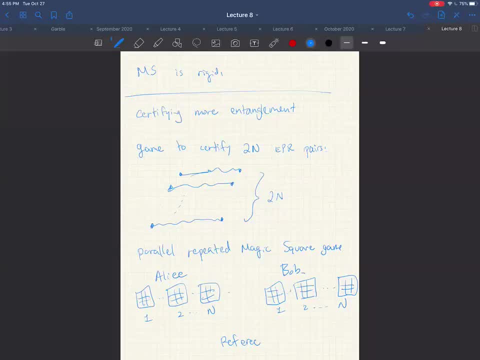 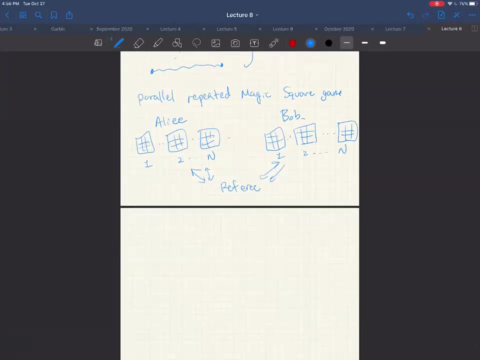 by three boards. the referee is going to pick a random row and column and also pick a random cell within that row and column, And so they're going to. Alice and Bob are going to have to simultaneously respond with assignments to all of those cells and they have to win each. 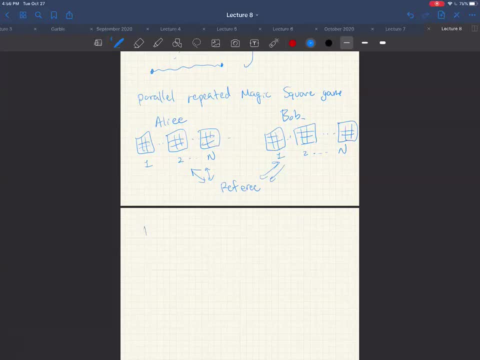 of those magic square games all at the same time? Is this at all different from just playing like two N CHSH games? That's a great question. Just give me one second. So let me just write down what the rules of the game are. 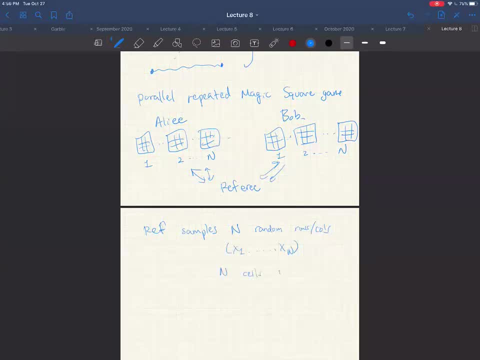 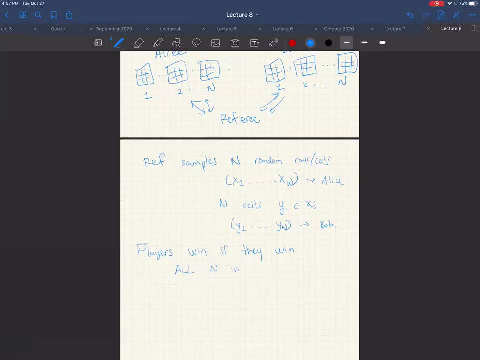 So there is one rule. there is one rule. it's like I have a little bit of a. I've got like a, a, a, I don't know- a, a demon, I mean, I don't know why people don't use demons. 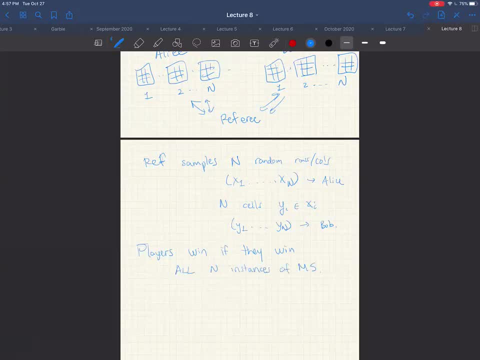 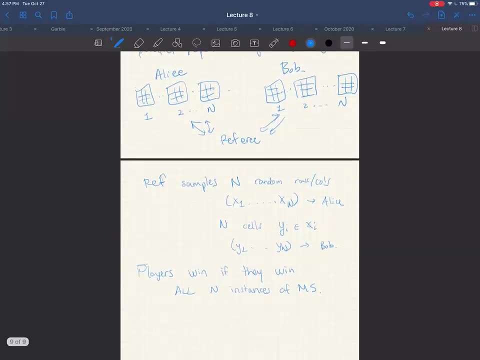 I don't want to be like you, Okay, So before I answer Ariel's question, so I've defined a new game, right Like? here are the rules of the game. here are the questions and answers that they're supposed to respond with. 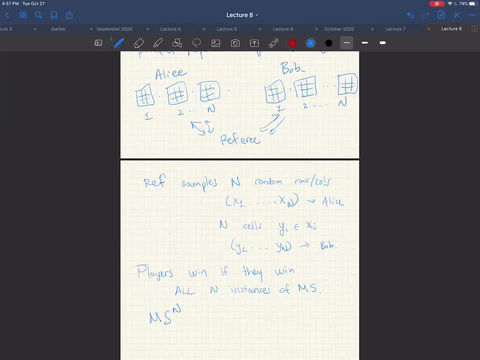 So I'm going to call this game MS, raised to the N for obvious reasons. So you can ask what is its quantum value? What is the optimal quantum winning probability for this repeated game? Why It should still be one? Yes, because, Because it's a protocol on each one of them. 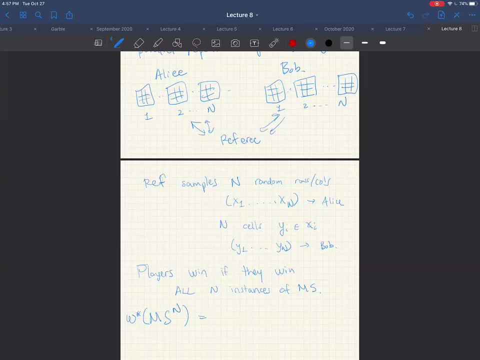 Right, Like the players will just be like: all right, we're really good at playing individual games with 100% probability, So we'll just do that separately And times what are the resource requirements for this game? Like what the strategy will just be. 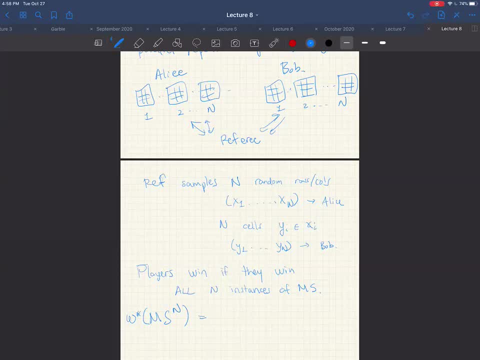 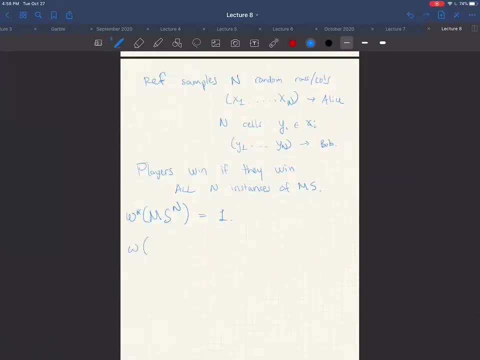 N copies of the original one. So that involves two Ns, Two N EPR pairs, right, Okay, So so this is one, The classical value. any anyone have any guess? So remember that the classical value of the original game is less than one: It's 17 over. 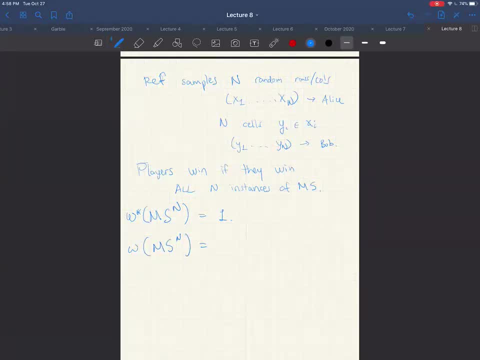 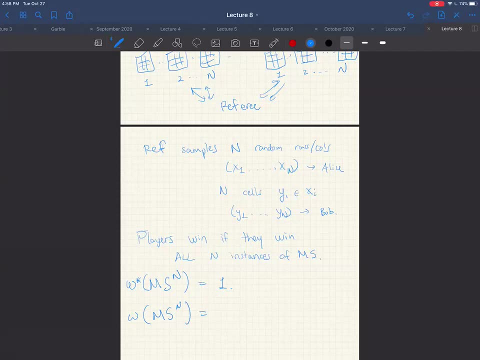 18.. So what's the classical value of MS to the N? 17 over 18 to the N? Very good guess, but that is not true, Which is really surprising. It's not 17 over 18 to the N. 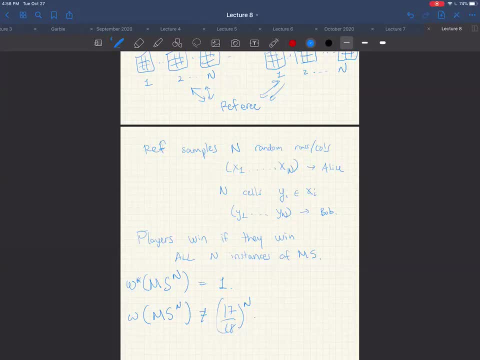 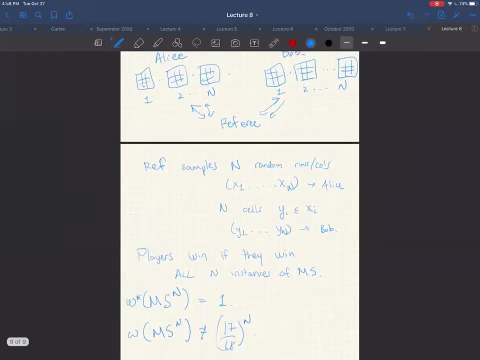 which you think: well, why not? Because all of these games are independent. So why, you know? why don't you just, why couldn't they just like play them all independently? So the reason that it's not so straightforward is because Alice and Bob actually see all of these. 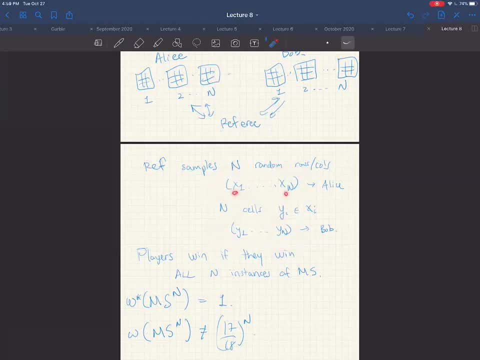 options all at the same time. So Alice sees X1 to XN all at the same time And in principle she can use a strategy that treat that doesn't treat all of the games separately. Like she could use some information about game one to decide what her answer is for game two. Why would she do that? 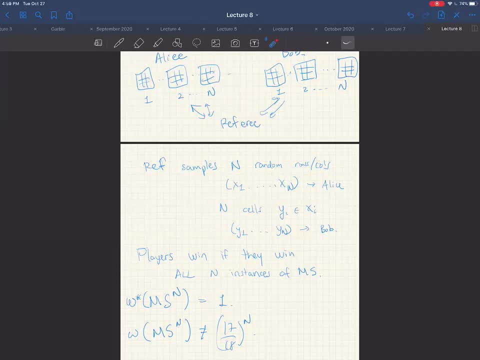 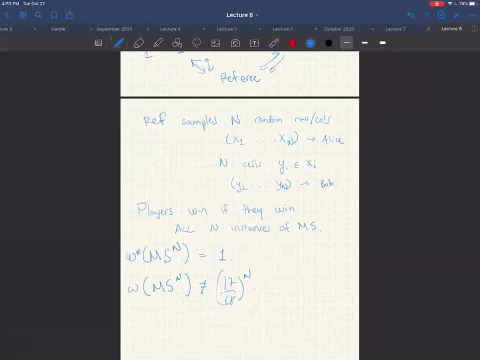 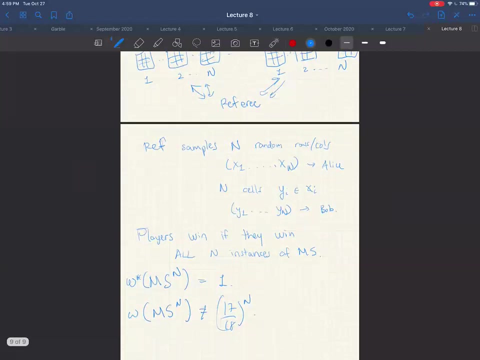 It seems like it shouldn't help her because they're unrelated games, but this can actually help Alice and Bob. So there's, it's actually a really. this parallel repetition of games is really strange, And it takes a lot of work to show that in fact, this, the classical value of this game, does decay. 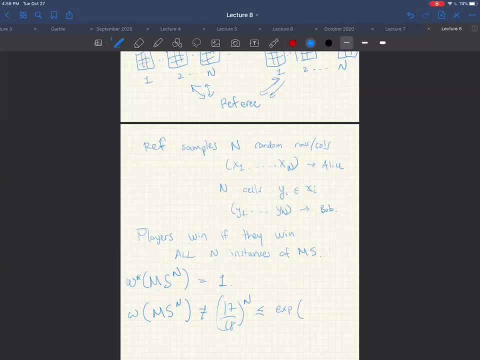 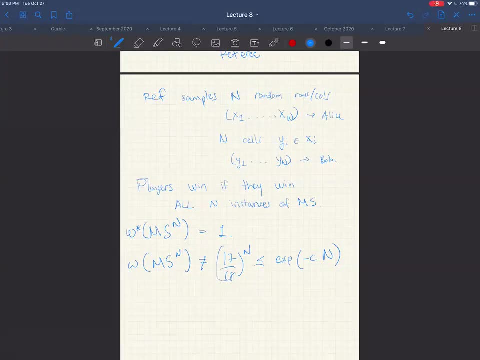 exponentially. but it's not this simple 17 over 18 to the N It's. it does decay exponentially with the number of games, but at a rate that's kind of funky, But it is as N goes large. this does go to zero very, very quickly. 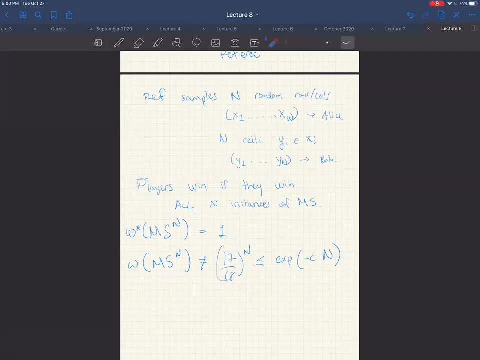 Is it this? is this algorithm similar to the one for the CH SH, the one that achieves 0.81 to to the power of N for parallel CH SH games? Oh, oh, you mean what the bound here is? Yeah, 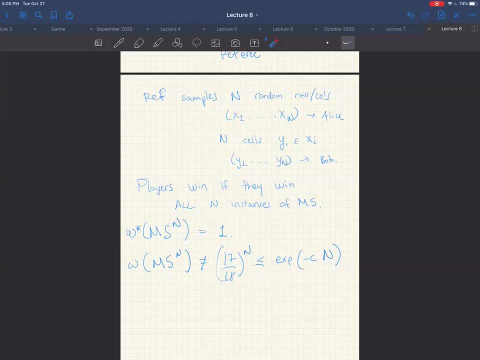 I actually don't know. No, no, no, no, Of course the bound be different. I'm asking if the protocols that beat this trivial answer are similar to one another. I actually don't know, off the top of my head, what is the classical strategy that beats this. 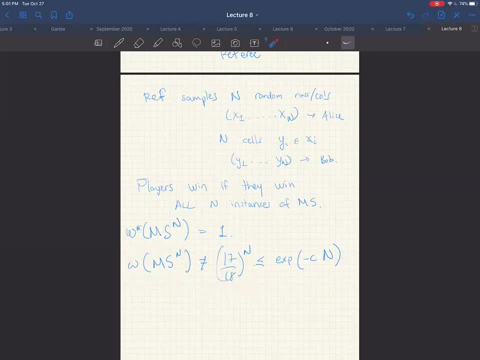 Maybe I'm missing something, but an idea for a classical strategy is: you know, both Alice and Bob just always return one for everything. So you know, 50% of the time they're going to have gotten lucky and Alice will have been asked a column and they'll win. 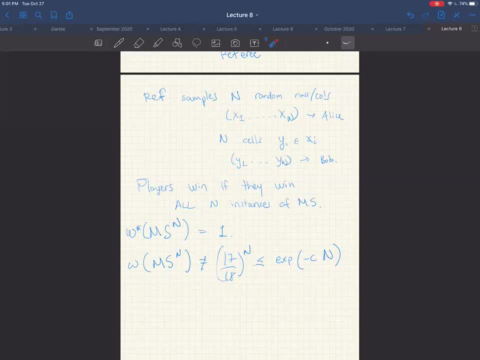 So that one will have a probability of half to win a single copy. then to win n copies, this will win with 2 to the minus n, which is actually much worse than this. Like, so clearly, like, okay. so I claim that for the single copy of the game they can do 17 over 18.. 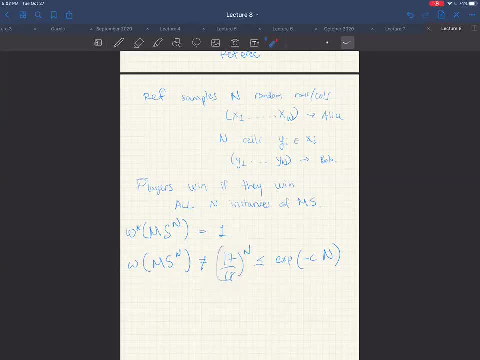 And if they just naively play n copies of those independently, then really their winning probability is this. But I claim that without proof that there actually is a classical strategy, a deterministic strategy, that allows them to win, with probability that's actually bigger than this. But they cannot beat this exponential, decaying band. 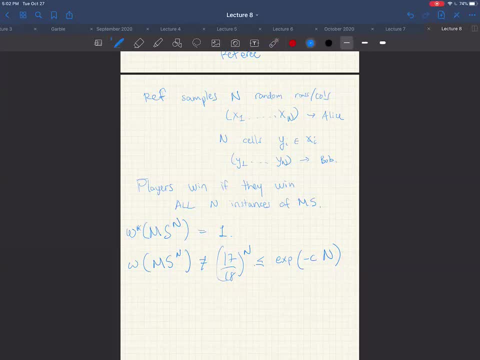 They have to output their answers all at the same time. right, For every game All at the same time. yeah, So they're just using like the question, like the fact that they have the question for every game. They don't have another strategy. 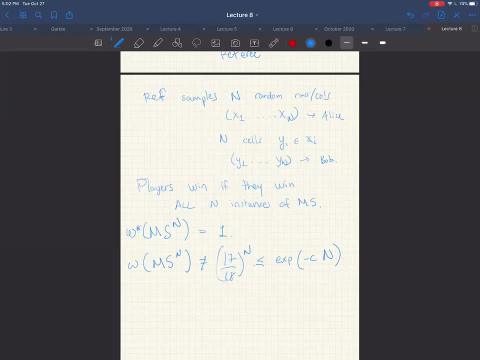 Yeah, That's cool. Yeah, If you're interested, I don't know- at some point I can give you a simple example of a game that like, just you know there's nothing quantum about it, You just have a classical strategy. 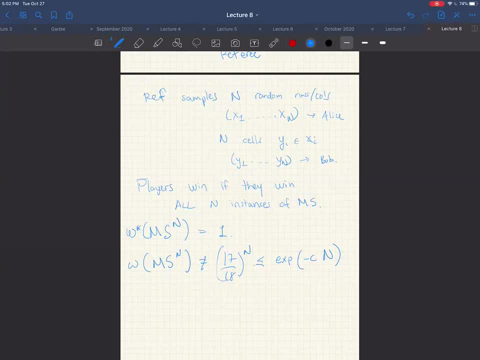 and you repeat the game twice And there's a strategy for the repeated game that has the same exact winning probability as the single copy of the game, And that's because they can sort of like cross-correlate their answers in this. 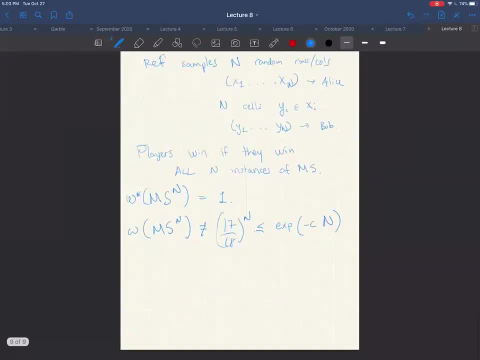 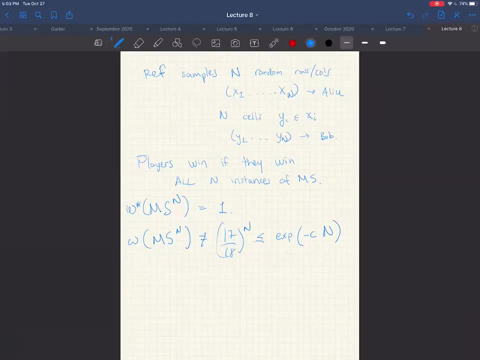 Okay. So yeah, Something that's kind of weird to me here and it's also a little weird in the CHSH games- that actually playing the game just once doesn't tell me whether, like I'm the referee, say, 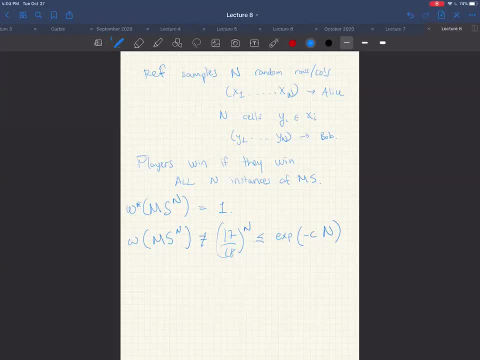 And by being the referee, I'm trying to see if something is outputting EPR pairs, And I do that by telling my lab assistants, Alice and Bob, to go play this game and I'll give them these assignments If I play the game just once and they win. I have no idea if they. 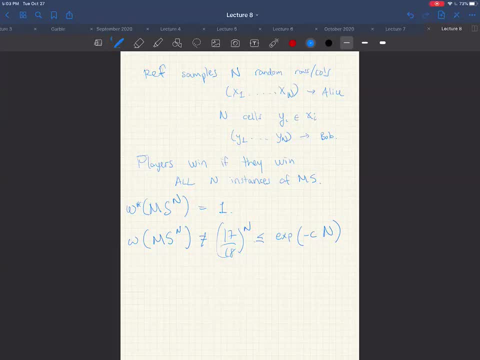 had an EPR pair. I need to keep going, and going, and going until I start converging on a probability, on like a frequency of one, two, three, four, five, six, seven, eight, nine, 10,, 10,, 11,, 12,, 12,. 13,, 14,, 15,, 16,, 17,, 18,, 19,, 20,, 21,, 22,, 23,, 22,. and I'm still trying to figure out how to play this game and it's becoming more and more difficult. if I'm starting to think I'm winning. 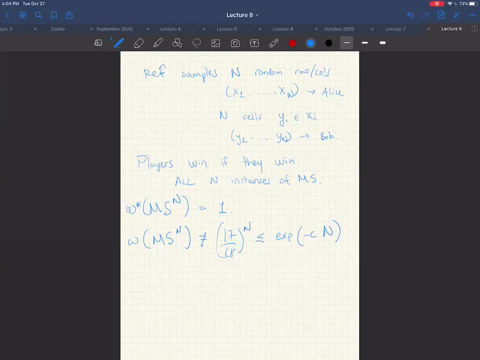 Such that I start to think that we're drawing from the EPR generating distribution, and 17 over 18 is already really, really high, And so the number of times I need to play this game to like feel reasonably convinced that. 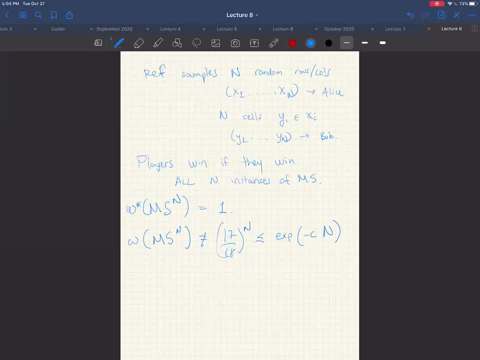 we'rewell, 17 over 18 is high. but that thing with the one is that if they lose once at all, I know that they're not drawing from the strictly EPR generating distribution Right, But if they have just like a barely faulty EPR generator, 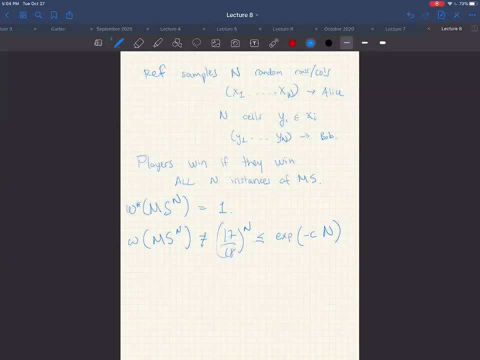 Right, It'll be very many games to tell like the barely faulty EPR generator from the classical strategy. That's a really good point. So I guess there's a couple right. So you know, in terms of like experimental usefulness, like to like tell whether you have a good EPR generator. 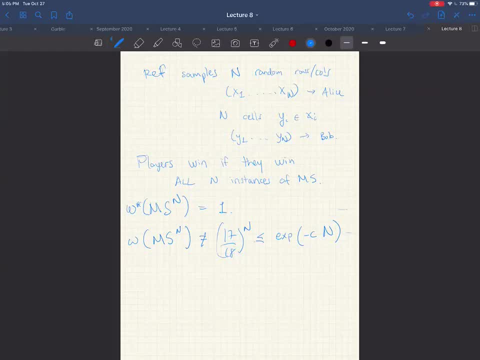 the magic square game is not necessarily the best one, because the gap right, Because one in 17 over 18- is small. Actually, you're better off using the CHSH game for that. So that's certainly true. Another point is like by repeating a game. 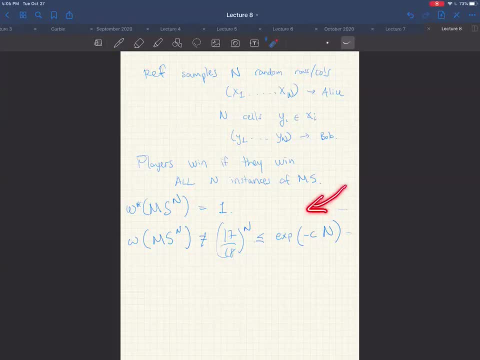 I mean, this doesn't fully address the concern, but by repeating the game you can amplify the gap. So here we have a gap between one and something that's exponentially small. So, at least in terms of the gap, this is much more useful. 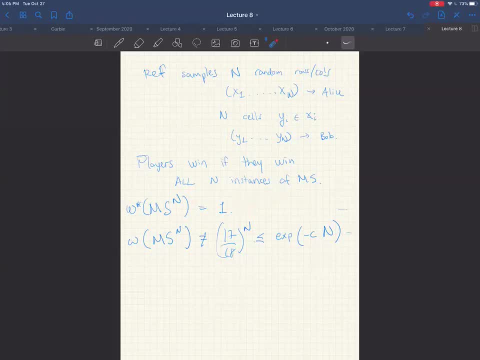 But, of course, how do you obtain this? Well, you need N copies of the EPR generator, So you know. so this is something actually people think about, Like can you design other kinds of games? or in the physics world they call them Bell inequalities. 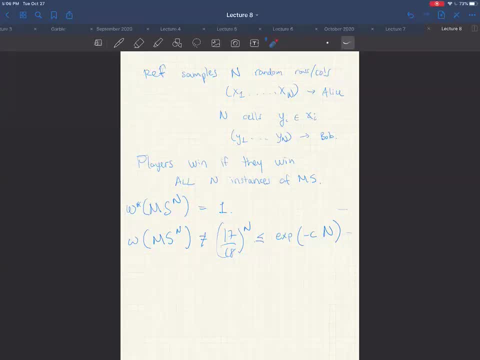 where they're much more robust towards, you know device imperfections and stuff, but you can still certify the existence of like an EPR pair or something like that. To go back to Ariel's question, you know how is this? Is this any different from repeating the CHSH game? 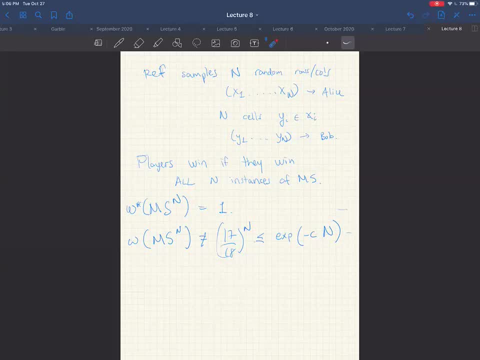 You can play exactly, do exactly the same thing, Like repeat the CHSH game and times, but there's a major issue with that. Can you see why? Like The fact that it's not one, it's also an exponential decay. Yeah. 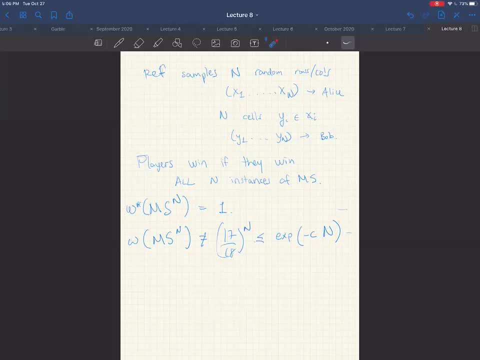 I mean you're gonna have exponential decay for both the classical and quantum values. One's going to decay slower, but it's still going to go to zero really quickly, Okay. so the final thing I want to mention before we take a break is that 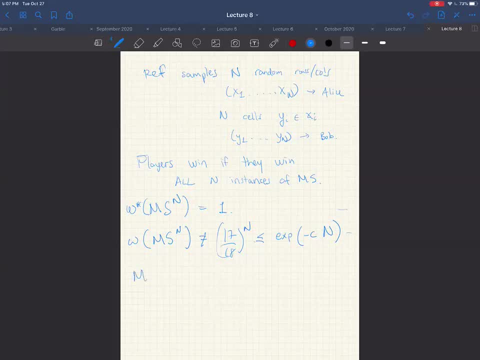 so here's the repeated game, and maybe it's not surprising that MS to the N is rigid. If you play optimally, if you went with probability one, you really have to have two N copies of the two N EPR pairs. That's not hard to prove. 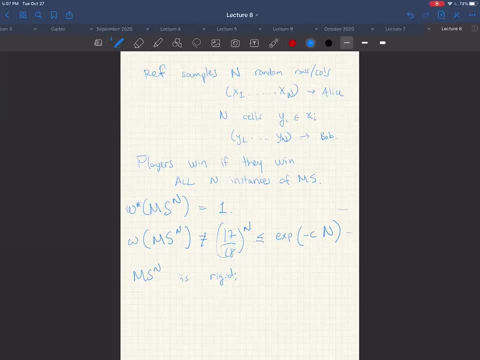 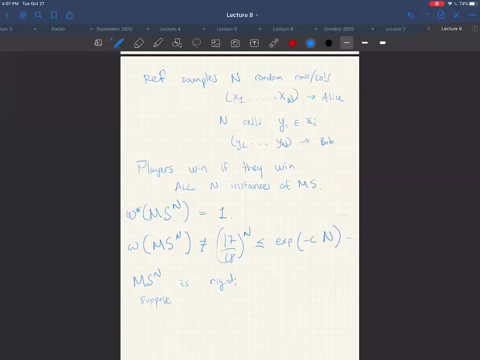 Like you can just, in a black box way, kind of derive it from the single copy rigidity. What's more interesting is the robust version. Okay, So suppose you have a strategy that wins with probability, one minus Epsilon. So think of Epsilon, is you know? 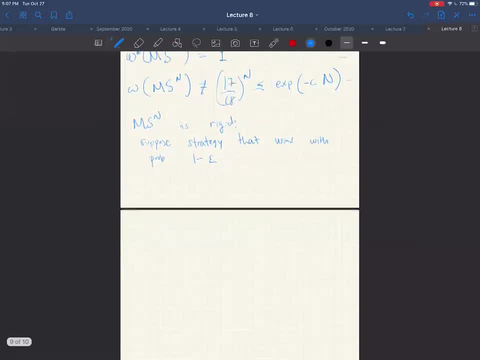 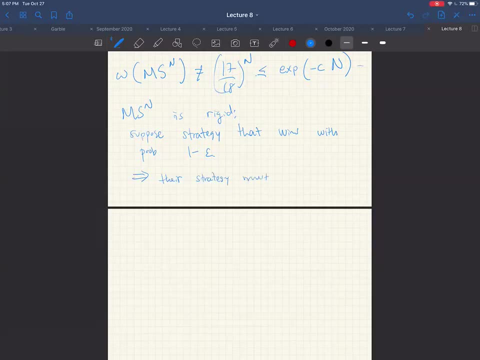 something small like 0.1% or something, then implies that their strategy under local isometries must be O of N times Epsilon to the one over fourth, minus N of O, of O plus O, and that's a good idea, Okay. So in this case, 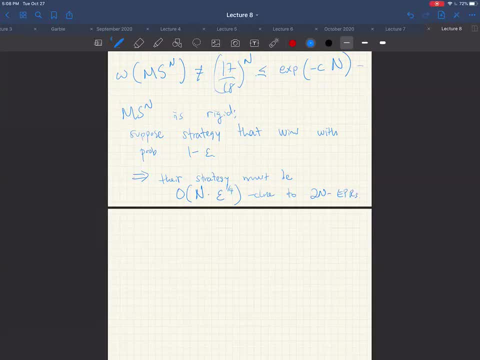 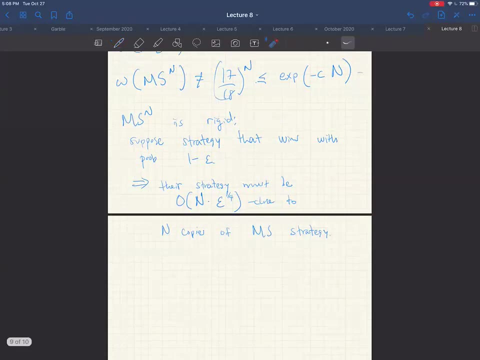 let's see if we can find some leg of something that's close to two N EPRs, One for each N. Okay, So this is the first one. So if you look it up on the right, you can see that there's one N. 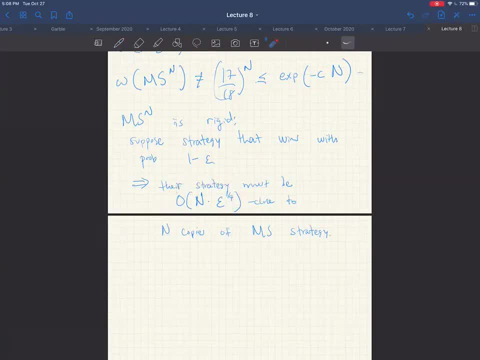 So I'm going to look at the upper two Ns here. There are some Ns here, Okay. Okay, if epsilon is really really small, like it epsilon is, you know, goes to zero as n gets larger, And so 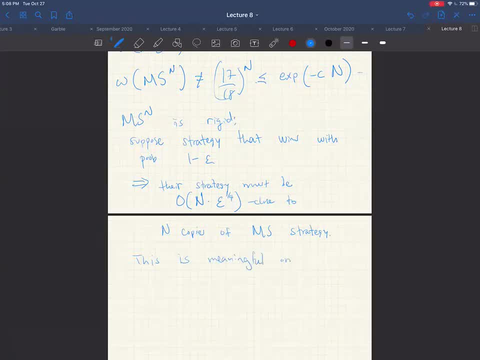 this is meaningful only when epsilon like less than n to the fourth, And so this is not super great because like in order, sort of to like connect it with. Sumner was saying: in order to get any guarantee, you really need to like. 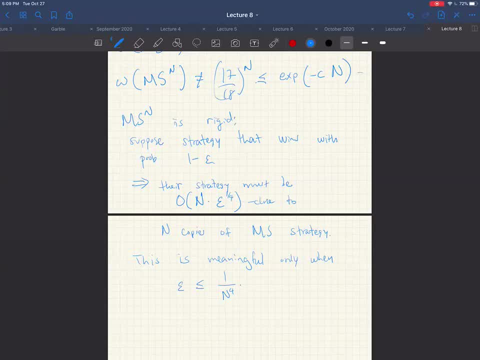 like: if you wanna certify, like a hundred, existence of a hundred simultaneous EPR pairs, then you need to check that they're winning, with probability one minus one over 100 to the four, And that will take a lot of samples to estimate. So at least you know this is not so practical. 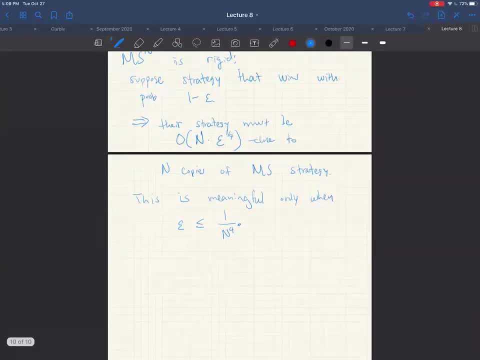 but you know, this is the theorem that we have And but people have worked to create more sophisticated kind of non-local games that can certify any EPR pairs where the robustness- like this, this closeness value, does not depend on n at all. 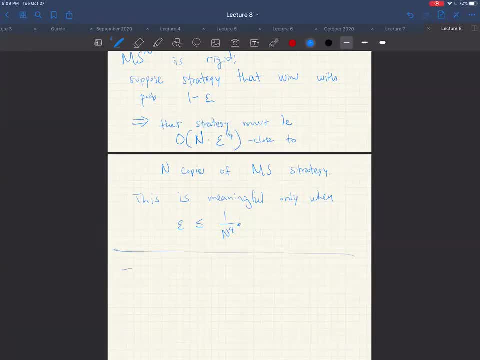 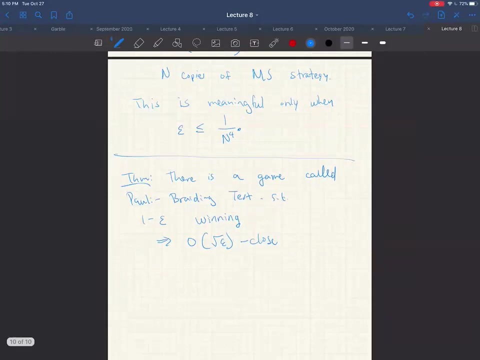 So I'll just write one thing. There's a game, There is a game called the poly braiding test. That's much better. in this regard. If you went with probability one minus Epsilon, then you're actually going to be squared and squared Epsilon. 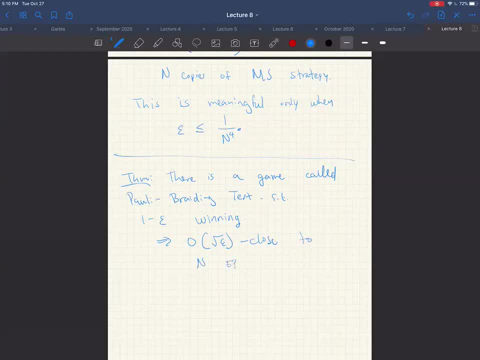 close to an EPR pairs, No matter what n is. So this is like a much more useful kind of non-local game. Okay, So let's take maybe like a five minute break, Let's come back at 5- 15, and then we'll see how we can use this technology in order to verify quantum computations. 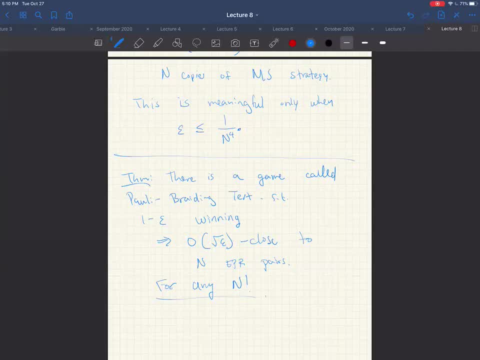 What if I restrict the amount of entanglement of entanglement. So let's say I'm giving you n copies of a game, but I'm allowing you little over n entangled states. Can you still design a game that you can win with probability one? 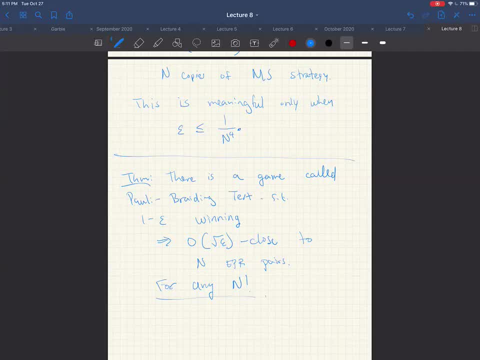 Great question. So if the original copy of the game, if like the single copy of the game, required, like so there's different measures of entanglement, but let's say it required like one E bit, like that's a measure of entanglement. 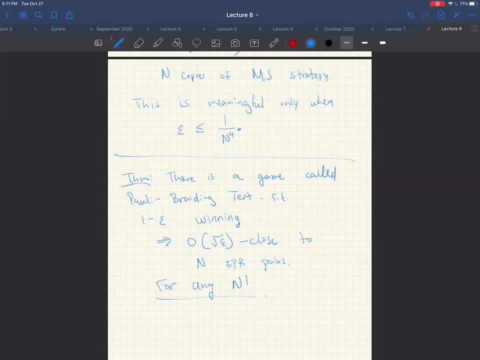 it's called E bits, one E bit of entanglement. then, in order to win with high probability in the repeated game, you essentially need a linear number of E bits. So you can prove that- Yes, this we can prove, Even actually to do anything better than exponentially. 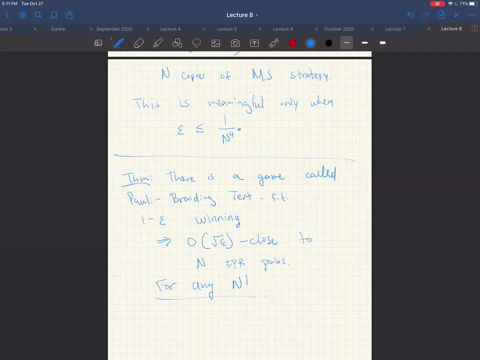 you know something exponentially small: you need a linear number of E bits. Okay, So we can prove this, but it's not quite a rigidity statement because it only says the says the amount of entanglement is linear in n. 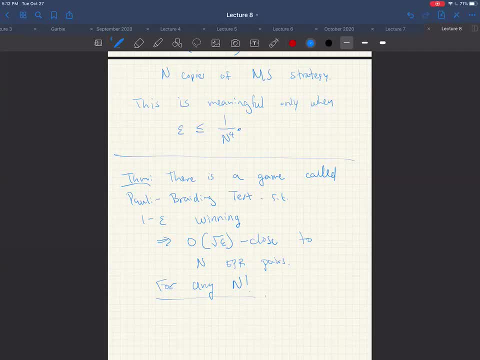 but it doesn't tell you structurally what the entanglement has to look like. So that's actually like an open research question. Okay, So that's actually like an open research question. Okay, Okay, Okay, Okay, I see. 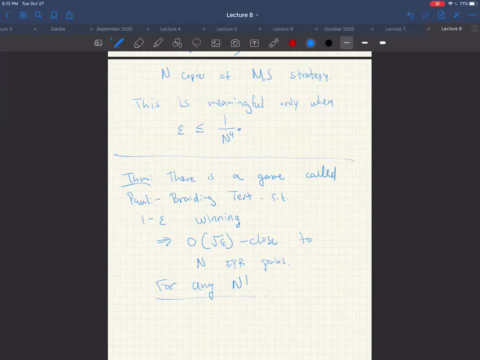 So it could be that, like for a single instance of the game- the entanglement- the entanglement needs to be very complicated, but for n repetitions of the game maybe it doesn't need to be too complicated, If I'm speaking in the right terms. 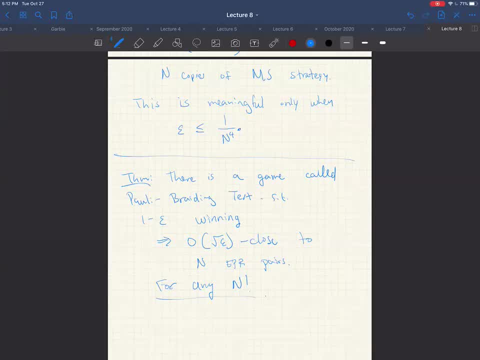 Yeah Well, I guess it's. the thing that people are wondering about here is all of these rigidity statements, like we only know how to say- we only know how to say meaningful things and what's called like the high winning probability regime. 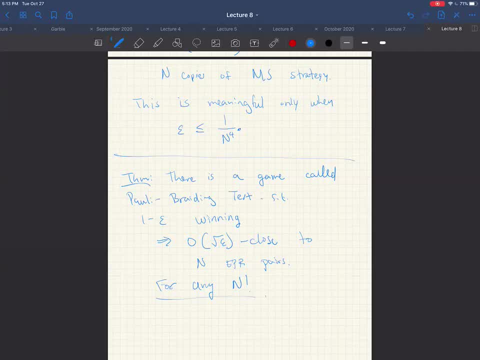 like something that's very close to one 99% or. but what if you're only winning with, like this repeated game with, only, say, 25%? this is still very good because the classical bound is exponentially small, So 25% is much better than that. 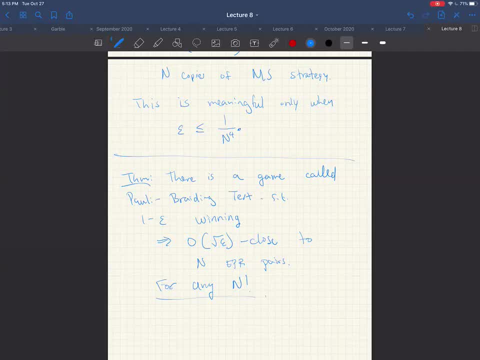 but we have no idea what to say about their strategy in that regime, Like it must be doing something rigid, but at least that's our guess. but we don't know how to articulate it. Are there natural examples of games where you'd get this like 25% or 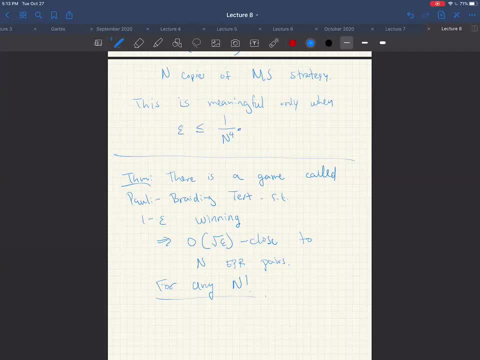 Well, like you can even like- for example, you can take this repeated magic square game. Like you know, something dumb that you could do is say: well, three quarters of the time I'm just going to sit and do nothing. 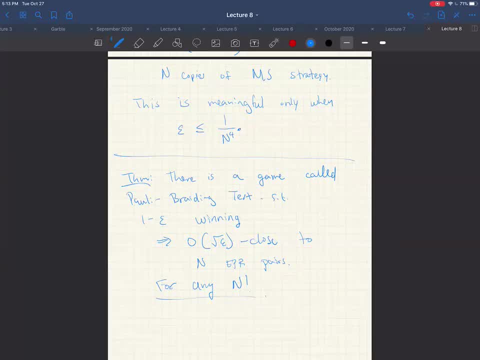 But 25% of the time I'll actually play the game. So so that's one example of a strategy. But there you- I mean you can see- like you can't get around using two N EPR pairs. It's just 75% of the time you decided not to do anything. 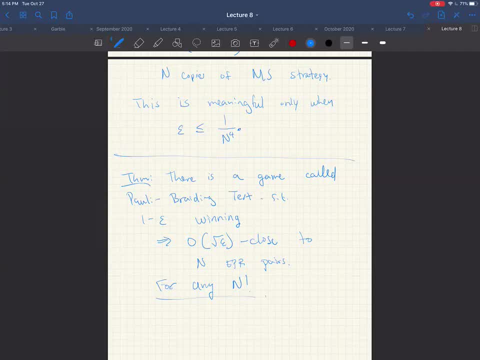 Yeah, So. so basically, the the open question is in this: in this low winning probability regime, can you still formulate a rigidity statement of some sort? Yeah, Yeah, I also have a question. So when we described closeness to N EPR pairs using complexity, 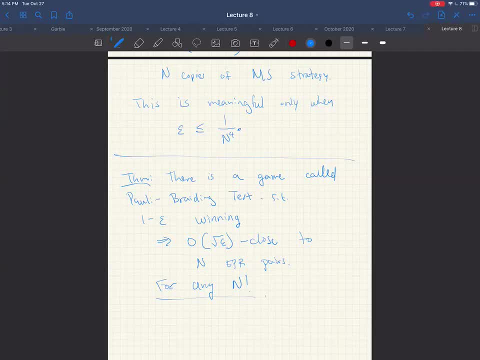 like all square root of Epsilon, is it related to one minus fidelity? When we say all squared of Epsilon, is one minus fidelity related to the square root of Epsilon, right? so i guess i didn't spell out what closeness means. um, there, there's one thing that you need to. 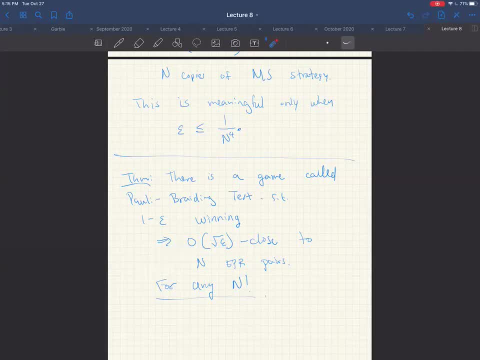 incorporate into this notion of closeness is you. you get to pick a choice of isometry for alice and bob, so you know they. there always has to be this freedom and changes of basis. okay, fine, then after that, um, the yeah, the closeness you can measure in terms of one minus fidelity, if you want, or 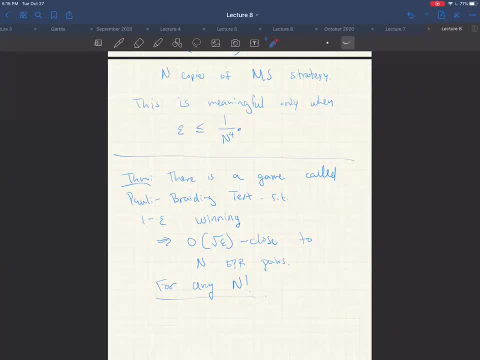 euclidean distance. it's not so important what choice of distance you use, like they're all essentially kind of equivalent up to square roots, um so, um. so we can- sorry, yeah, it's basically like what you said- up to up to a local isometry, so we can also measure the degree of closeness by when we change basis. 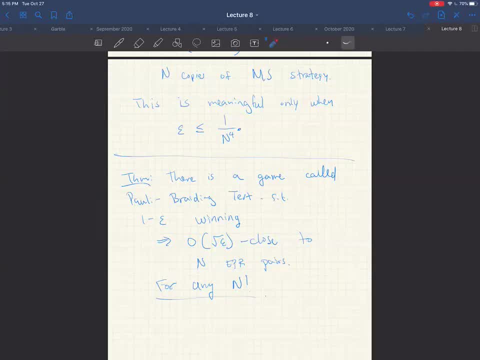 how much do we preserve the entanglement? right, yes, okay, thank you. i have one other one comment. um is a lot of this like certifying the existence of quantum states. uh, you know, in the process of certifying it, you can't you destroy the states, you can't, uh, like. 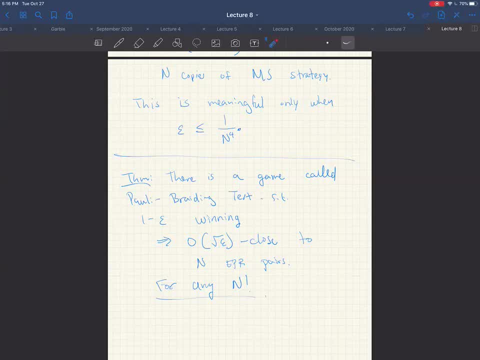 you can't certify that they have states, uh like, available for future use? that seems like an annoying restriction. yeah, great question. it's, like you know, in the process of certifying you actually destroyed the entanglement, so there's a way around it, which is you can sort of um, you can imagine that. 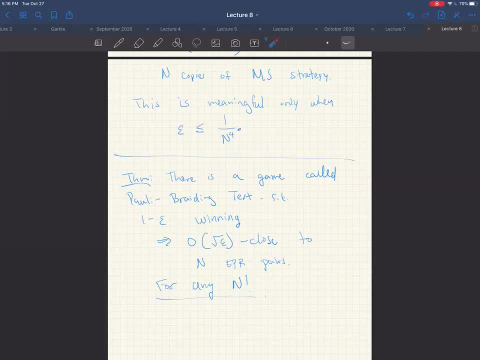 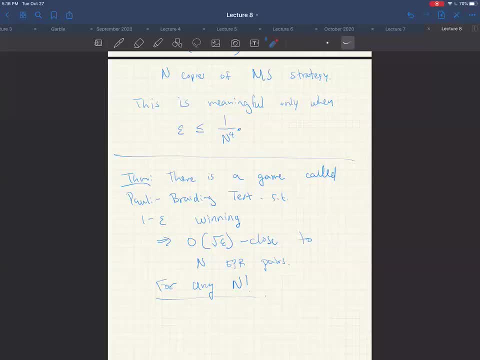 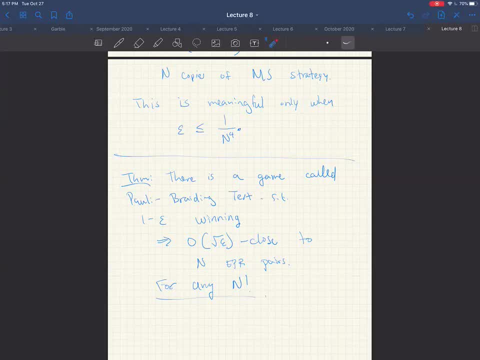 then you know that they must have um, a reservoir of epr pairs on hand ready to use, right? but let's say you randomly decide to say at like the the 57th game, you actually just stop um. then then you know that with high probability in the 58th game they're 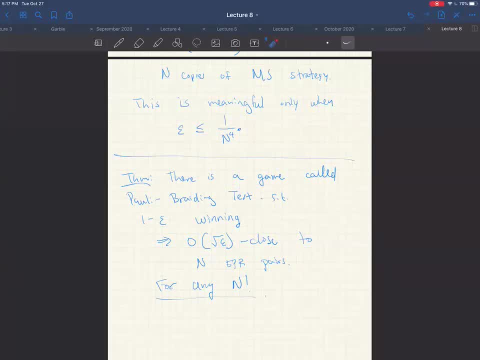 they're very likely to have a fresh EPR pair ready to use. So that's a way in which you can kind of certify that they would have entanglement ready. You don't tell them where you're gonna stop, You just randomly choose a point to stop. 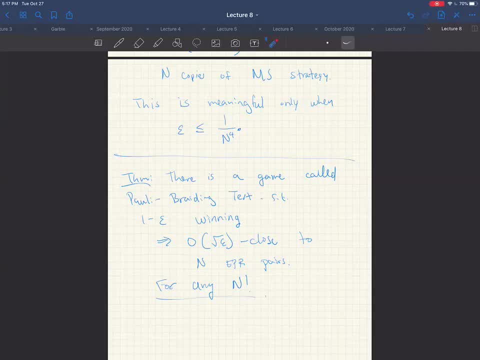 Yeah, I mean I can see why that's useful, but that's still kind of like regular, like maybe they're your best friend so you just believe them, Like there are all sorts of reasons you could have to think they have more EPR pairs on hand. 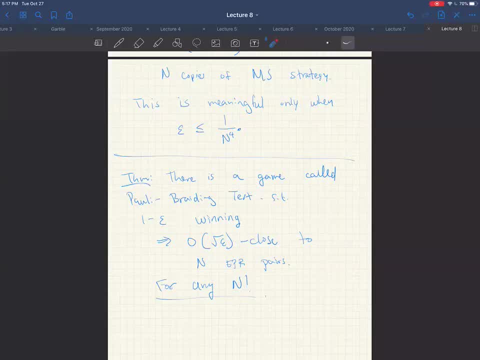 but there's no guarantee and there's no quantum benefits you can get from to be sure that they have those on hand. Well, in terms of quantum benefit, well, I guess we'll kind of see like. so this is actually, if you're playing with Alice and Bob. 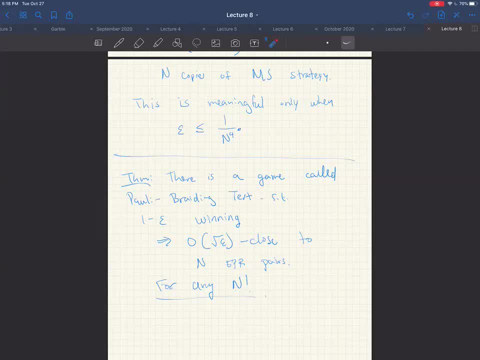 and you're sure that they're not communicating, then actually you don't have to trust them. Like, if at any moment they don't have enough EPR pairs, then they won't be able to win the magic square game with probability one. This magic square game gives you a way. 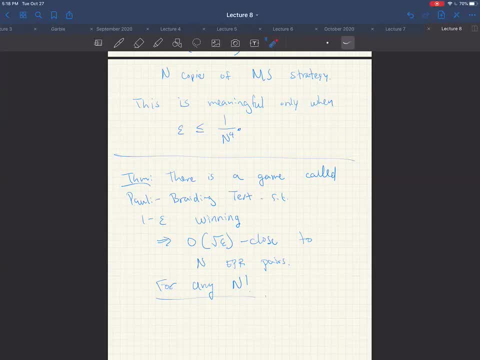 to test that they have enough, In fact, at least world of theoretical quantum cryptography and things like that, they use this magic square game as a sub protocol. They'll say: well, we want to use these EPR pairs to do something like: 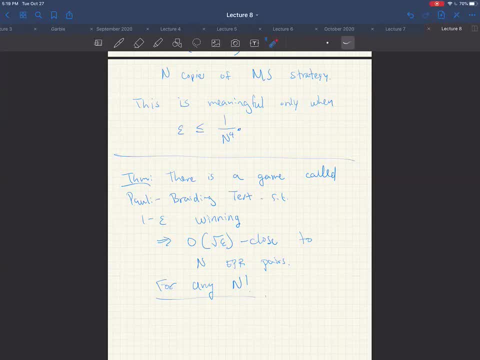 quantum key distribution or some other task. But how do we first check that they have these EPR pairs? Well, they'll pick a random number of games to play. They'll play the magic square game, play the magic square game, play the magic square game, And then, at a certain point, 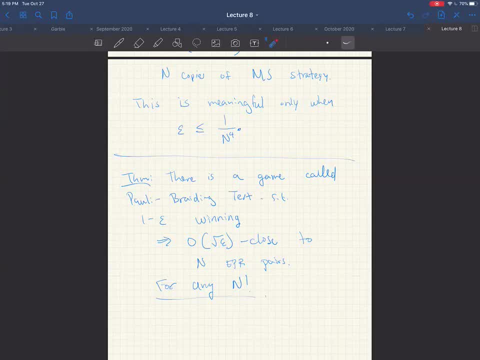 the referee is going to be pretty certain that they will have an EPR pair ready to go for the next round. So then the referee will just switch to performing the other protocol And the players won't necessarily know. The players won't know that they're suddenly being asked to play a. 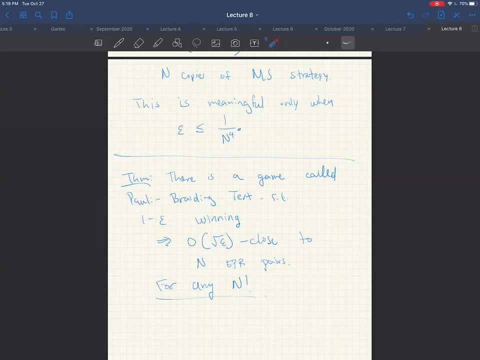 different protocol, And this way you can actually leverage this rigidity guarantee to do something else that's useful. Actually, this ties exactly into the thing I wanted to talk about next, which is how do you use this to certify quantum computations? So maybe I'll jump into that. 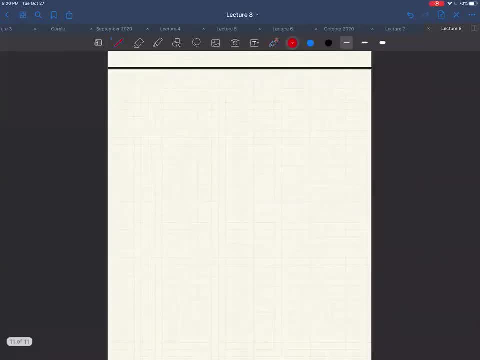 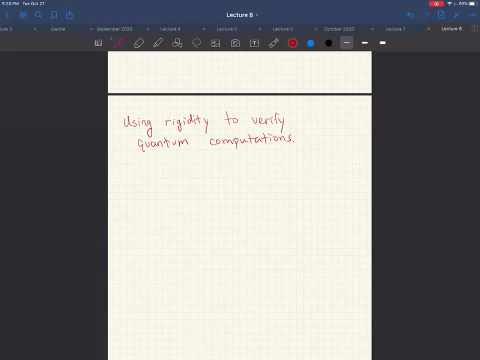 So let's start a new page, Okay, Okay, Okay. So let's go over the setup. We have a classical verifier or referee, like they're the same thing. So let's say that the verifier has an n-qubit circuit in mind. 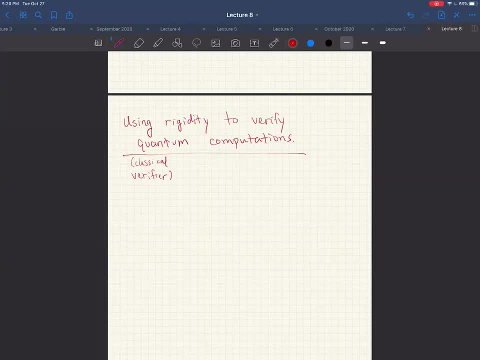 and what the verifier really wants to know is what happens if I ran the circuit, let's say I initialized it to all zeros, did some polynomial time computation and measured it. I want to know if it accepts with probably high probability or accepts with low probability. so let's call it the 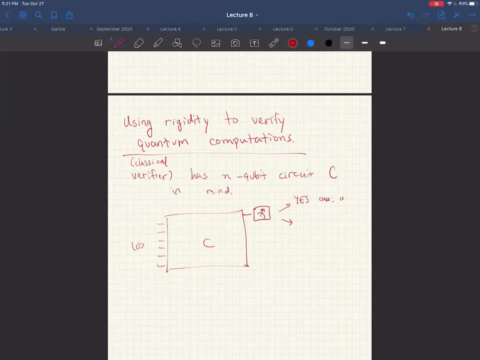 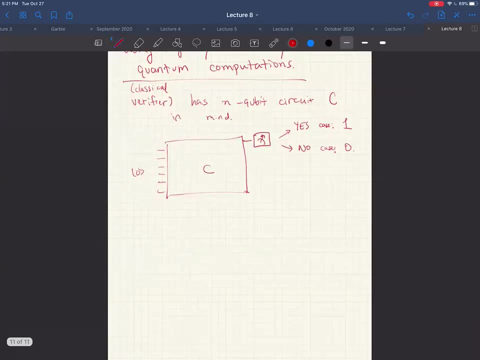 yes case. you know, let's say to, just to keep things simple, it accepts with probability one and in the no case it accepts with probability zero. so the verifier would like to just determine is it a yes case or a no case. but since it's classical, it has no way of of determining this on its own. so it's going to. 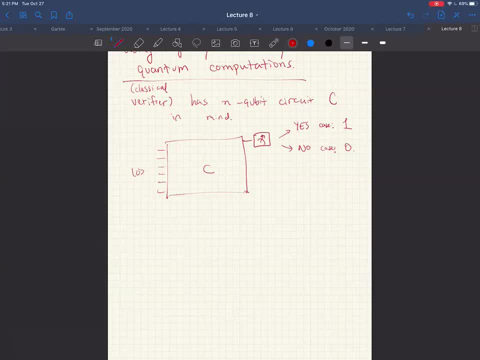 use the help of some quantum computers. but you know we're going to adopt like a very paranoid mindset. the classical verifier doesn't trust these quantum computers. you know what if maybe they're defective or maybe it's just like you know a scam or something? so instead the verifier 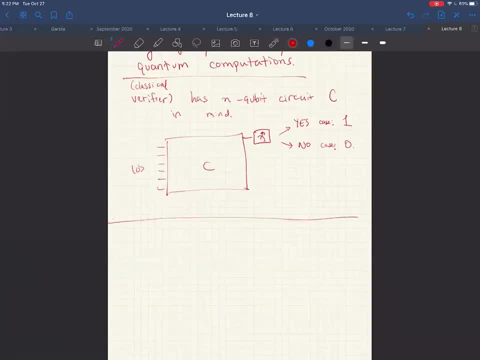 is going to interact, you know, run some interactive protocol with these quantum computers to to check for itself whether it's a yes case or a no case. so in this, the model that we're going to, the protocol that we're going to talk about, we're going to have two quantum computers that we're going to name Alice and Bob, for obvious. 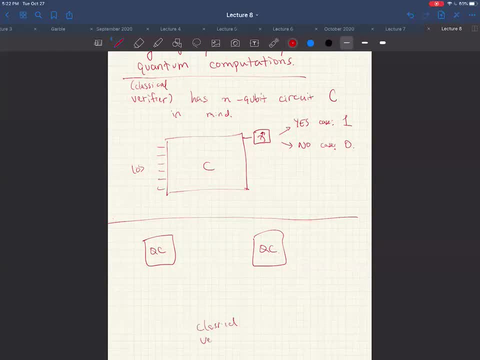 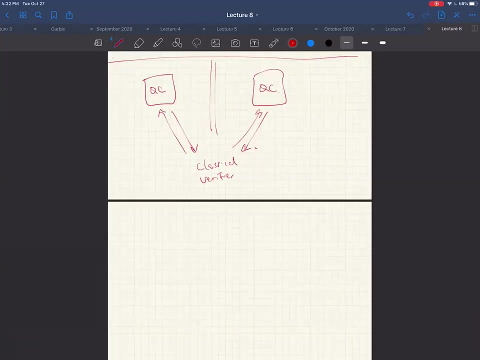 reasons, and the classical verifier is going to play games with these two quantum computers to determine yes or no. so that's the, the setup. you know, there's no communication between these two quantum computers and the protocol that we're going to design. we want it to satisfy the following properties: 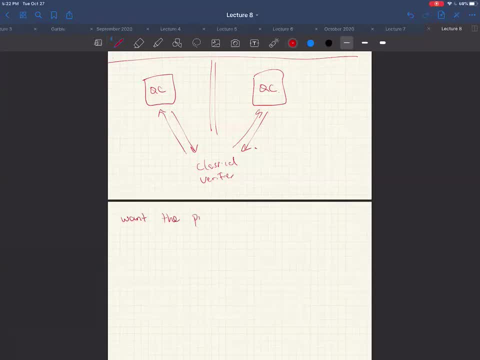 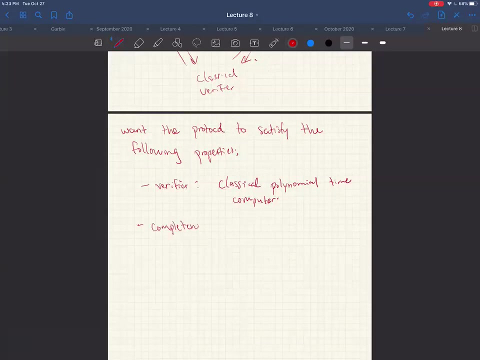 okay, so one property is that well, we would like the verifier to. we don't want to demand too much of it, so, verifier, it's a classical polynomial time computer, all right. so that's obvious. we want this protocol to satisfy a completeness property, meaning that suppose that the circuit c is a yes instance. 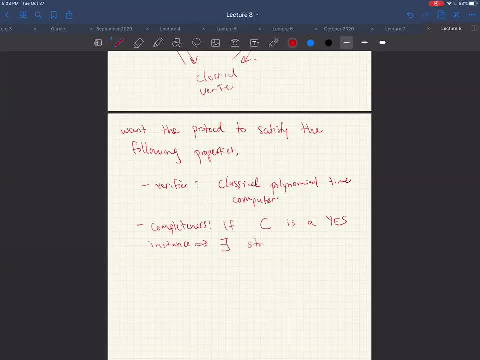 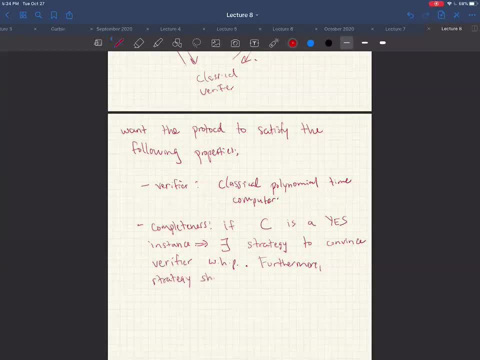 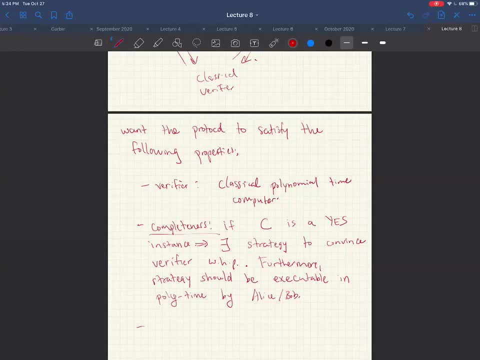 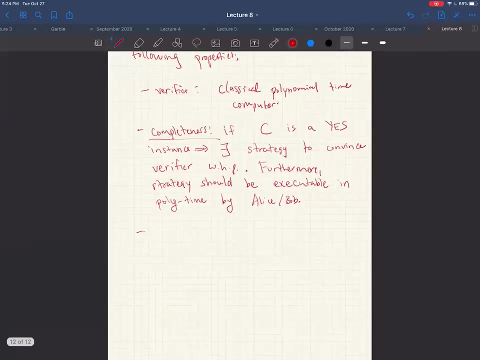 I mean, this is actually kind of important because you know we actually want to run this protocol in the real world. so if, if the quantum computers are behaving honestly, then then they should be able to carry out this protocol in a reasonable and rational way amount of time. And then, on the flip side, we want a soundness guarantee, which is that if C is a no, 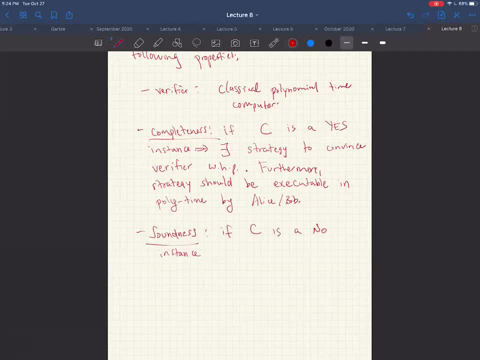 instance, then no matter what strategy Alice and Bob come up with, the verifier rejects with high probability. And here we can even say this should still be the case. even if Alice and Bob are allowed to do things that are very, very complicated, There's no limit on their power. I mean this. 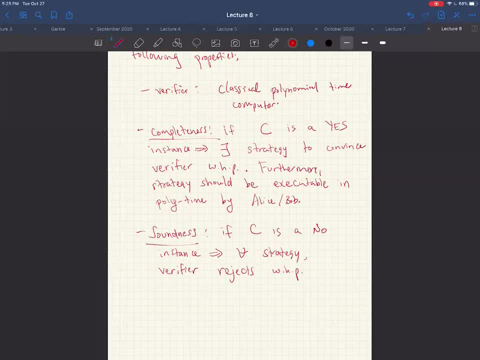 only strengthens our guarantee. No matter how powerful Alice and Bob are, they cannot convince us of a yes instance. Okay, So we want to design a protocol satisfying this, And if we had such a thing, then this would be a verifiable way of checking quantum computations, And the classical referee doesn't. 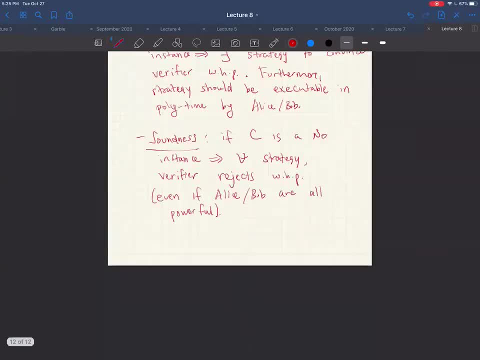 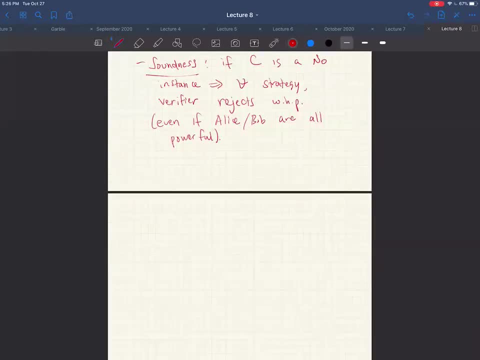 have to trust these quantum computers at all, but it can still get a guarantee, All right. So I hope that makes sense. In order to describe this protocol. I'm actually going to break this up into different steps. So first I'm not going to describe the full protocol, but sort 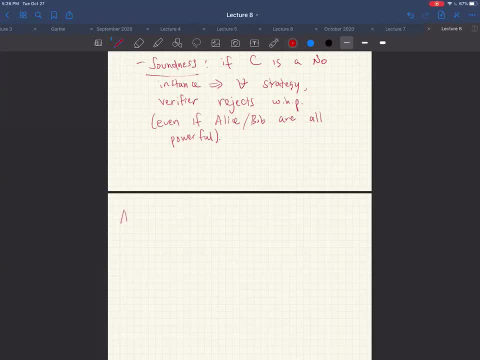 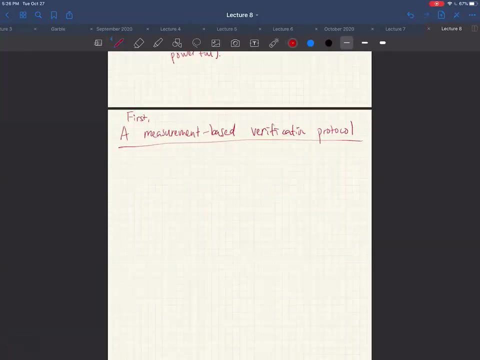 of a simplified setting. So I'm going to describe what's called a measurement-based measurement. Okay, So I'm going to describe what's called a measurement-based verification protocol. So here the setup is as follows: Like the classical verifier has access to a special quantum device. 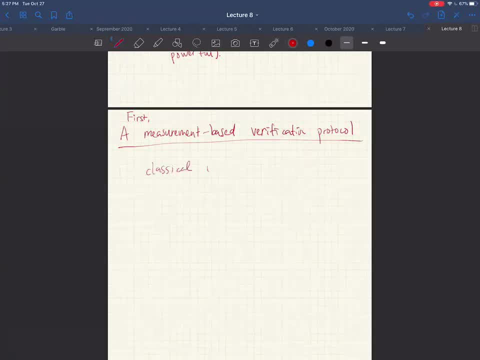 So the classical verifier has access to a special quantum device. So the classical verifier has access to a special quantum device. So the classical verifier has access to a special quantum device, That's it's called a measurement device. And this measurement device is going to be extremely simple. 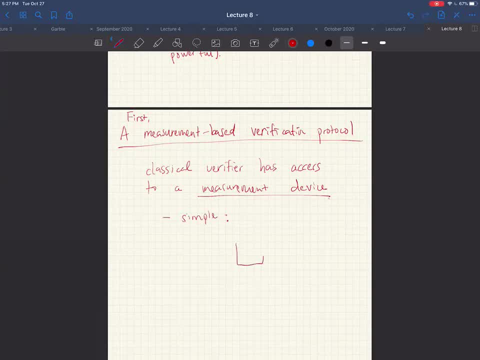 Because all it can do is you know it's a box, So I'm just going to call this measurement device M. It gets some state psi just comes from somewhere, And what the verifier tells the box to do is just measure in either each qubit separately, in either the x, z, or you know identity, which means you don't measure it. 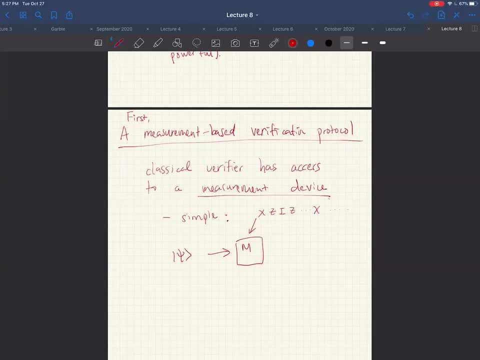 You know, just measure each of the qubits according to some basis, right, standard basis, or X basis, or don't measure. And this measurement device is supposed to do it And it returns a sequence of outcomes. So it's going to return A1, A2.. Up to You know. 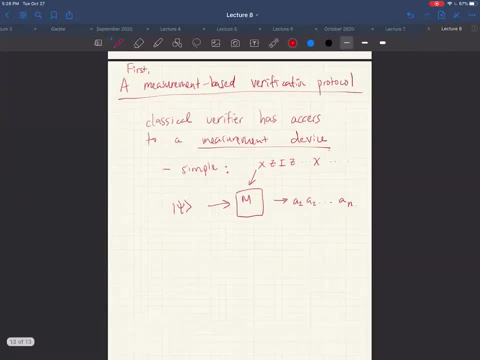 to a, n, how many ever qubits this state has? So and that's all the measurement device does. It's not capable of doing running a circuit or anything, So by itself cannot execute full quantum computations. It's really simple. 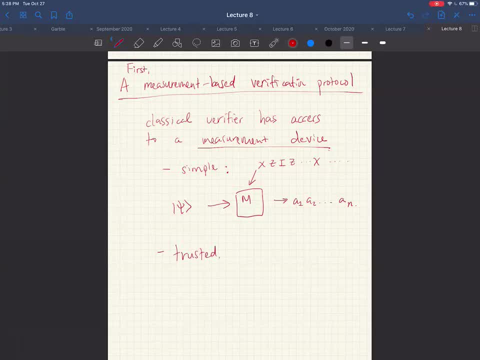 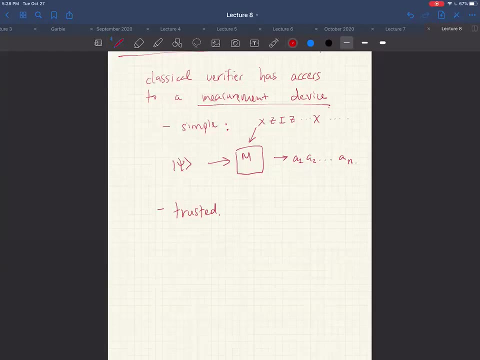 but the important thing is that it's trusted, Like when the classical verifier tells it to do this measurement, it's actually gonna do it in an honest way. So the claim is that in this model, the verifier can actually verify a quantum computations, and in a pretty straightforward way. 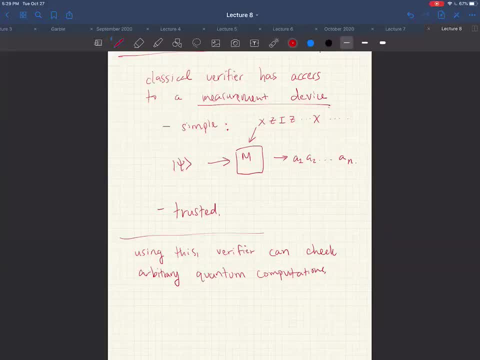 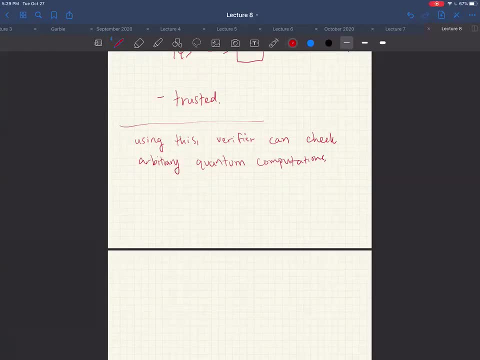 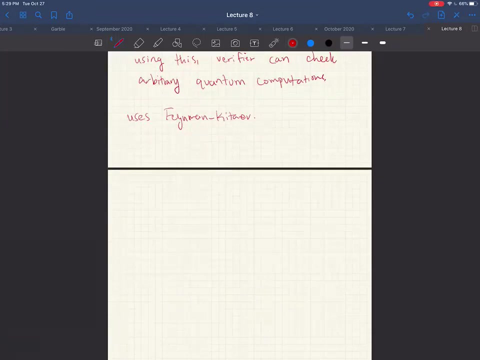 And this makes use of our beloved Feynman-Kataev transformation. So how does it work? Well, it actually uses a variant of it. So what's the variant? So it's going to be a. we saw that, given any quantum circuit, 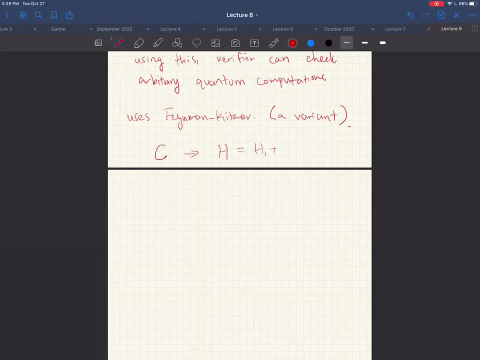 you can map it to a local Hamiltonian Right. so in this variant it's gonna map circuits to Hamiltonians, but this Hamiltonian is going to satisfy some different properties than before. So this Hamiltonian is going to be a triplet right. 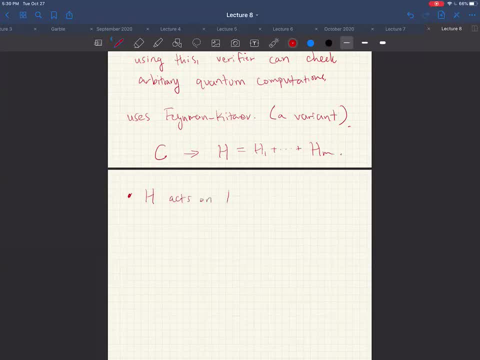 is going to act on. let's call it R qubits. So what's R? It's just going to be some polynomial in N. Each term of this Hamiltonian is going to have a very special form And it's going to be tensor products of projectors. 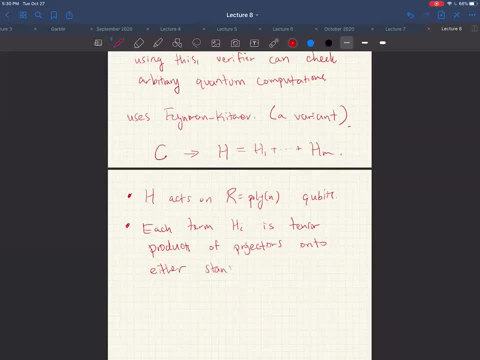 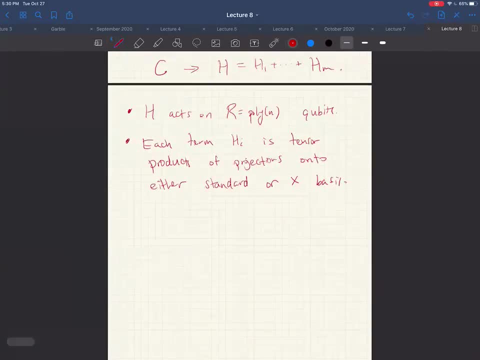 onto either standard basis states or X basis states. So you know, here's an example. So HI could look like zero zero applied to some qubit of X. So you know, here's an example. So H- I could look like zero zero. 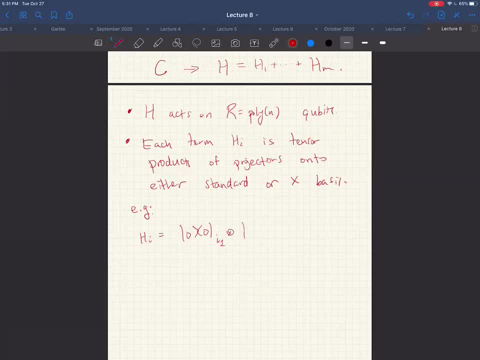 applied to some qubit of X, I1, tensor plus plus acting on qubit I2, and so forth up to minus minus on some qubit IK. So HI acts on qubits, you know index by I1 up to IK. 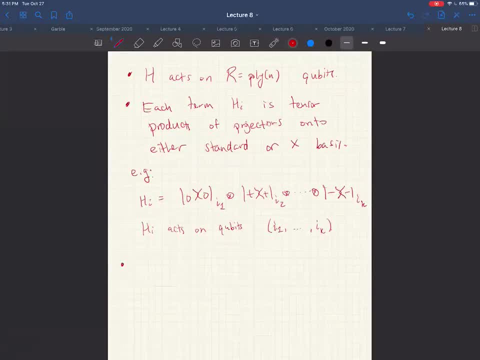 So pretty simple form. Another thing is that this is not going to be a local Hamiltonian, So like the number of qubits that each term exon could be up to R, Okay, but we're not going to be so worried about that. 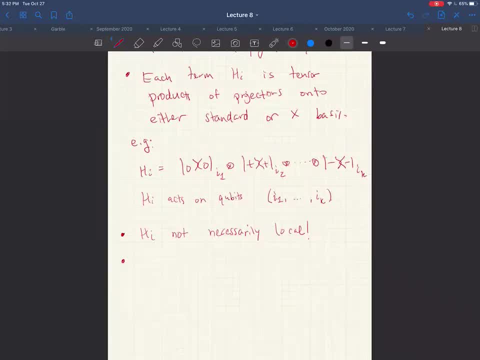 Like it's fine that it's not a local Hamiltonian. Another thing is that there could be an exponential number of terms. In fact there generally will be. Despite having so many terms, they're actually efficiently computable because, given any index, i, the verifier, can compute any given term. 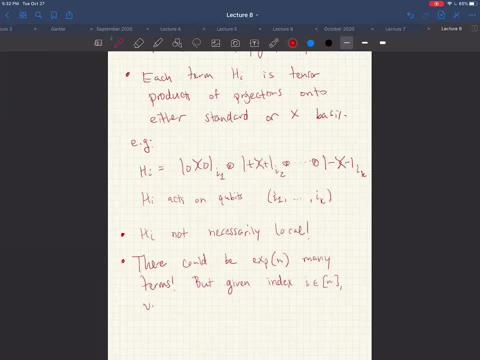 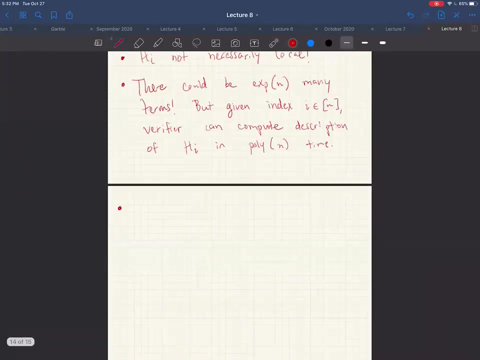 All right, so there's a lot of terms, but each of those terms are easily computable. Okay, so just a couple more properties, So we start with a number of terms. Okay so, just a couple more properties, So we start with a number of terms. 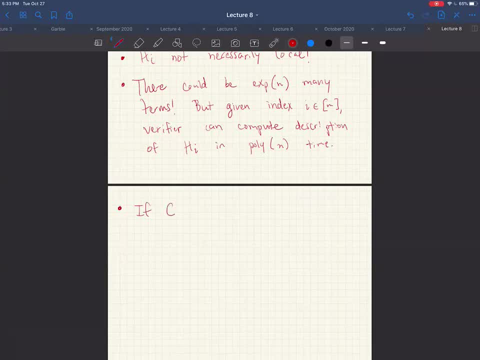 So we started from a circuit. We created this local Hamiltonian. What's the relationship between the two? If c is a yes instance, then there exists a ground state such that it has energy zero, And if c is a no instance, then for all states the energy is actually going to be very high. 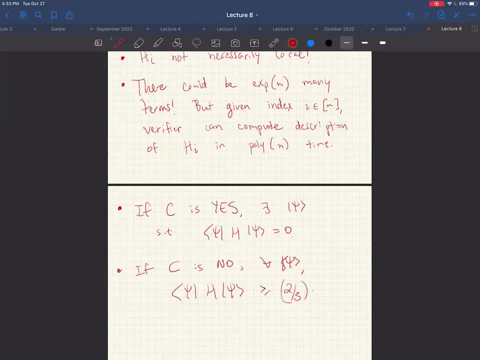 In fact, it's going to be something like two-thirds times m. In fact, it's going to be something like two-thirds times m. All right, so there's actually a huge gap between these two cases, And this is something we didn't even see with the Feynman-Kataev construction. 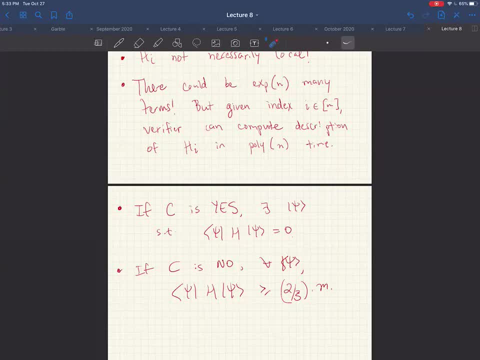 Like the Feynman-Kataev construction, had like a very, very small gap, some inverse polynomial gap between yes and no. Here we actually have some ginormous gap And we're able to obtain this precisely because we don't have a local Hamiltonian and we have exponentially many terms. 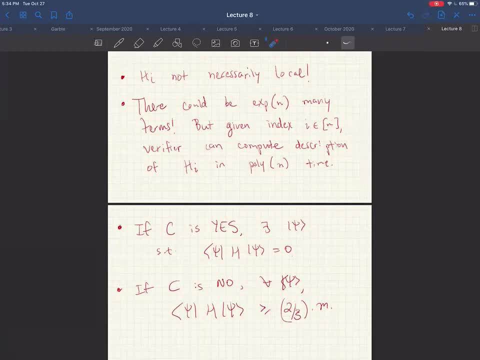 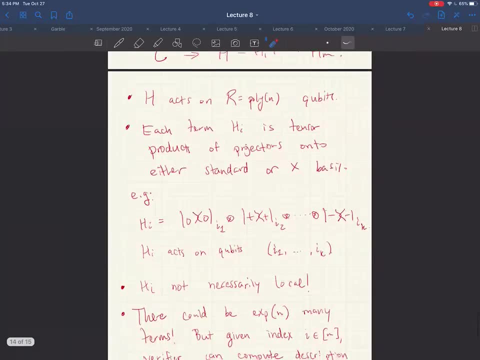 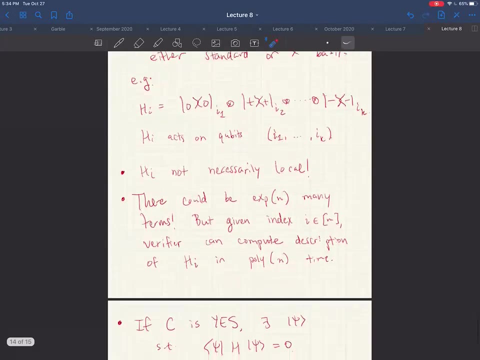 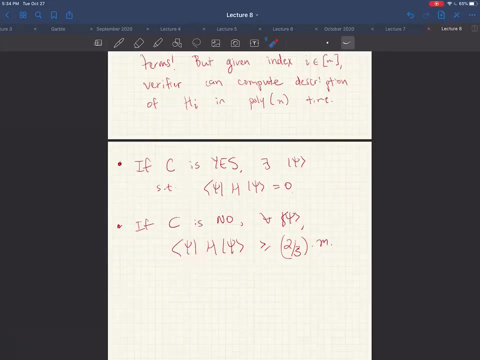 This is something that we can do. Does this make sense, Like what these properties that are spelled out here? All right, so it's not a local Hamiltonian, It's just some huge Hamiltonian, But it captures whether c Is a yes instance or a no instance. 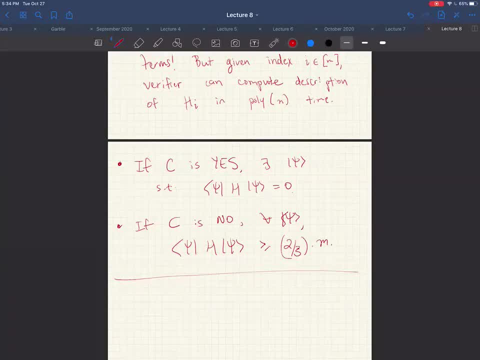 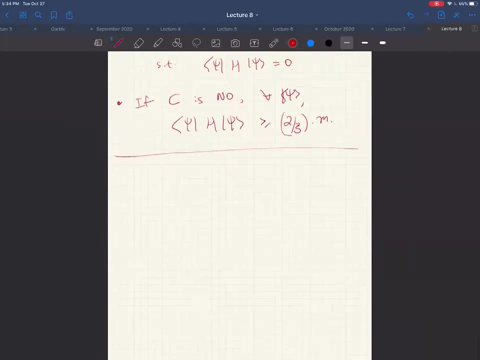 When you say that it's not local, do you mean that like a single term can like act on all the q bits? Exactly, yeah, Okay. so with this Hamiltonian in mind, the verification protocol is going to be very simple. So the verifier is going to do: just pick a random term. i. 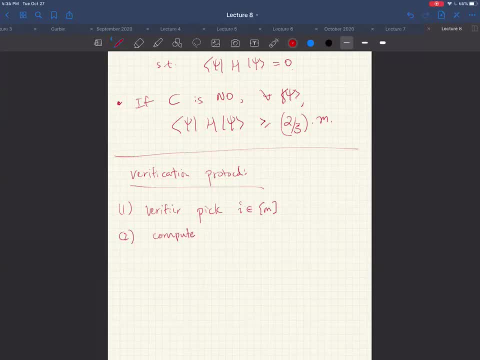 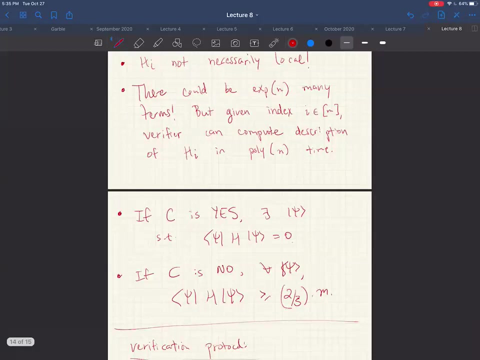 And then it's going to compute the description of this term, Which I promised you could be done efficiently, given the description of the circuit c. And what do we know about this term? HI? Well, it's this like tensor product of measurements in the X or Z basis, right? 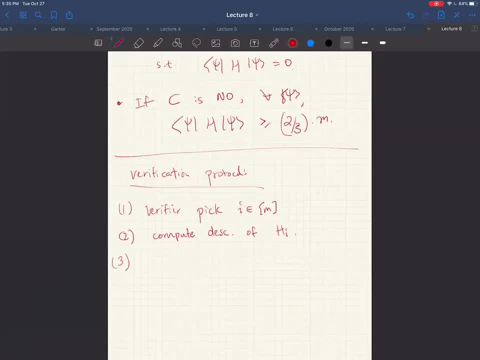 So the verifier is going to compute a string of measurement commands. All right, so sorry, just a second. So like for this example that I wrote here, like there's zero, zero, plus, plus all the way to minus, minus. 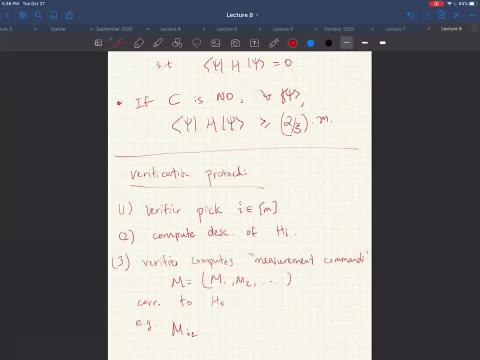 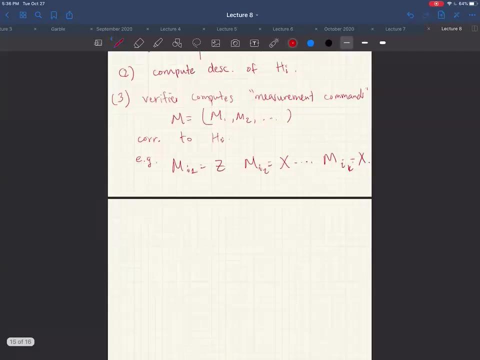 then this one would be measuring the Z basis, i2 would be measuring the X basis, And the last one would be measuring the X basis. So it computes the measurement commands and then what the measurement device is supposed to receive from the quantum computer, like this untrusted quantum computer. 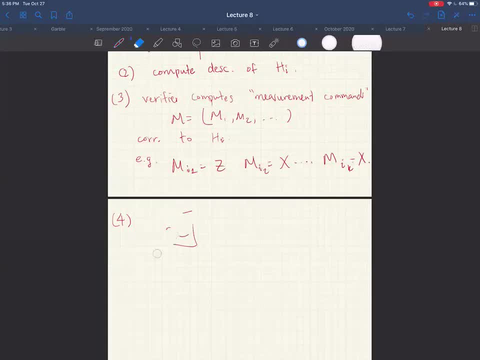 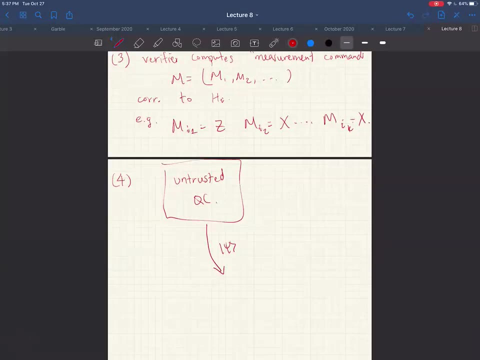 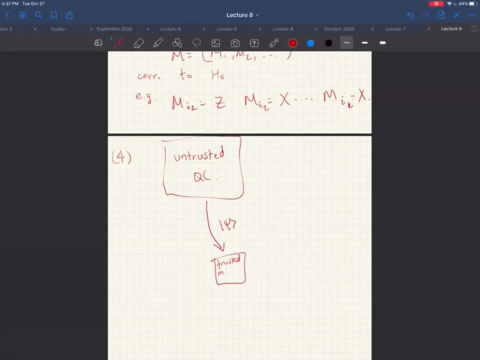 So here's the QC. it's untrusted, It's supposed to send down, supposedly, the ground state of this local Hamiltonian to this trusted measurement device And the verifier, you know, tells it to measure the sequence of measurements, M and outcomes. 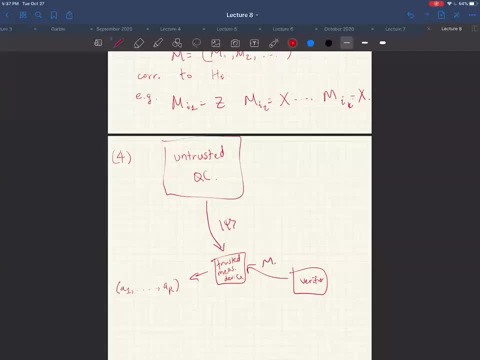 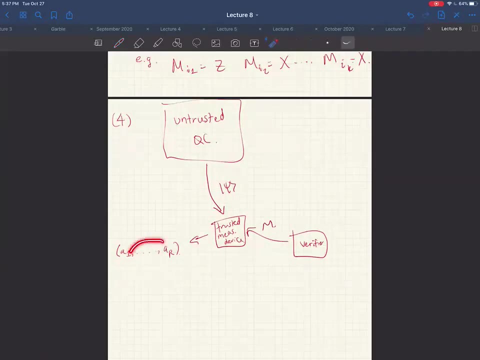 a sequence of outcomes, A1 up to AR, which is like measuring this psi, each qubit of psi, and you know, according to the right basis, right, And then based on the outcomes, the verifier is going to be able to tell whether 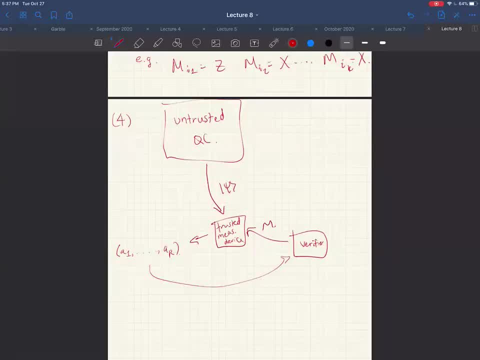 like get an estimate of the energy. This will tell Amazon M we're going to get all this electricity out of this piece of that low Graphene fase, Or would be able toardon in not getting the low versa and they could just run without it. 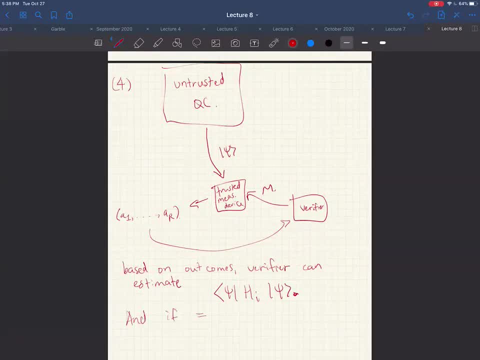 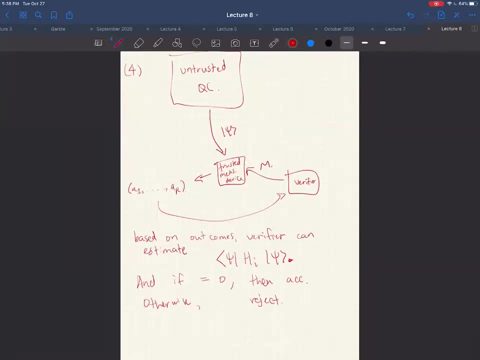 And then, basically, if this is equal to B, knows that I'm in. if this is equal to B, to zero, then accept, Otherwise reject. So right, like if it. you know, if, according to this term, it has low energy, then you're going to say: well, I think it's very likely that this 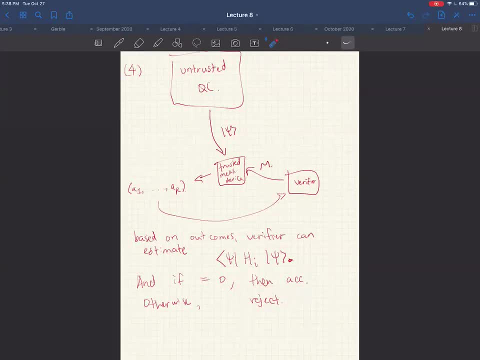 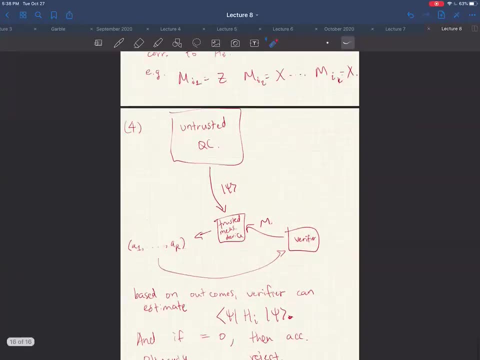 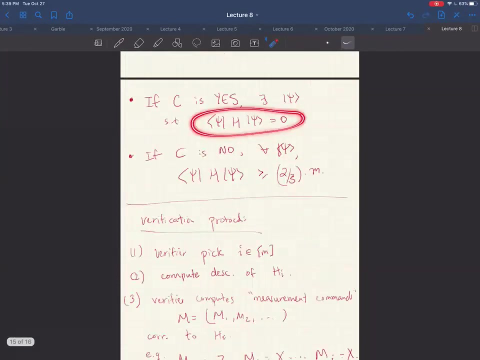 is a yes instance. On the other hand, if it has energy that's, you know, non-zero, then I think it's going to be a no instance And this is going to be a like, actually a very good protocol, because if it really was a yes instance, then what this untrusted quantum computer could do? 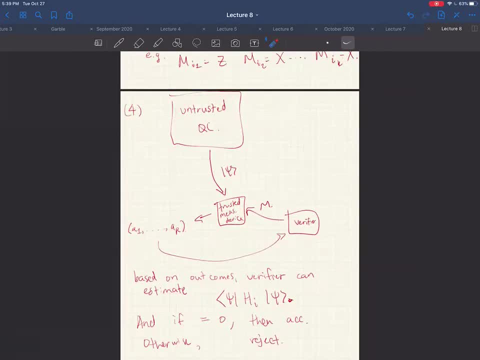 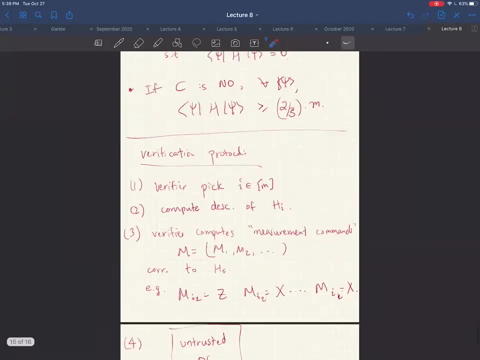 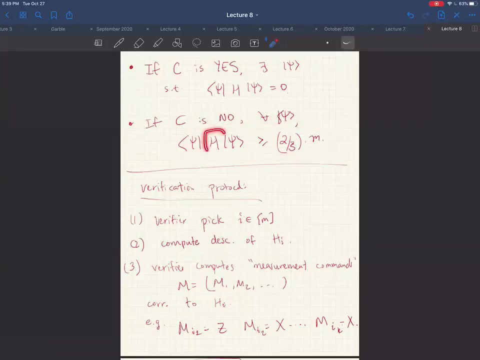 is prepare this zero energy ground state And then the verifier will you know all the all the checks will pass. But in the no case, what this energy tells us is that if you sample a term at random and there's M terms, the energy is going to be on average. 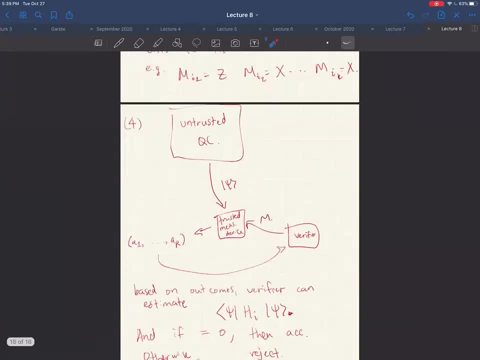 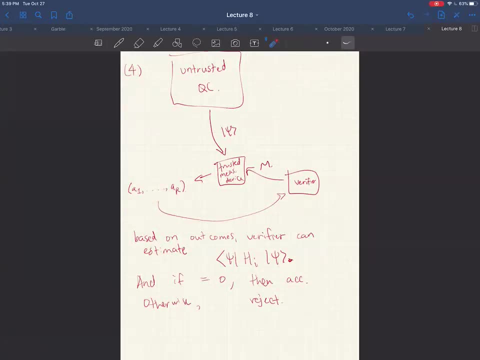 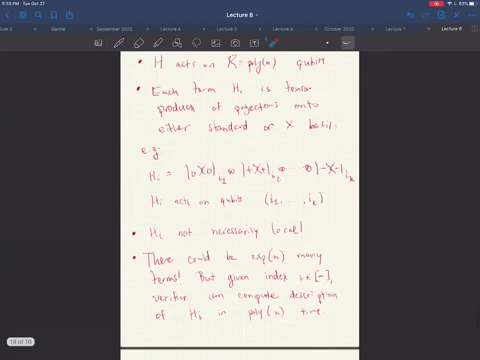 at least two thirds. So the measurement results are going to reflect that. How do you exactly approximate the, the, the, the, the A, the measurement? Okay, good, So if let's you know, take a look at this example, this HI. 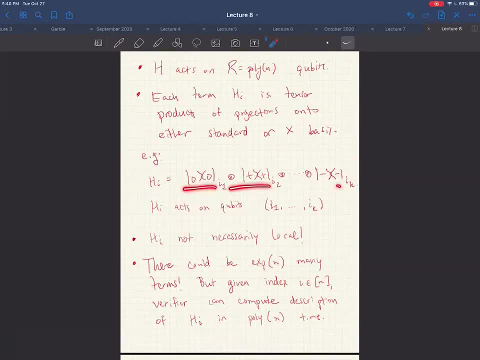 Basically think of this as telling which measurement results are forbidden. So you know. so let's say we, we picked this HI and we look at the qubit, the measurement outcomes for qubit, and we look at the measurement outcomes for qubit and we look at the measurement. 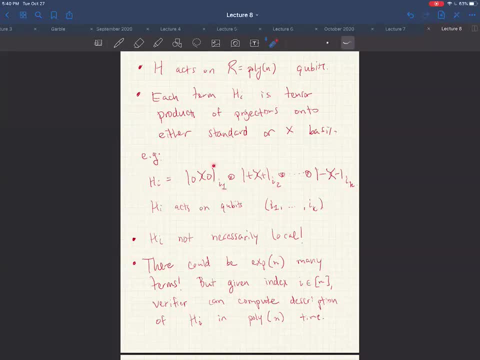 får firsts. So say qubit's I1, I2 up to IK. you can use osm lagd on q, regawqt Vi. you can look at the measurement 저�ch solid. if any of them match this, then we know that the energy is going to be non-zero. 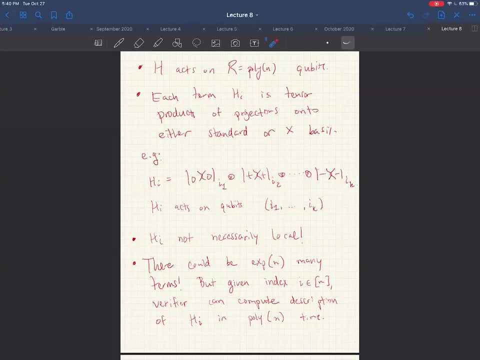 No, zero answer. As you're reading this, I've left you, so in this case we would reject. but if we get measurement outcomes that do not match any of this- like let's say, for qubit I1, we get a measurement outcome one- then we're. 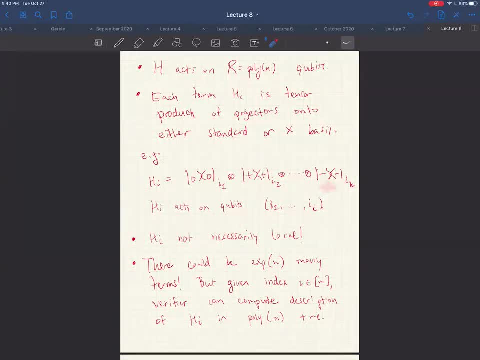 happy. We get minus, then we're happy. if we get plus, then we're happy. changes results, And then we accept. It seems like one could definitely create Hamiltonians, though, where the variance in the energy of any one term acting on the ground state is wild. 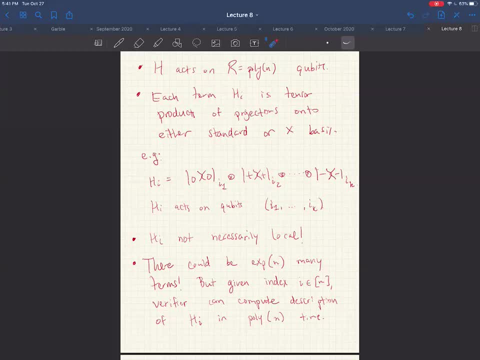 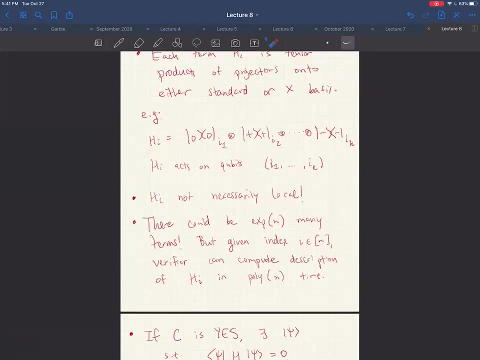 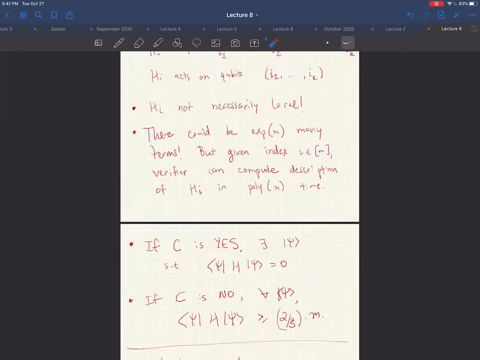 But the ground state energy is still zero. Well, if the ground state energy is zero? well, here one thing is that all of these terms are positive, semi-definite. So if this ground state energy is zero, then we actually know 100% of the time, the correct ground state will always have energy zero with respect to all of the terms. 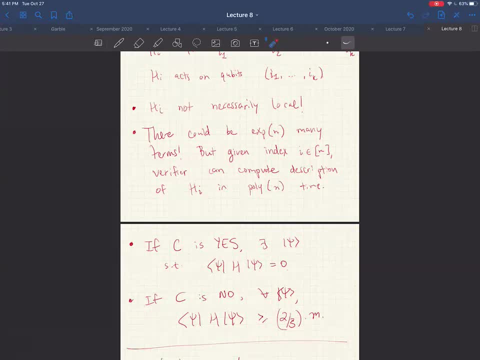 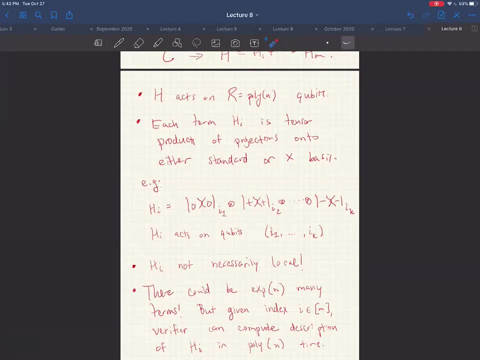 Ah, okay, That'll do it. Yeah, So we are using that fact. Don't you need to match all the terms for it to be non-zero. If we scroll up a bit Right here, If any one of these terms, like if you get a state with zero as in the no, no, if you get a state with one in the i1th qubit, then wouldn't that just change everything to zero? 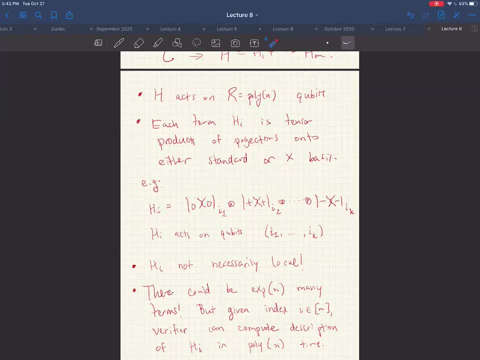 Oh, yes, Yes, Sorry, You're right. I think I said that wrong. Yeah, As long as you. Oh, I see. Okay, Let me put it this way: In order to get a non-zero energy, you have to match all of these. 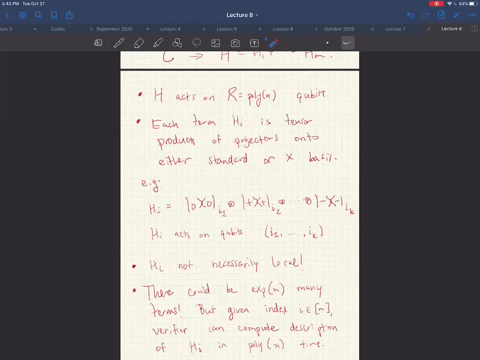 That's, that should be the right thing. right, Right, Okay, Yeah, As long as you do not match any one of them. it's, it's like. what is it called? Yeah, Yeah, Yeah, Yeah Yeah. 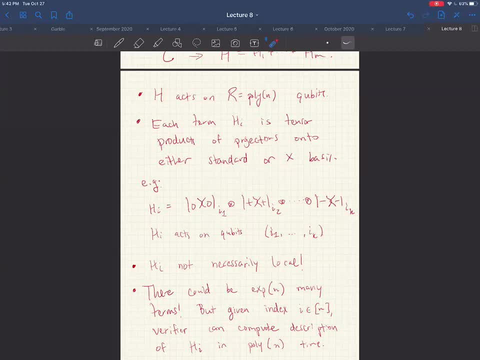 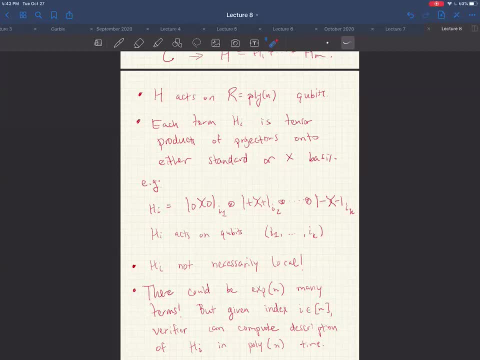 Right, Okay, Yeah, As long as you do not match any one of them. It's, it's like: What is it called The disjunction you know you have, or if you do not match any one of them? 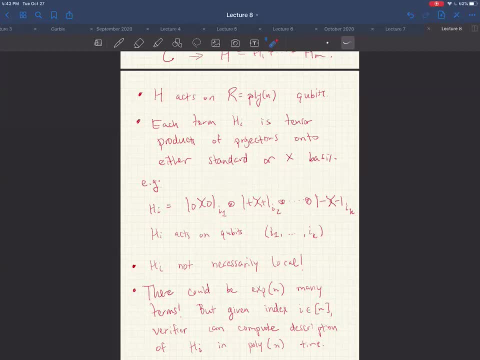 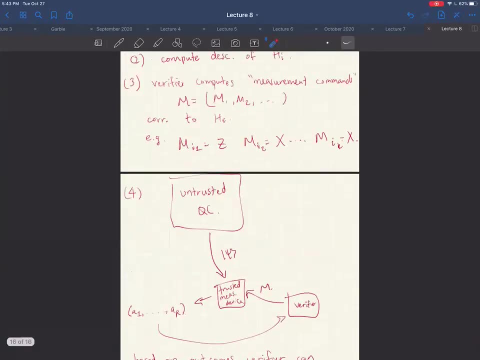 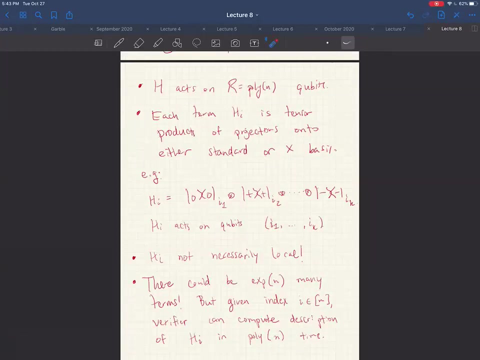 then you're going to get zero energy. Okay, yeah, Good, Good catch. But isn't it like sort of counterintuitive? Because, like Yeah, This contradicts the thinking of the yes case is an exists case and the no case is a for all case, because basically, you're now saying that there is only one state who can get this term to be non-Z? Z, zero. 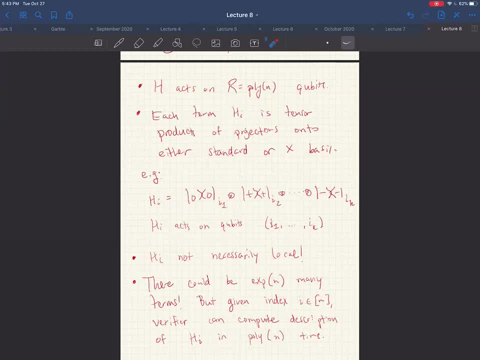 But any other state which follows this form will be a Z, Z, zero, zero, zero. Do you understand what's confusing me? Yeah, I see. Let me make sure I have this right. I might have simplified this a little too much. 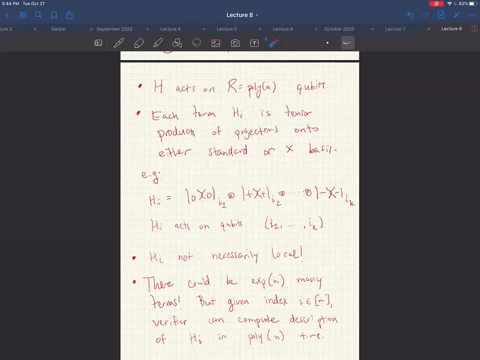 Like when you explained it the first time, I simply thought that, okay, no, we are simply measuring different qubits each time on like n copies of this state, And then what you said previously: It works, I think. 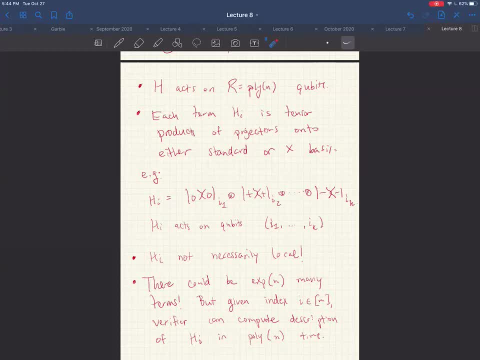 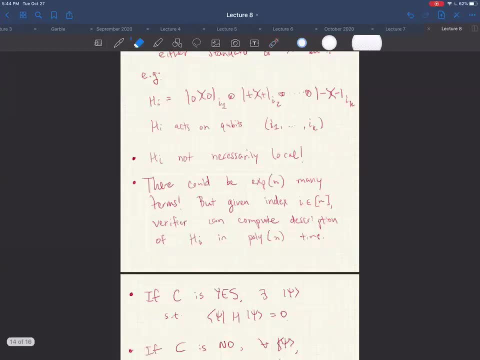 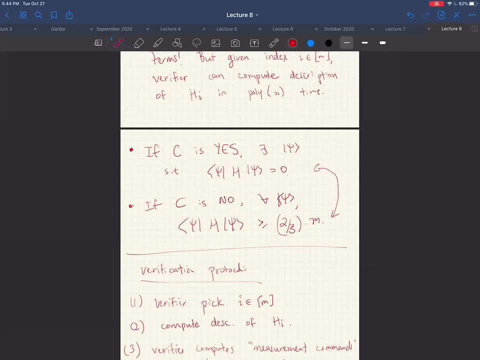 Yeah, I think you know what, maybe I might have switched my yes like. yeah, I might have switched these two cases. I mean, you can also like choose the HIs so that only one state will give you a yes state, right? 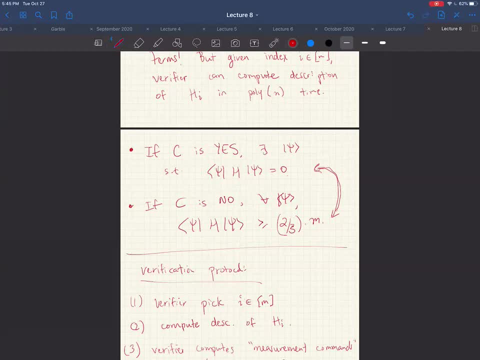 Because if One HI is not Actually no, Oh wait, no, that doesn't make sense. Yeah, I'll have to check this, but I think the, If there's an issue, it would be resolved by switching the yes and no cases. 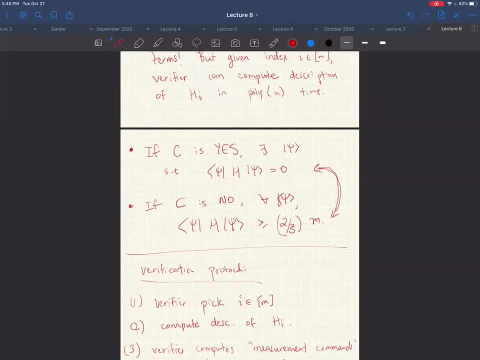 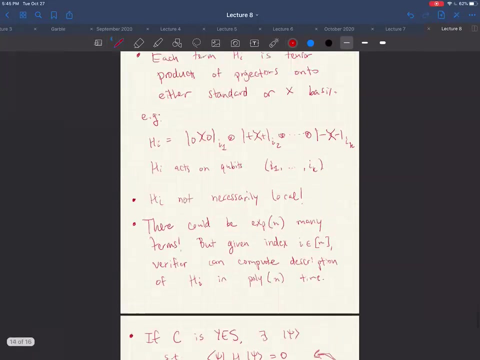 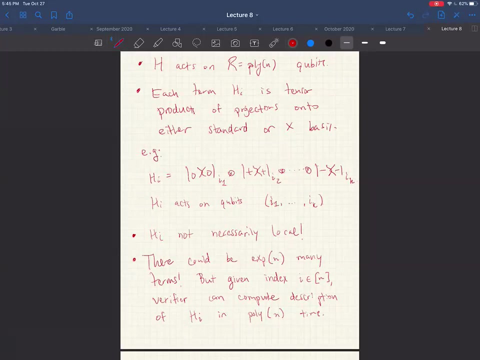 Like in the yes case there's a state with very high energy And in the no case, like all the energies are, like all states have pretty low energy. But I will have to check that, Let's see. But actually I'm not sure. like you know, for example with 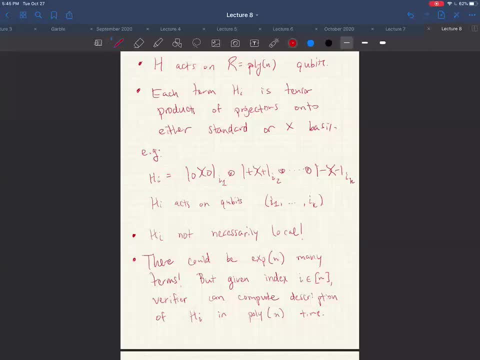 Just to go back to the classical Like. what's the classical analogy? Like, three set Like. each of your clauses are forbidding exactly one assignment to the Like. it's saying there's one Like setting of the three variables in each clause that are forbidden. 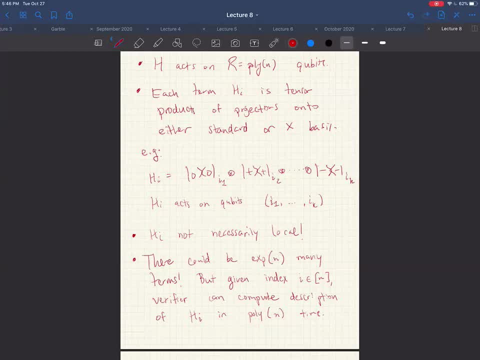 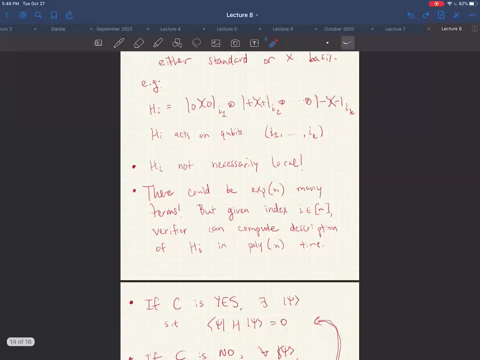 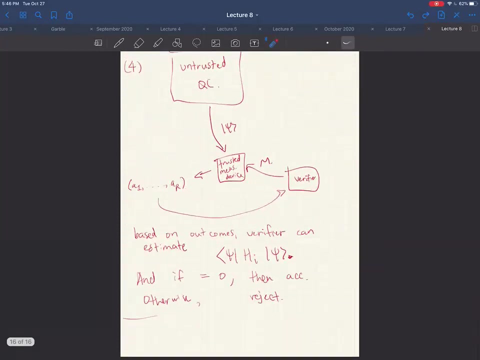 So that would be kind of the analog. here We're saying that there's one setting to those qubits that are forbidden. So I think maybe this could be correct, But I'll have to double check, Okay. Okay, now it actually makes more sense. 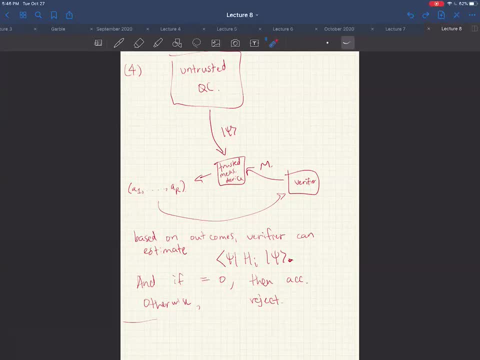 Because A and B do not know which H I chose, And so I gave them basically a random C and F, If I'm thinking about it in classical terms, And their assignment needs to satisfy it. Oh yeah, So that's a good point. 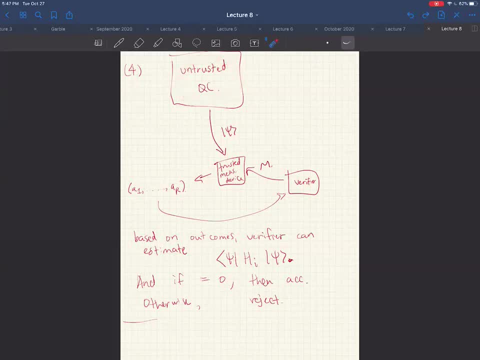 So this untrusted quantum computer has no idea what term you're checking, You're just telling, Like the verifier at the beginning says: Hey, quantum computer generate me the supposed ground state. The quantum computer generates it, sends it over. 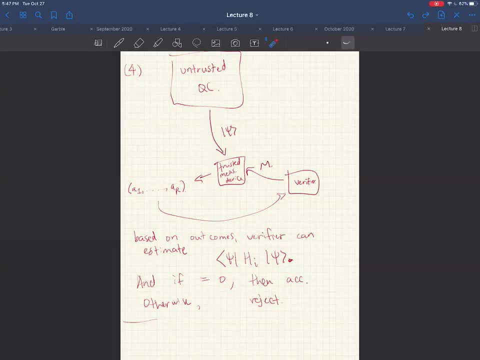 And then the verifier will choose a random term to check, So the state cannot depend on the term you're checking. If it did, then actually that would be really bad. Okay, great questions, though, Like any other questions about this measurement-based verification. 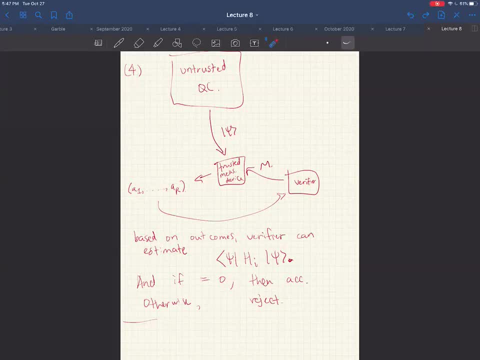 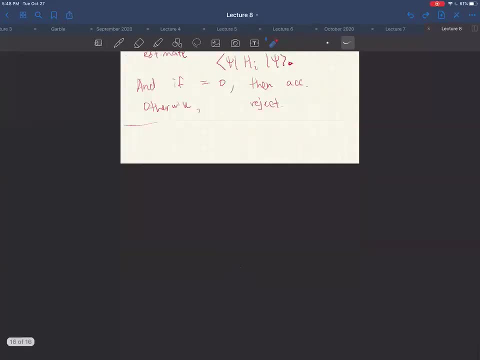 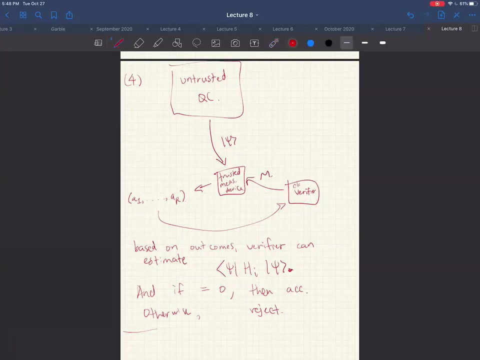 Okay, Okay. So this is pretty cool, But this is like not what we wanted, Like the verifier still has. You know, in order to do this, the verifier needs this trusted measurement device. Okay, it's a simple thing. 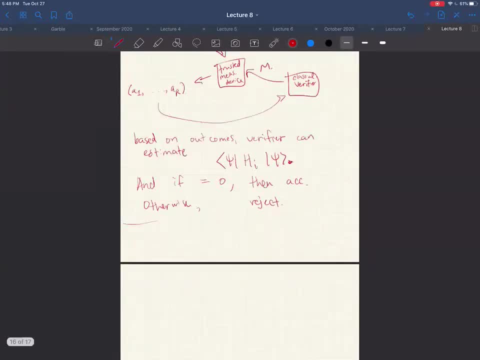 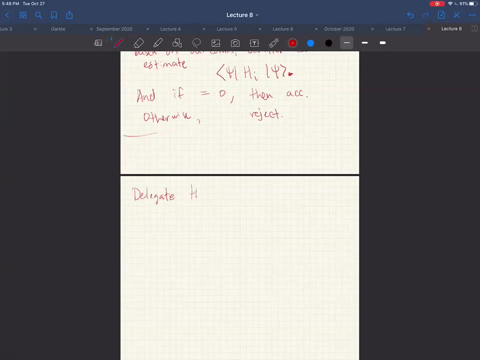 But it's still some extra assumption, And it would be nice to get rid of the need for this trusted measurement device, And so this is where we go back to this two-player setting. Okay, The idea is to delegate the measurement to untrusted provers. 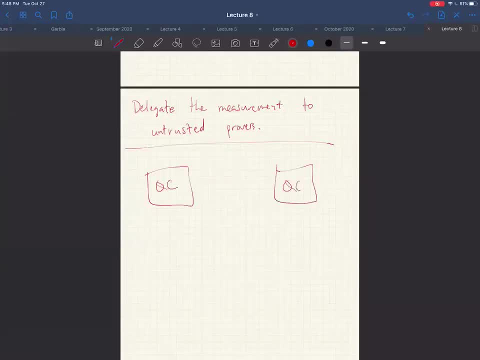 Okay, so we're gonna go back to this two prover model. So we have two untrusted quantum computers and we have the classical verifier, And now we can only have classical communication between the quantum computers. And the key idea is we're going to play these rigidity games. 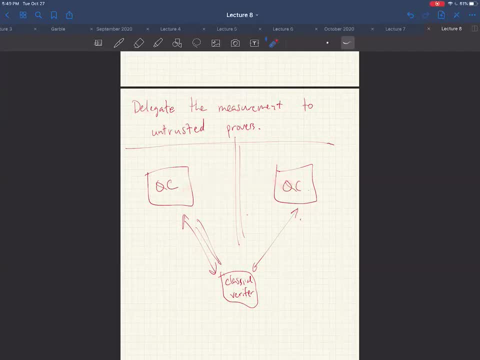 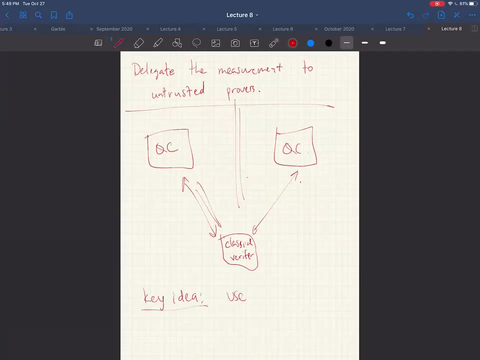 like the magic square game between these two quantum computers, to basically force to convert one of these quantum computers to become the trusted measurement device. Wait, so you are allowing the quantum computers to convert To communicate. Is that what you said? No, no, no, they communicate with the verifier. 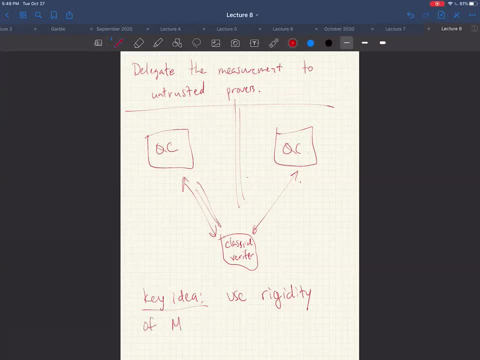 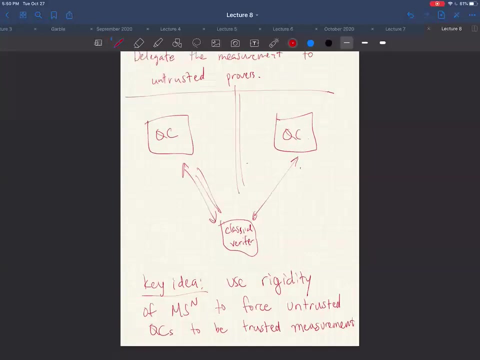 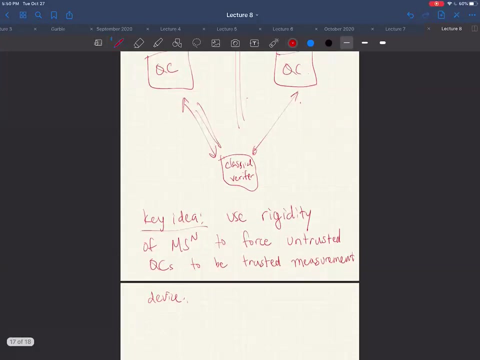 I see I didn't hear you. This should make intuitive sense. like our rigidity statements are so powerful, Just by observing how often they went a game, we know exactly what measurements and what states they're using And we're gonna leverage that to simulate. 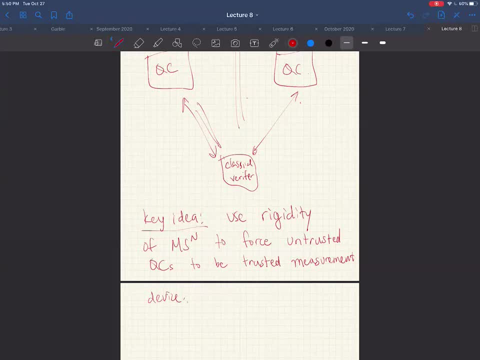 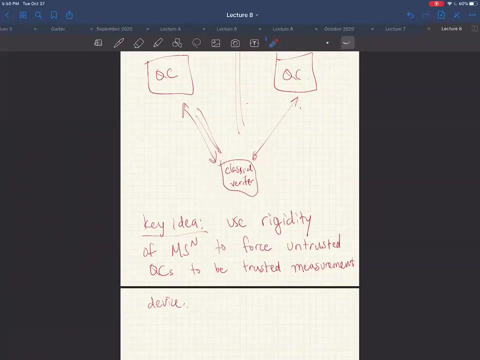 this verification protocol that I just described So Right. The first step is this classical verifier can play this repeated magic square game And you know, let's say that the two provers, the two quantum computers, win with very, very high probability. 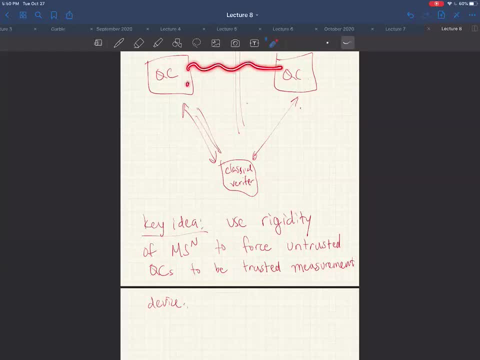 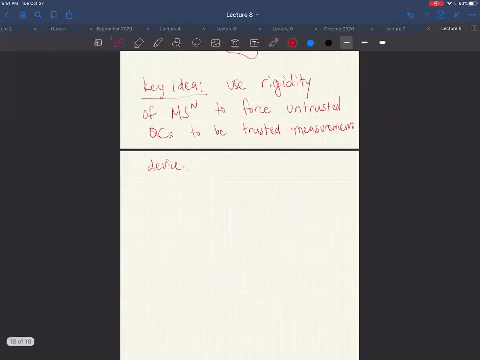 Let's say you knew that. Then this guarantees us they must be sharing many EPR pairs And in particular, this quantum computer is going to be making these poly measurements on each of those EPR pairs separately. So Let's see, OK. 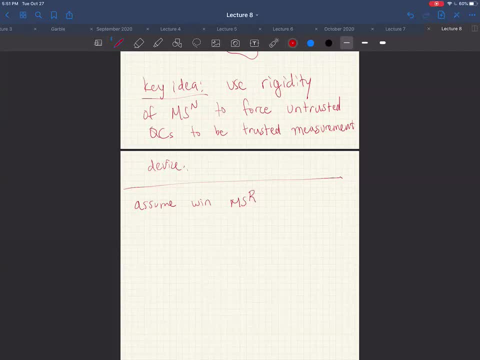 So I'm going to just say the number of games that we're playing is R, just to connect it to this verification protocol we just saw. Let's assume that they win with probability very, very close to one Right. Then, by the rigidity thing, this implies that Alice and Bob share 2R. 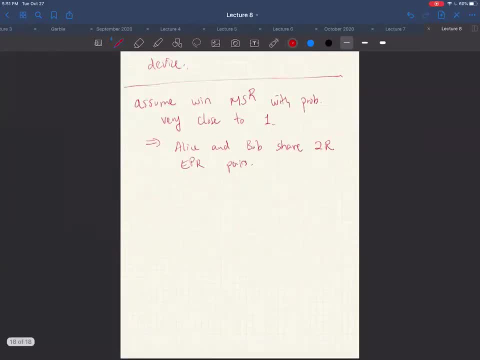 EPR pairs: right, Two EPR pairs for each of the separate games. So let's organize the EPR pairs in the following way: So I'm going to draw, So you know, here's Alice, here's Bob. So here's a pair, for instance one. 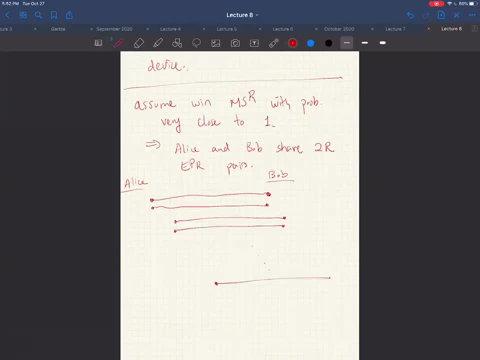 Here's a pair, for instance, two, so on. And you know, just to make things simple, I'm going to always ignore what Bob's doing on the first EPR pair, like we don't really care. So we're just going to ignore this. 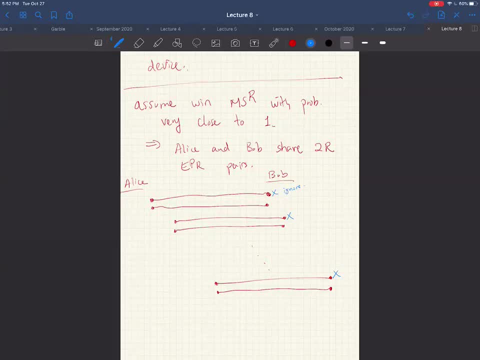 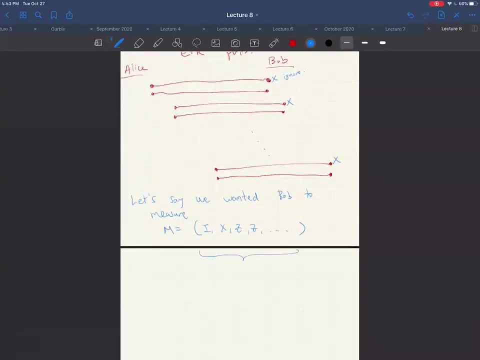 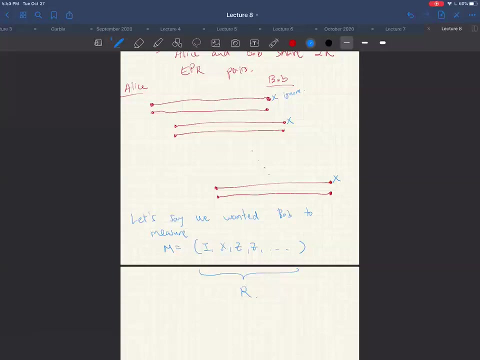 So, So how can we turn Bob into this trusted like, how can we make Bob simulate this trusted measurement device? So So, So let's say we had a string of measurement commands that is of length R And we wanted to say: for the first qubit measure, I, for the second qubit measure in the X basis, for the third qubit measure in the Z basis, and so on, 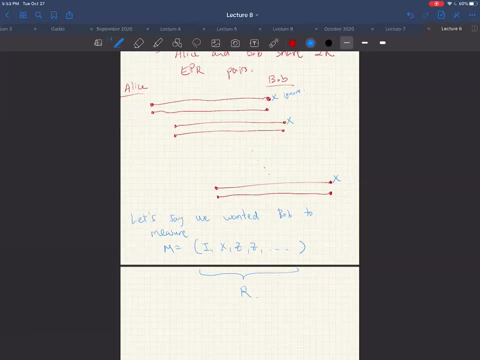 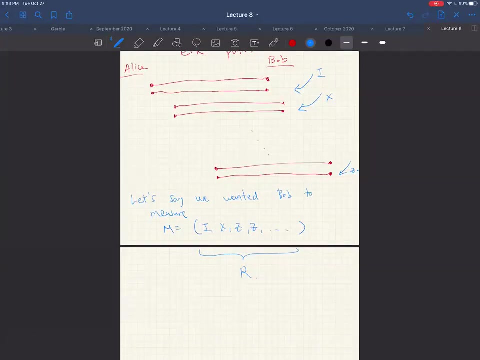 Right. And so, Diagrammatically, what we want him to do is measure this in I, this in X, and then you know the last one, and you know say to say Z. Well, we can simulate that by embedding those, these measurement commands inside the magic square game. So, 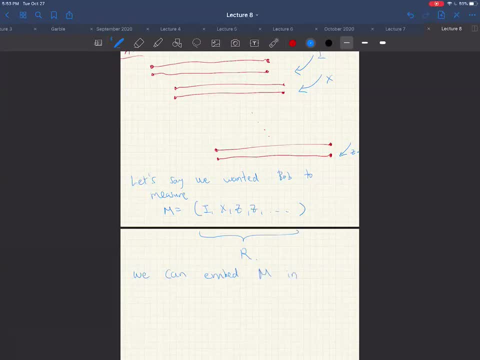 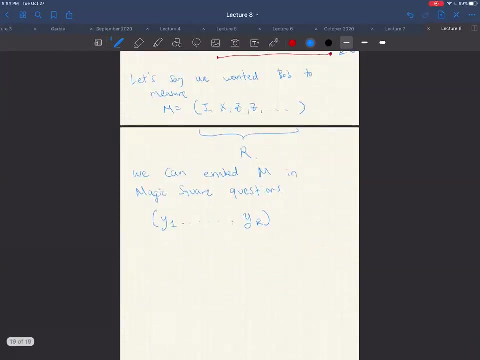 Right? So in the magic square game, Bob receives a sequence of questions Y1 up to YR. What are these Ys? They're supposed to be different cells of the magic square game. right So the YJs, Right? So in the magic square game, Bob receives a sequence of questions Y1 up to YR. What are these Ys? They're supposed to be different cells of the magic square game, right? So the YJs. 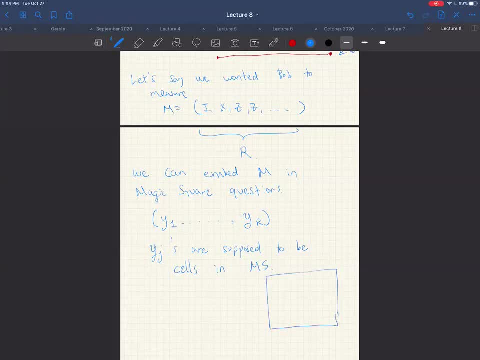 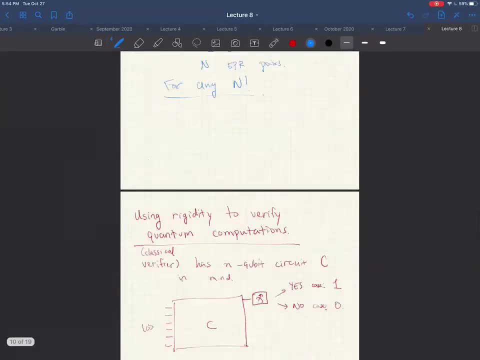 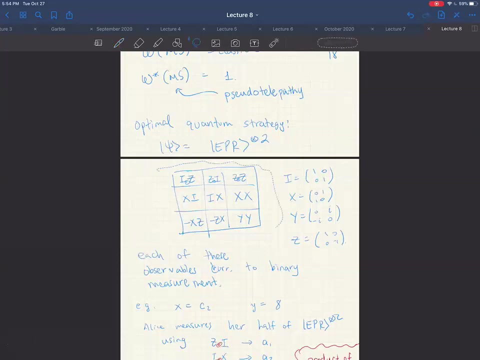 And let's sort of recall like what the canonical textbook strategy is supposed to look like, And I'm going to copy it really quick, Up up, up. Right, It was this, this thing here, So I'm just going to copy it. 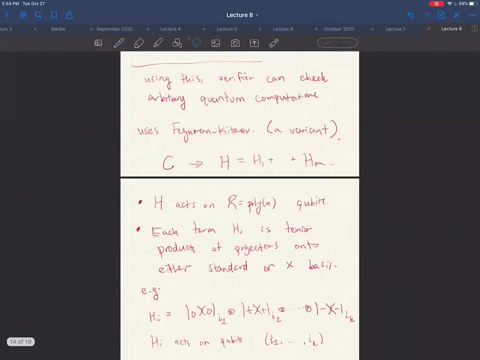 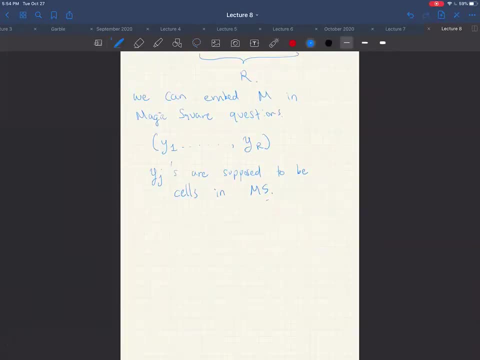 Okay, cool. So if I wanted to embed it, then I'm going to focus on these two special questions. cells one and five, Like those, correspond to measuring the second qubit in the magic square game. Okay, So for these two different questions, how would I measure the second qubit in Y? 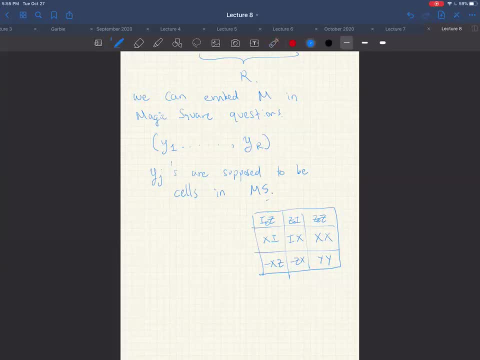 So I would measure the second qubit in Z or the second qubit in X. So let's say like, just as an example, let's say M was yeah, like like I, X, Z, so on. Then we can embed this into a magic square question by saying: I well, I'll just send them a dummy symbol, because I'm just telling Bob, like I don't really care. 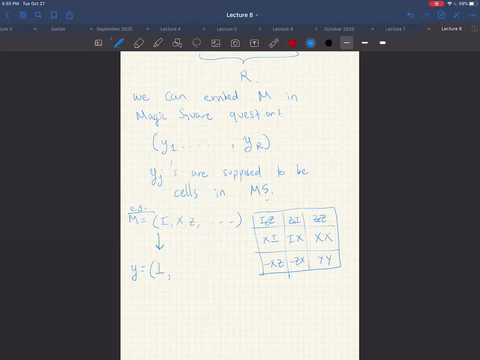 And then I just sort of get the first one Right, And then for x, I will send him cell number 5. And z, I will send him cell number 1, and so forth. So when Bob sees this, he thinks he's playing the magic square game. 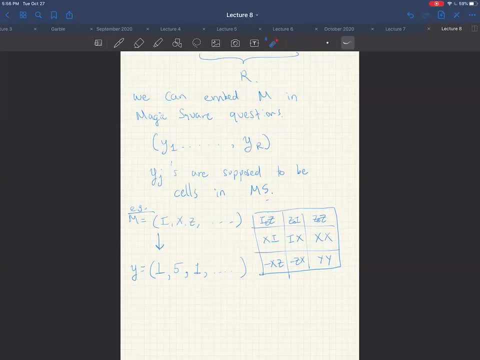 And since he's supposed to be winning with high probability, he has to be doing the honest thing. So, for the second instance, he has to measure his two qubits using ix, And for the third instance, he has to be measuring iz right. 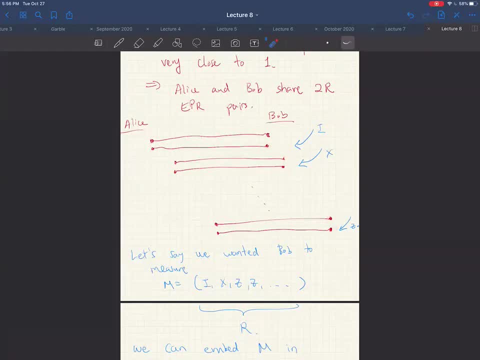 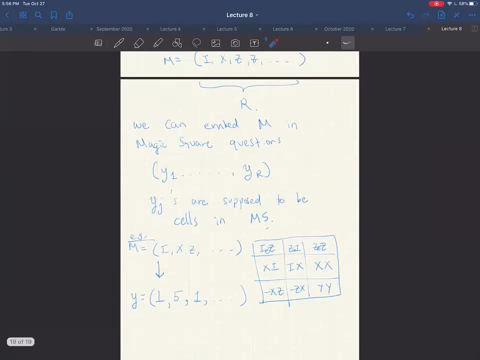 So on these EPR pairs, he's going to be doing those measurements And we know he's doing them. Why do you have that dummy? Oh I'm sorry. I'm sorry, You go, You go, OK. Why do you have that dummy? 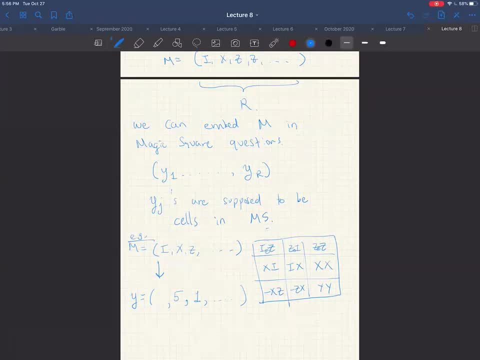 Oh, actually, basically I'm going to put a random question, so I'm going to put a wildcard. It doesn't matter, because we don't care what he's going to do in that coordinate. You just pick a random cell. 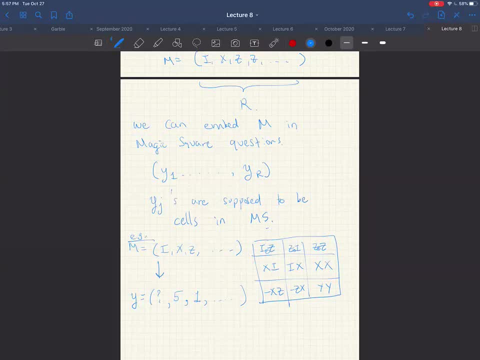 Just choose one at random. He'll do whatever measurement he does there, but we'll just see more of the answer. Is there a reason why we don't care about the specific coordinate? Oh, because your measurement command that you use, Your measurement command that you want, is ixz. 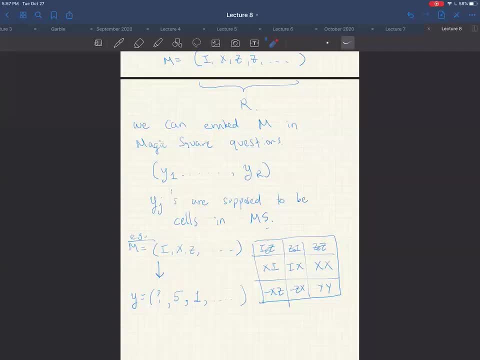 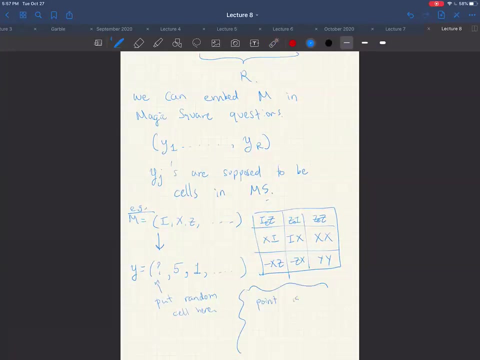 So i means like, i just means I don't care what the measurement result is, Oh, OK. yeah, that was basically my question too, So yeah, so the point is OK. So I'm going to say: Bob thinks we're playing magic square. 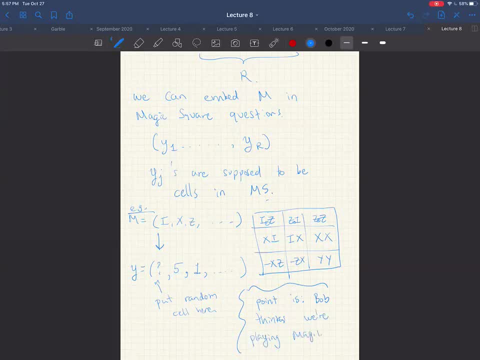 I don't think it would matter. but could Bob kind of figure out that he's not playing magic square because of the distribution of you know, if we're repeatedly using the top left square and the middle square, Yeah, So Bob will kind of realize that's what we're doing. 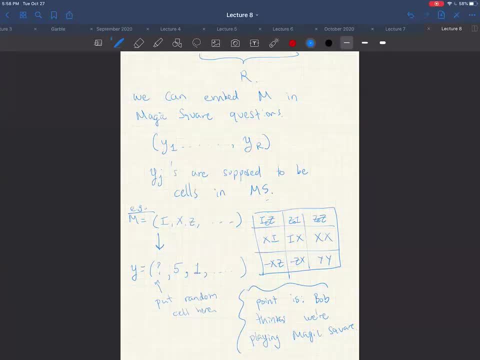 Yeah, OK, that's a super good question. You're right, Actually, in the way I described it, just this naive mapping, You know, if you start seeing a bunch of fives and ones, you're like, hmm, I wonder what. 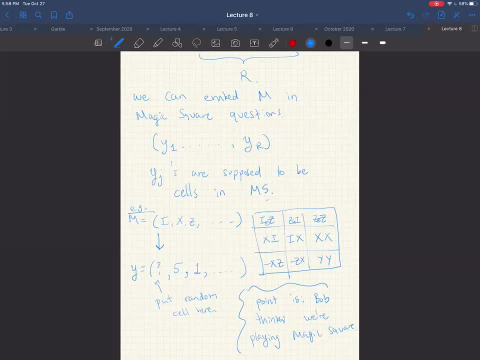 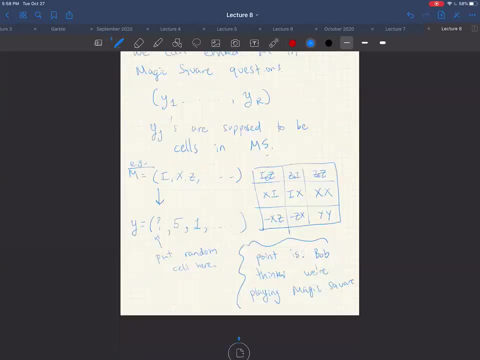 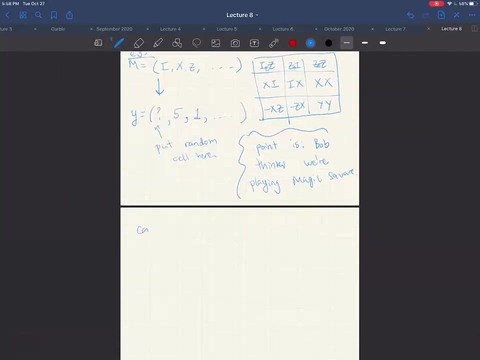 the verifier is asking me to do So. that definitely would be like a giveaway. So the way to solve that is actually you actually embed the M into like a larger Y. So imagine that Y like you're playing not just R games but, like you know, R squared different games. 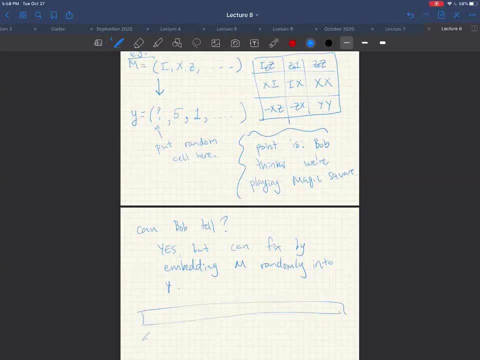 So your Y vector is going to be super long, Yeah, But then you just randomly drop in M at different locations And then that will be enough to kind of mask whether you're playing magic square or asking them to do a specific measurement. Bob is all powerful, isn't he? 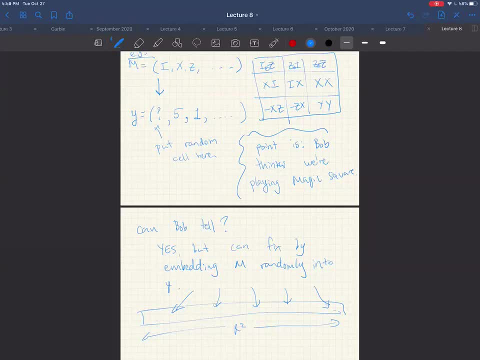 Like, if our question distribution is even in the slightest Far away from the uniform one, he'll be able to tell. He'll be able to identify this, And what you're describing here is not exactly the uniform distribution. Good, Good point. 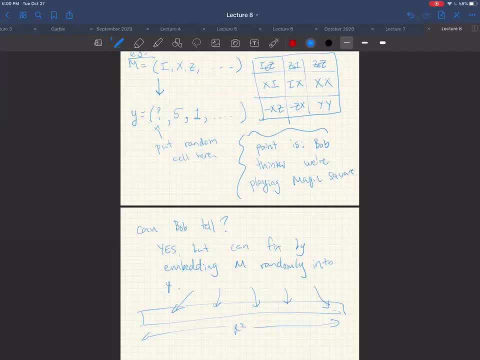 So it definitely won't be 100%. I see The uniform distribution, The statistical like the statistical variation will be actually very small And just based on that Bob will not be able to be 100% sure whether he's, you know, playing magic square or something else. 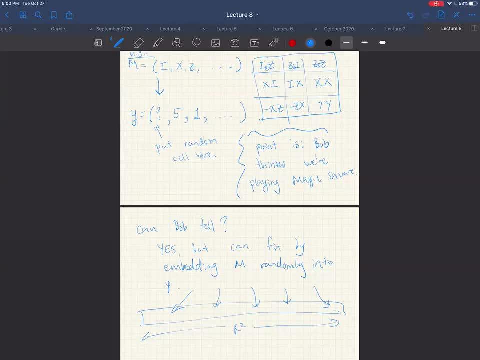 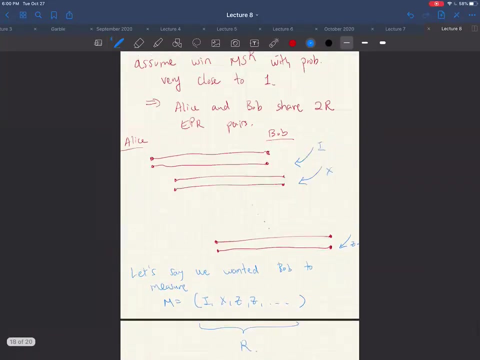 And so it cannot affect his strategy too much. Okay, Yeah, Okay, That's a really good observation. Okay, So we're out of time. I think we'll pick this up next time. But just to look ahead, you know, now you can see like we've used this rigidity to force Bob to be a trusted measuring device. 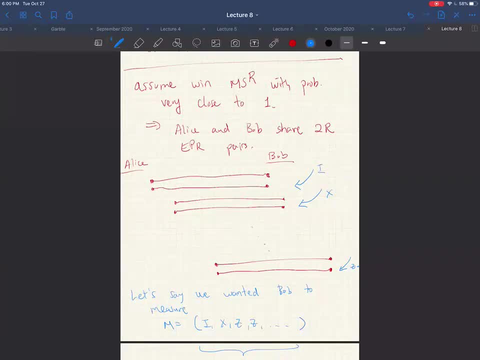 But we're missing a big part of the verification, which is like: well, he's measuring, it looks like he's measuring EPR pairs, But we actually want him to measure like a supposed ground state of this Hamiltonian.